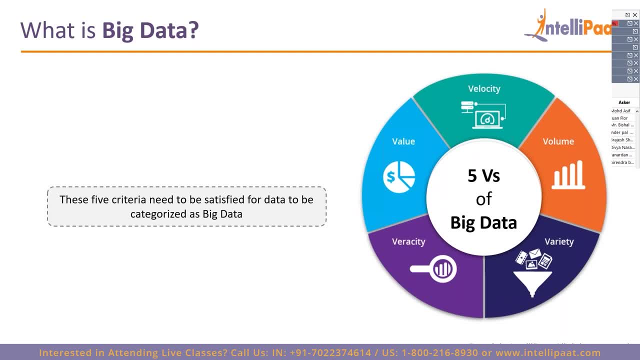 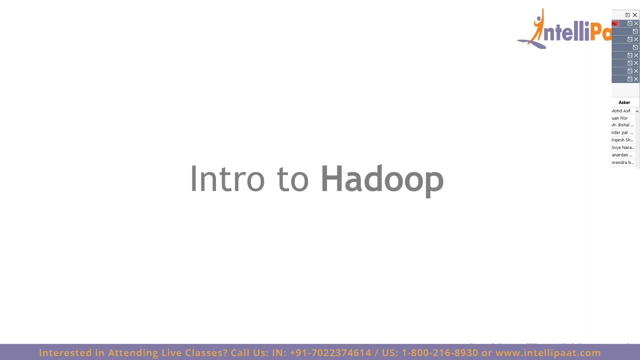 So these are basically the five B's that you need to satisfy in order for data to be called as big data. So, moving on the intro to Hadoop. So, naturally, a large amount of data and a large amount of real time data analytics processing requires tools that would help you do that. 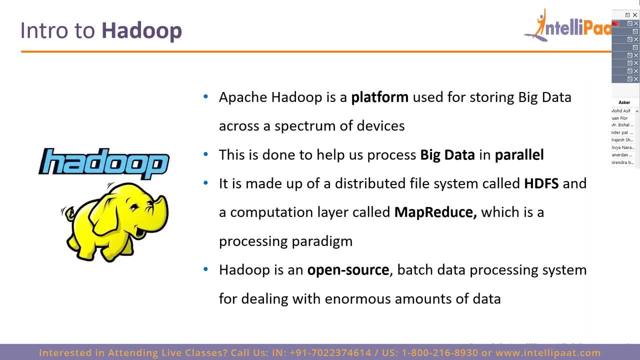 So that is where Hadoop comes in. So a brief introduction to Hadoop: It is a platform for storing big data and it is a platform for processing big data. So how does a platform- a software only platform- help us achieve a faster data processing and 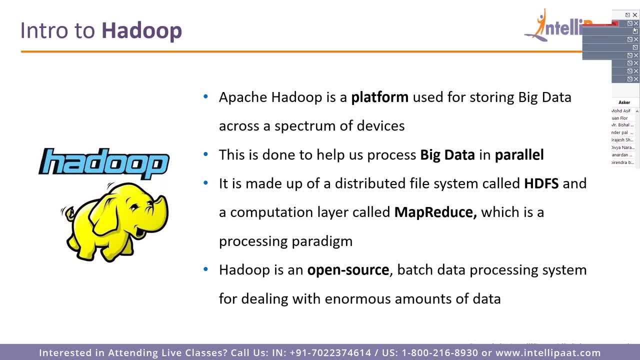 more efficient data processing whenever big data is concerned, right, So we're going to be going into that. So, firstly, that you guys need to understand is: in order, in order to process data faster, you need to process data in parallel, right? 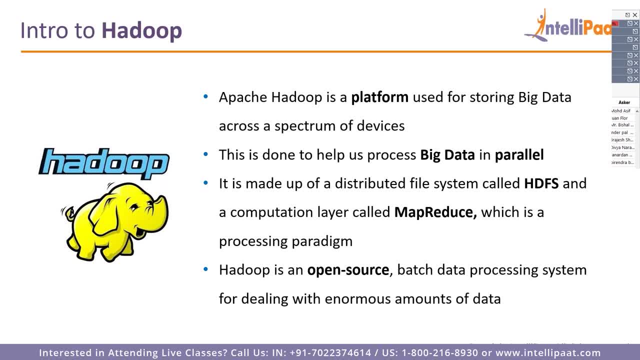 So if you are doing something on one system, and one system only, All of the processing work will be done in a sequence, right, But say: if you want to divide the workload by half on one system and do the work faster, you will assign, you will use two systems, You will divide the workload, give half of 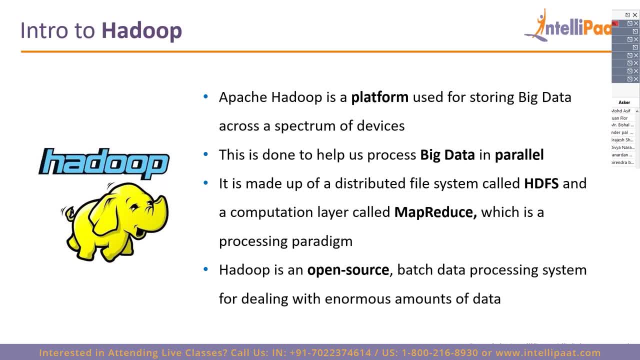 the work to one system and half of the work to the other system. Both of those will work independently, run independently and produce the output. Then you can merge that output and you can get your final answer for their particular problem statement. The processing is done in half the time and it's basically more efficient. 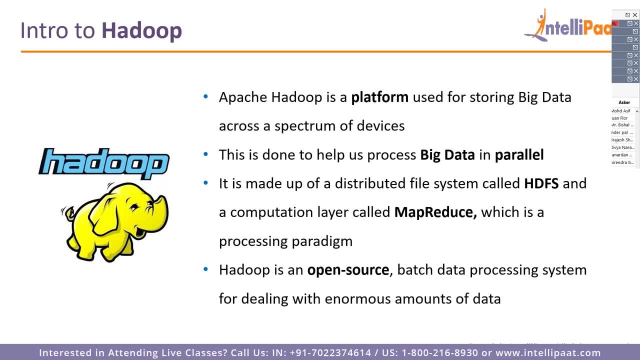 way to go about. So that is what Hadoop MapReduce is. MapReduce does exactly that. We'll be discussing how the Elastic MapReduce works in the cloud computing space, But right now, what do you need to understand is: imagine there are multiple computers. They're all connected together. 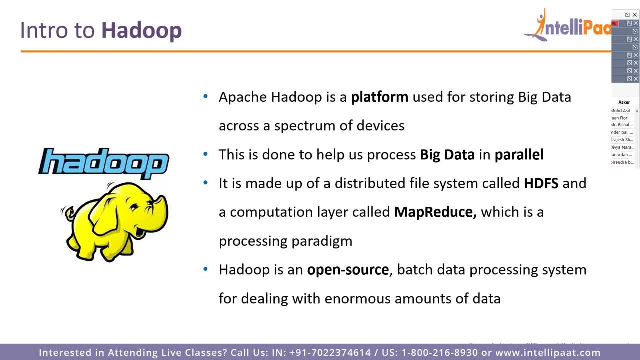 All of them have Hadoop installed on them, right? And you're basically giving data into that, into that cluster of systems. You're basically giving data into that and processing data on each of them. And you're basically giving data into that cluster of systems. You're basically giving data into that and processing data on each. 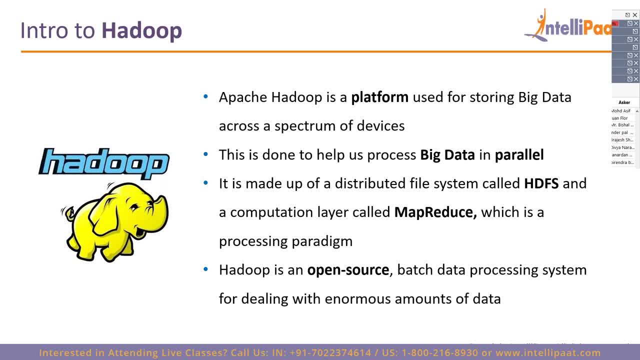 of those systems and back, And that way the work is effectively, the time taken by the work to be done is effectively reduced by a very, very large margin, And that is the only practical way to process big data, And it is an open source technology. So if you 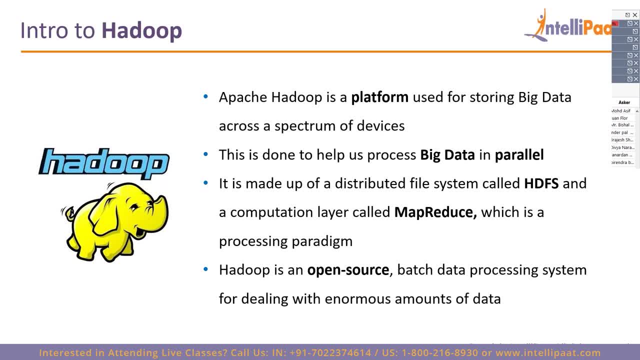 want to look further into how Hadoop works and look into the source code of Hadoop. make some modifications according to your needs. When you get into a professional space, it's obviously open source. You can do that as well. So this is the architecture. 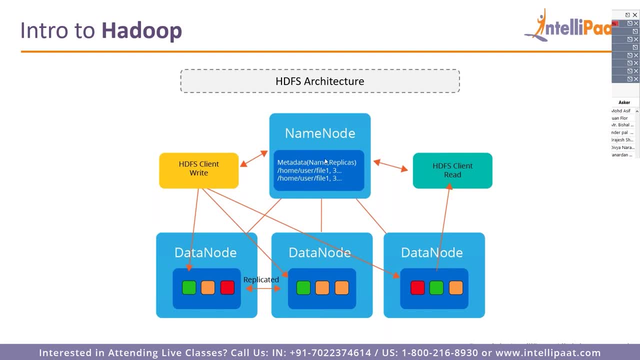 So if you guys can see my mouse, So imagine all of these four blue squares, that you have these four blue squares as computers or servers. you can call them servers, computers, basically a replacement for commodity hardware. So all of these systems are not very expensive. They're very cheap systems for everyday use. 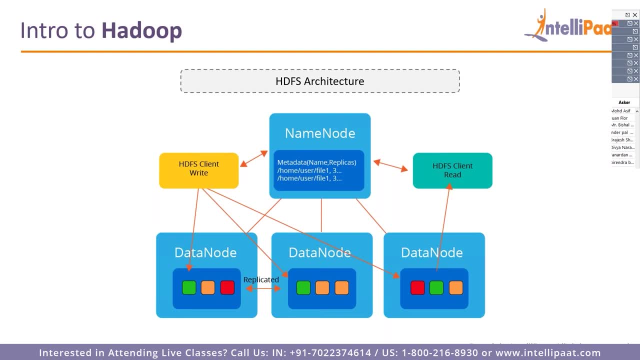 that you would use in your office or in a normal working background, with a decent enough RAM that is not too high. It could be four gigabytes. four gigabytes is the norm for laptops today. So these are systems, very average systems, but not too bad or not really great. 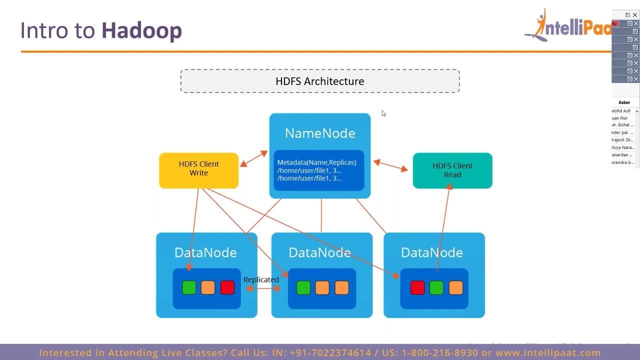 So these are synonymous with commodity hardware. So you have four systems. This is your big data cluster. You attach all of these four systems together, So what happens is you will eventually choose the system that is the least powerful to be the name node system. 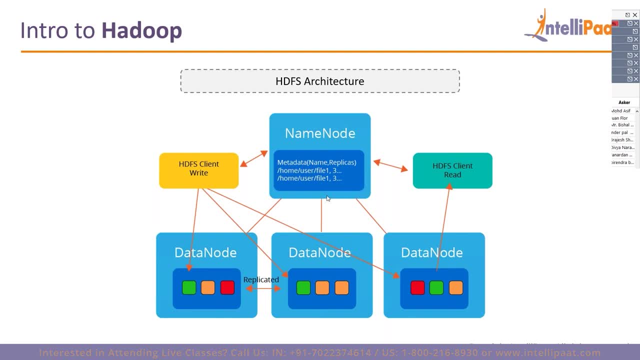 So the name node system only stores the metadata. So let me explain to you what the metadata is. So when you upload a big data file to a Hadoop cluster or a big data cluster, what happens is the file will be divided or, depending on its size and the block size of the HDFS. 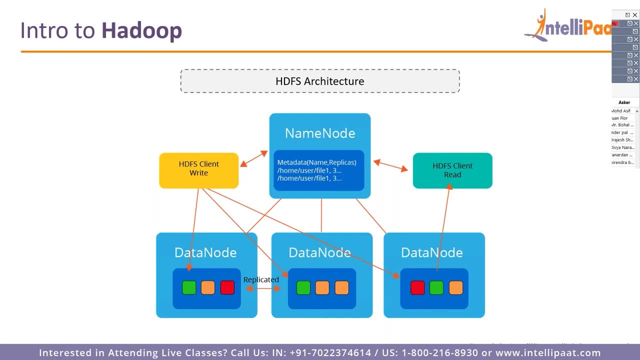 So the default block size is about 128 MB, So it would be divided into the multiples of 128 MB files and the first file. say, if you had a 256 MB file, Which is a 128 MB times twice, right? 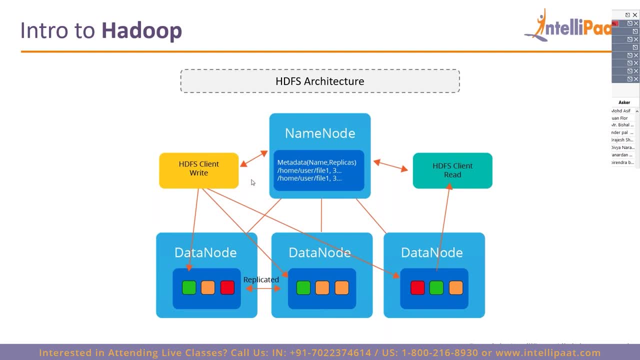 So you upload it, the client uploads it to the cluster, the client upload it to the cluster And then what happens is it will be the first block of that 128 MB would be on data node one and automatically the second block would be on data node two. right, 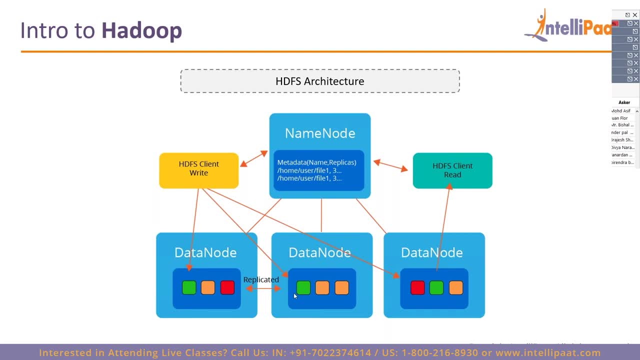 So this will happen automatically within HDFS, which is the Hadoop distributed file system. So Hadoop does that for you automatically. And what Hadoop does Additionally in order for you to get some sort of data security, say if one data node 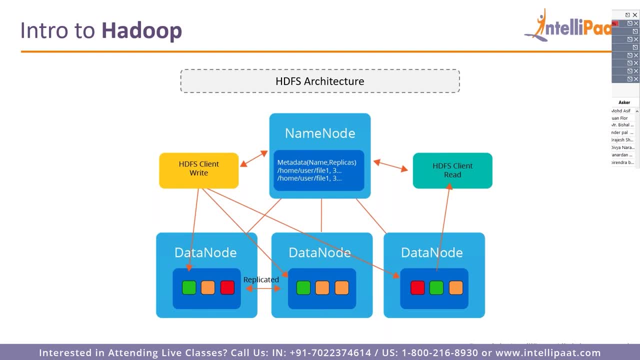 fails. you don't want your data to be lost, right? So for that, what you will do- you'll basically, what the data node will do is it will replicate all of those blocks on each of the data nodes. So in our in say, data node one fails, it's still on data node two and data node three. 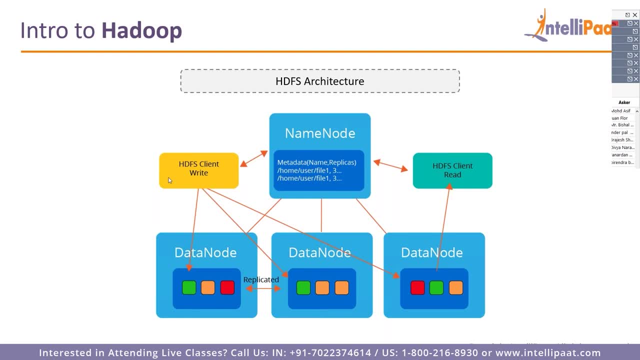 that particular block of file And the client doesn't even have to notice all of this. The client only needs to deal with the name node. So he's on the client. There's a remote remotely connected to the master node, So the client only needs to deal with the name node. 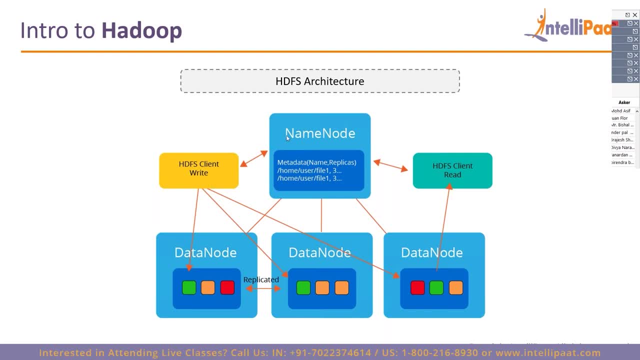 So he's on the client. There's a remote, remotely connected to the master node, Which is the name node. He uploads a file to the name node- He doesn't care about what's happening with the data nodes- And say if the data node one fails, the client will still be able to access this file without. 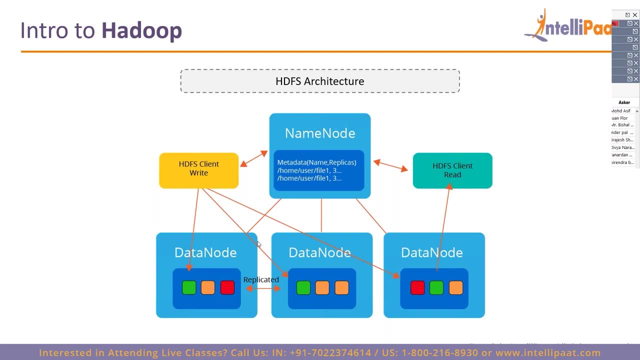 even knowing that the data node one fails. So this is the kind of abstraction that the ATFS gives to the client right. So this is the read and write procedure. The client can read, read this way and write this way without actually having to deal with. 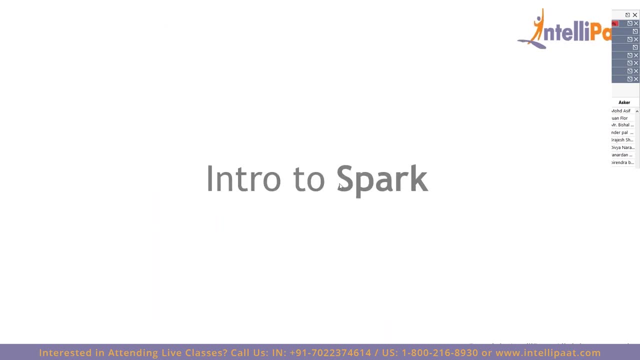 what the data nodes are doing. This is what the ATFS does for you, The introduction to Spark. So now that you know Hadoop, A little bit about Hodoop. basically the HDFS and how, what MapReduce is. So the thing about MapReduce is it has gone deprecated in a way, right. 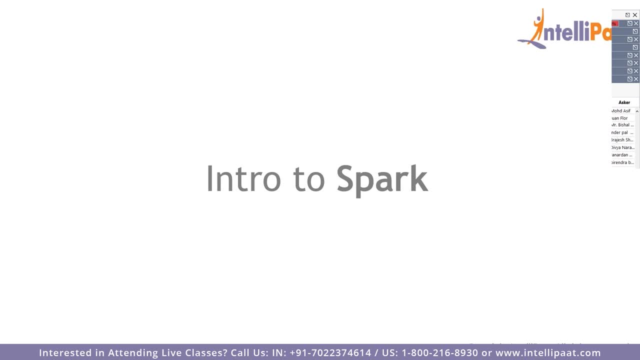 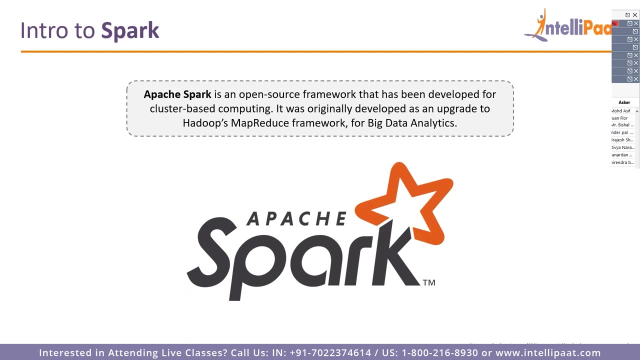 Because MapReduce is a much slower way of processing things, and I'll discuss why. So there comes Apache Spark. The advantage about Apache Spark is that it uses the HDFS, which is the Hadoop distributed file system, as its storage space. It can use it and it's the most efficient way to use Apache Spark. 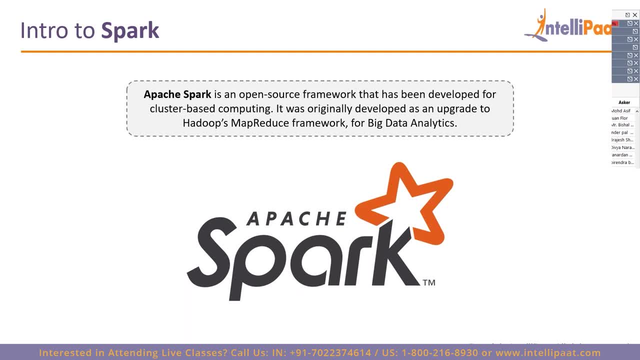 It can also use local storage as well. Apache Spark is not limited to HDFS, but the best way to go about Apache Spark is using the HDFS for your big data storage space, and it has an open source framework, so you can edit the code as much as you want and do it according to your specifications, and it is 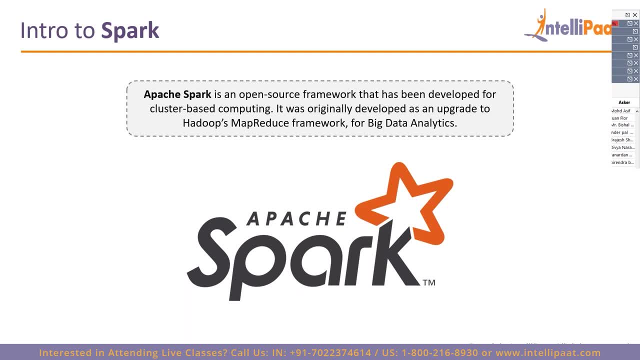 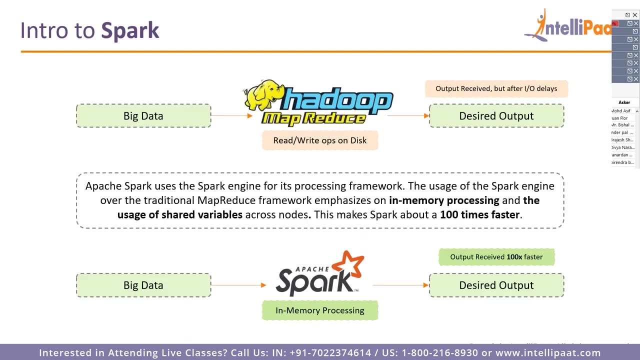 an upgrade to Hadoop MapReduce framework for big data analytics. So Apache Spark has been optimized for a cluster, so a lot of computers or servers attached together, Like I was discussing earlier, which is a cluster based computing. It's optimized for that, so it does all of that for you. 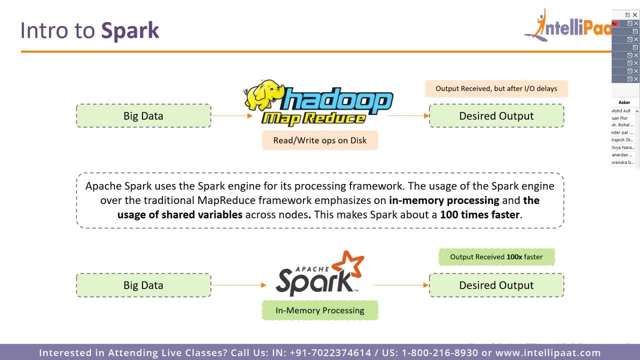 So let us discuss why we don't use Hadoop MapReduce anymore and we use Apache Spark for the programming part of things, not the storage part of things. Say, on the upper hand side you can see big data, MapReduce and the desired output. 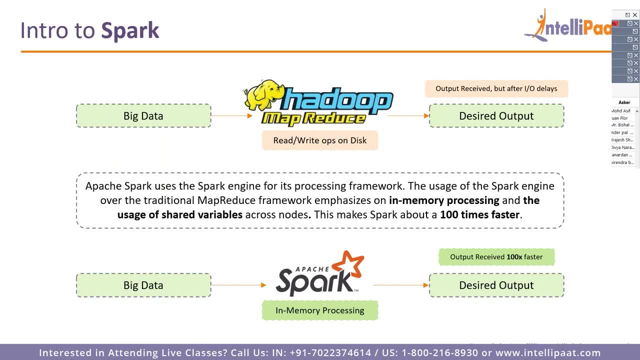 So what MapReduce does is say you're processing data. all of the intermediate jobs, all of the intermediate files that are generated in your MapReduce Procedure- right, They are not stored in the RAM, they're stored on the disk space. right, only while it is. 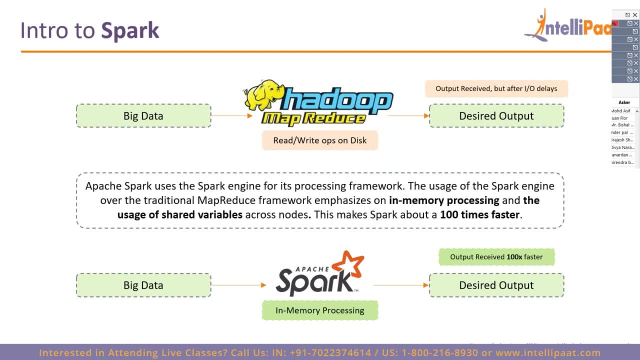 being processed, They are stored in the stored in the RAM, and when they are not being processed, they're stored in the disk space. So if you understand how computers work, you need to first transfer the data from your hard drive or your disk space to your RAM and then the CPU processes that data in the 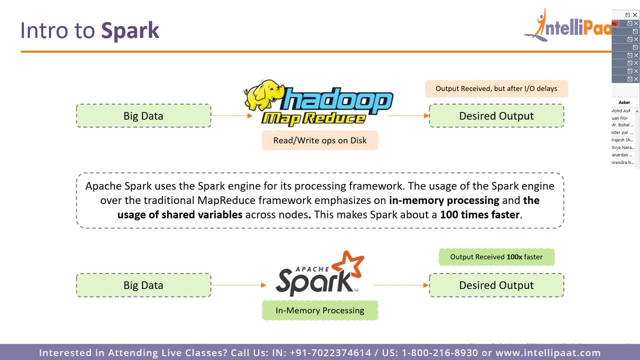 RAM. The CPU gives the output to the RAM, Okay, And the output is then transferred into your disk, right? This is the standard procedure of how processing works in general. This is how read and write operations work, right. So this is what MapReduce does. 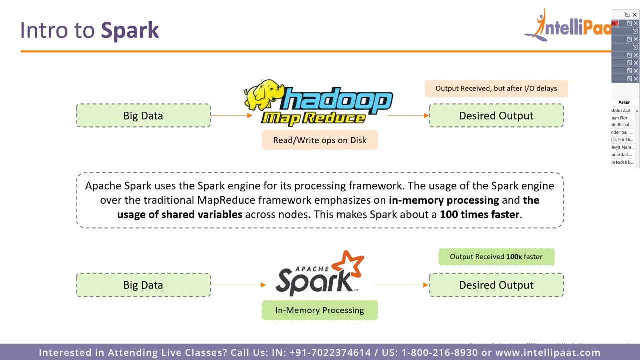 It takes that data in the RAM, it processes, it puts the data, puts the output back in the RAM and then it basically puts it back into the disk. right, So you get your desired output. But this cause this causes input output delays and it is a slower method than what can be. 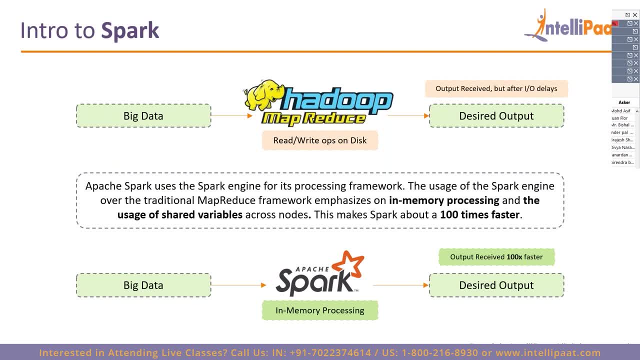 achieved today. So from that time a large amount of RAM has gotten cheaper. RAM costs have gone drastically down. They are not as expensive as they used to be. So getting excessive amounts of RAM for big data purposes- at least not for everyday user. 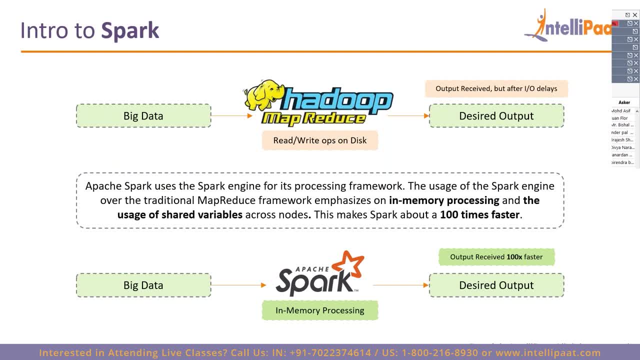 purposes, for big data purposes, it's cheaper, right? So then comes in Apache Spark. So Apache Spark, instead of reading, writing every time it does in memory processing, right? So what that means is that, say, you have multiple data nodes and multiple data nodes each. 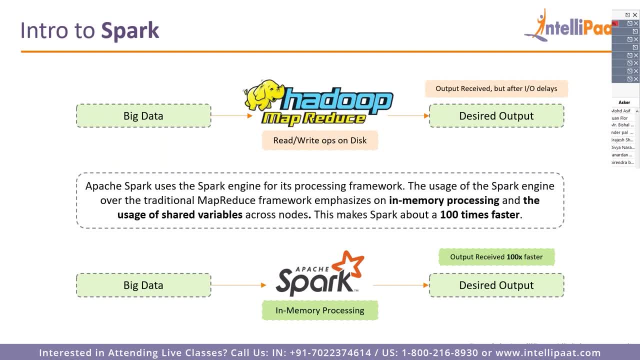 of these systems, each of these components on the multiple data nodes. they all have RAM right And they have increased amount of RAMs than before. So Apache Spark will take the block of data access to that data almost instantly. It does not have any input output delay from the disk to the RAM. 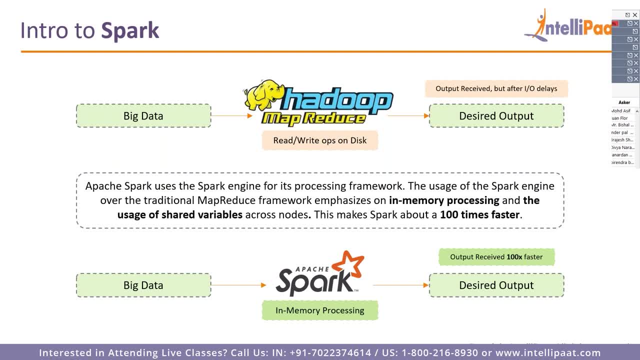 It gets that data almost instantly right. So this is why Apache Spark as a framework is better, And I about it. It's about a hundred times faster than MapReduce, So because of that in-memory processing procedure that it follows, it's about a hundred times. 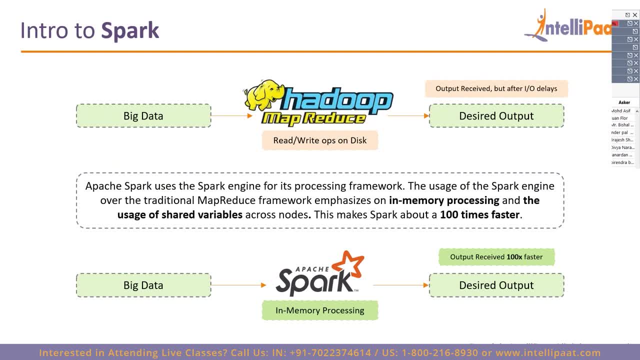 faster, right. So this does not mean that you will take two megabytes of file and put it into it and you'll notice the difference. This happens when you're trying to process terabytes to petabytes of data that you'll notice the actual difference about within the speeds of Apache, Spark and Hadoop MapReduce. 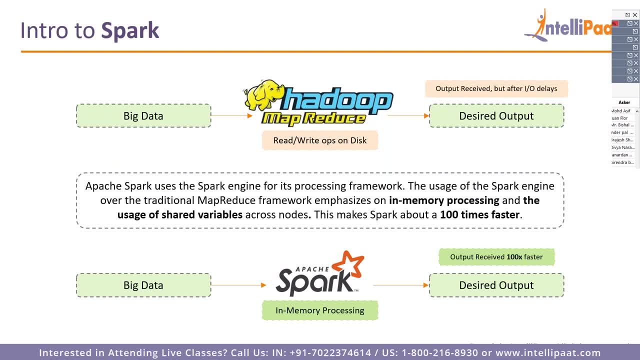 That is where you'll notice the difference, because a little bit of delay adds up and that gives you A very delayed output when you're using MapReduce file. That does not happen when you're doing Apache Spark. So let me get to the next part, which is Elastic MapReduce on the AWS. 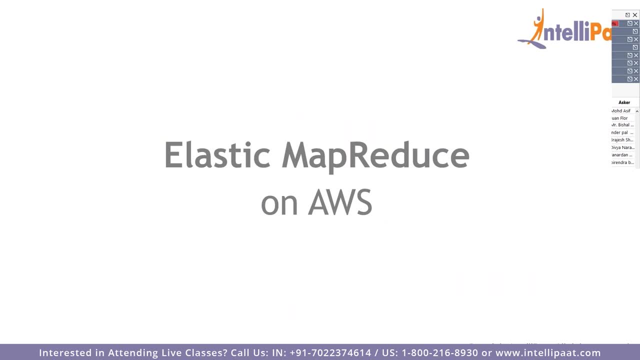 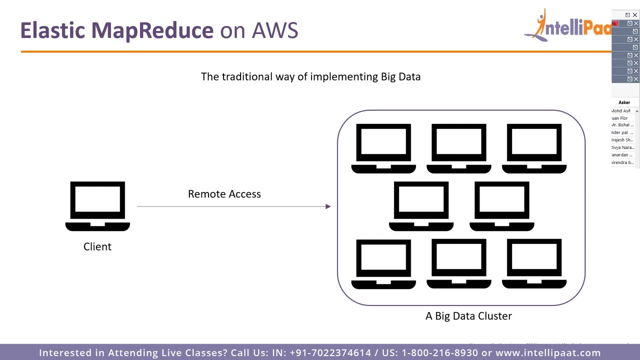 So you know how MapReduce works. you know how Spark works. We're now on to the part where we discuss Elastic MapReduce. right, So it's nothing. Elastic MapReduce basically means that the original way, the traditional way of implementing big data is: you're sitting in your very cheap laptop somewhere. 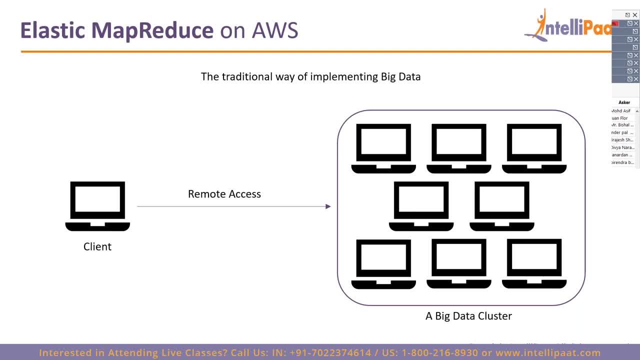 You're an assistant, right, And you're a client. You remotely access a big data cluster which is basically a combination of a lot of computers And that is a big data cluster. essentially, This is what you do normally if your big data cluster is housed somewhere locally within. 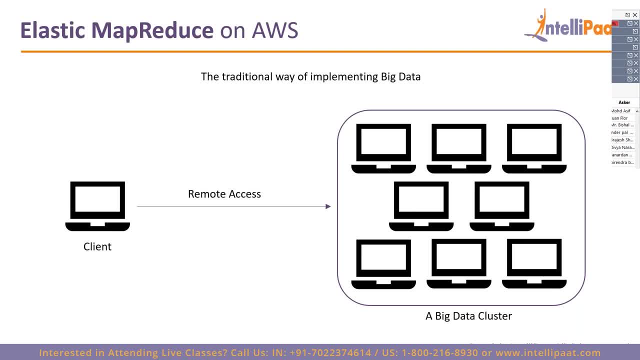 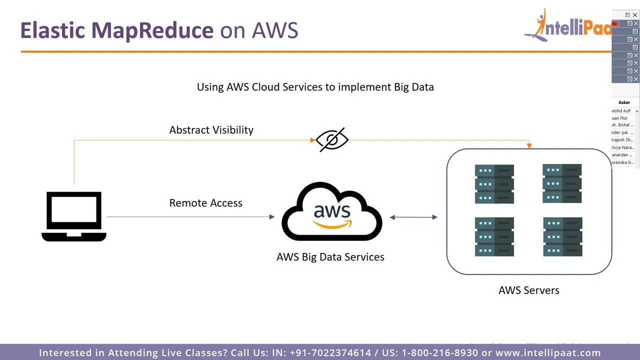 your organization or being rented- right, So this is what it does. So Amazon thought about this. Amazon thought that we could make this business profitable, right? So we use our EC2 instances and create a big data cluster out of that and offer that as. 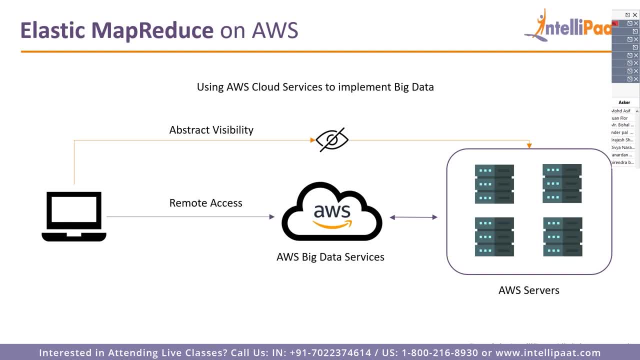 a service to our clients, right? So instead of the client and the organization where the client works having to set up a Hadoop cluster, add all of these servers to that Hadoop cluster, all of these hardware, the commodity hardware and everything, instead of the organization having to do that and 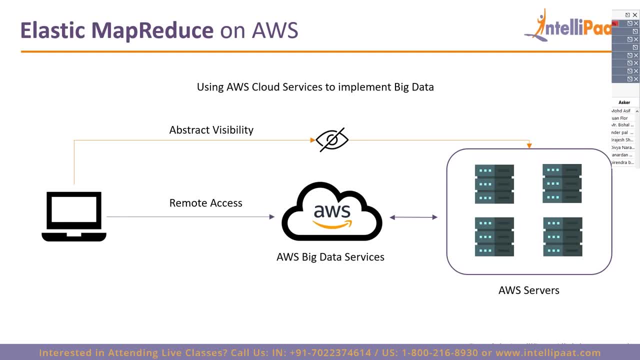 maintain it within Hadoop administrative and everything. Yeah, So what Amazon provides to you is basically a service where you use their Hadoop clusters, their cloud computing clusters, and you pay only for the amount of time that you're using those particular cluster of features. 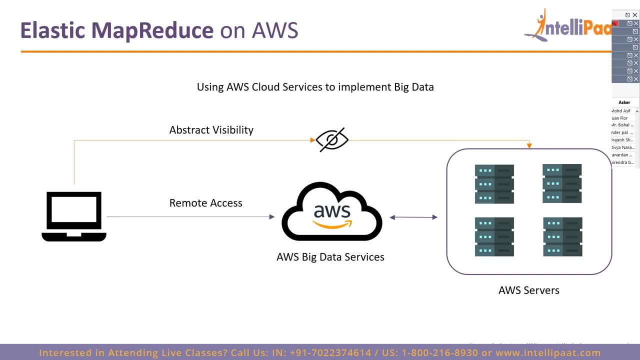 So not only does it reduce the time that it takes to set up a cluster and everything locally, it also reduces the cost. So if you're renting a server, if you bought a server, Yeah Yeah, You have to pay for maintenance. 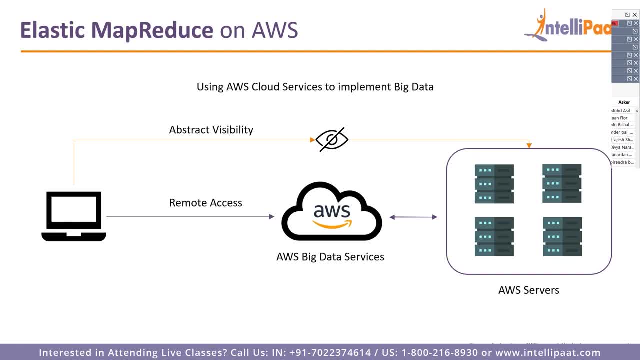 You have to pay for electricity because the server is always running right, So you have to do all of that. So when you actually subscribe to AWS and use their EMR, their Elastic Map Reduce, what happens is you only pay for whenever your job is running right. 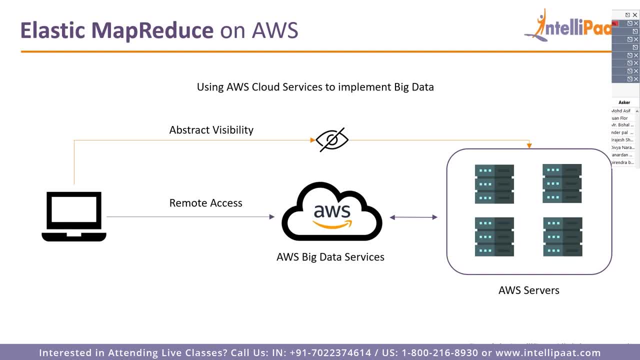 And you don't have to do maintenance. You can scale up as much as you want. So say, if you want to increase the amount of data nodes in your server, you can simply put that number into a section, into an option, basically. Yeah. 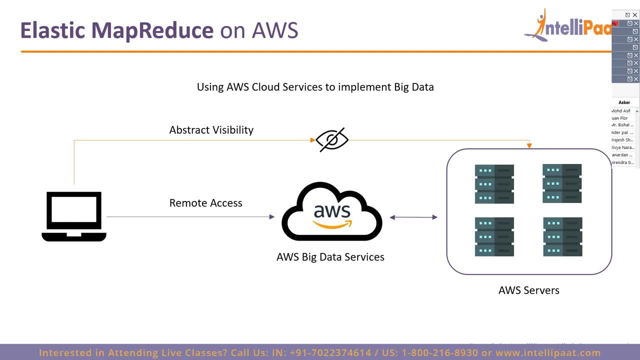 Yeah, Yeah, In a web browser and your server would be scaled up instantly, right? So these are the things that AWS has, a big data service provider, does for you, As you can see on the other hand side, you don't again. you don't need to care about. 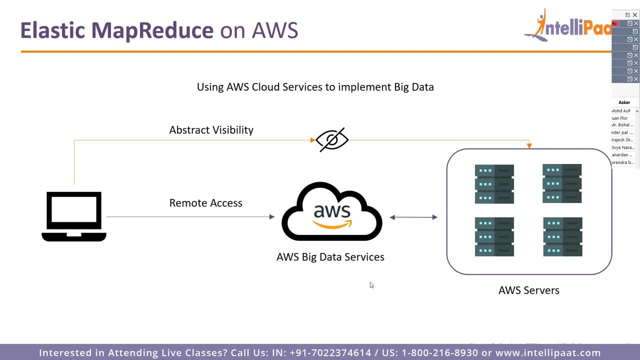 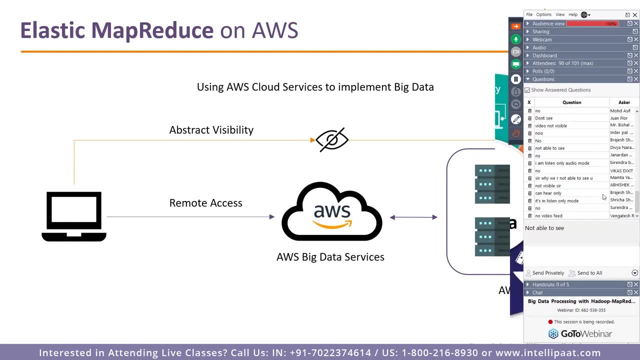 whatever is happening inside the server, The AWS- you're only dealing with the AWS website, right, The AWS login page in that sort. there's also customer support for that. so if you're facing any issues, you can simply contact an aws individual from customer support and he will absolve your doubts for you, if you. 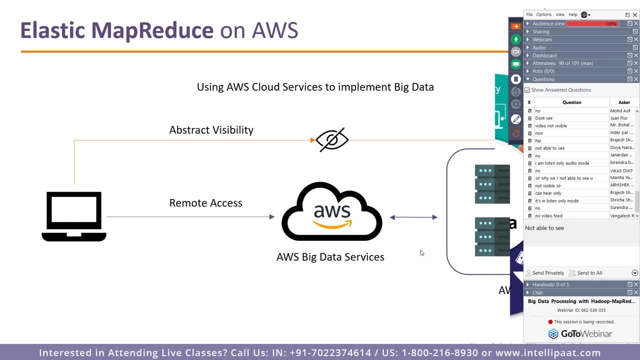 are facing an issue with it. so, instead of basically no maintenance, uh pay, pay as much as you. these are the two benefits uh, canon is asking: is spark also using hdfs? yes, spark is also using hdfs, uh, but it has the option to use other file systems as well, so any file system that there. 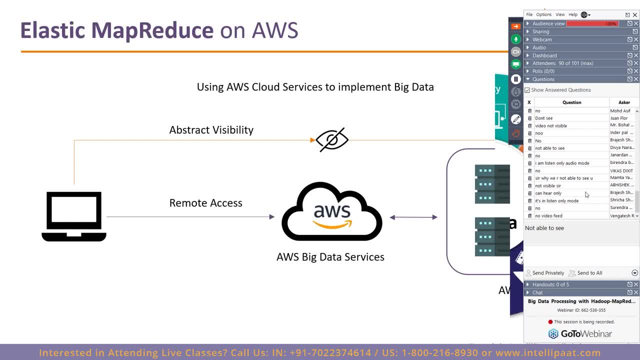 exists. spark can use that. it's not just limited to hdfs, uh. but if you're operating on a cloud computing, on a cluster computing structure, it's better to use hdfs as your storage format, because where else are you going to store big data? you're dealing with big data here. you're not dealing with. 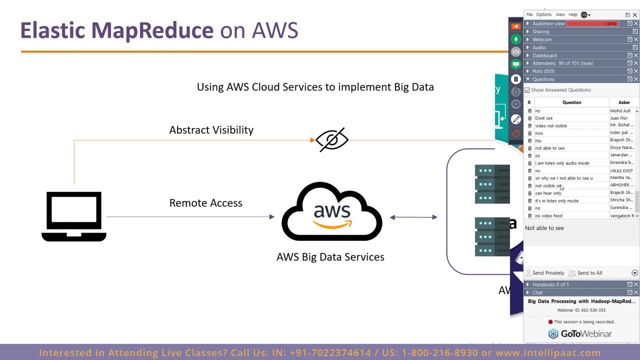 normal data, so local file system doesn't actually work. uh, we know, this is asking: is spark costlier than hadoop map reduce? no, uh, spark is just software framework. it's uh, it's cheaper actually. i mean, i don't mean cheaper, i mean it's free. it's free to download. that's these, these particular software frameworks. 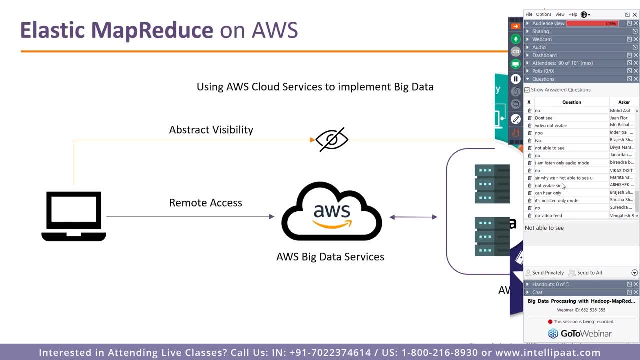 like hadoop and spark. they don't cost anything. uh, the only thing that will cost you is renting a server, uh actually buying hardware for that or uh subscribing to the aws services. so anything that you're buying, or hardware oriented that you're buying, or if you're subscribing to a cloud. 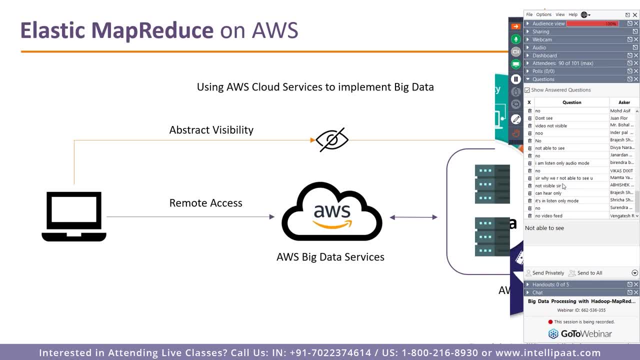 computing service that will cost you nothing else. uh, if you mean costly in the way that it uses more ram, yes, definitely that way it's more costly, but not from a price point. uh, the howard is asking: what exactly do you mean by? uh? you, it's, it's a, an it's. so, basically now, 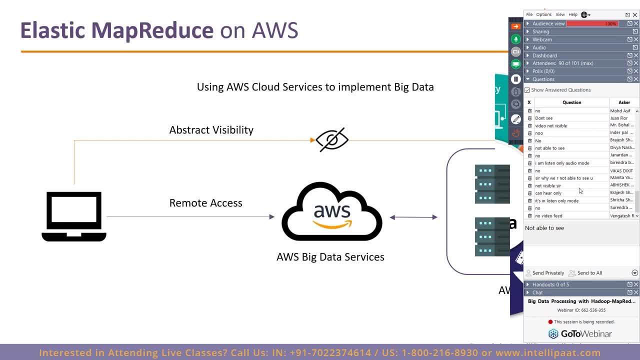 that's if we have to pay for uh, only for the services that we use. say, you've started your emr cluster, right? uh, other than the ebs volume, which is the hard drive space on those particular instances in your emr cluster, it would mean that you're actually spending a lot of money and that might be ön. 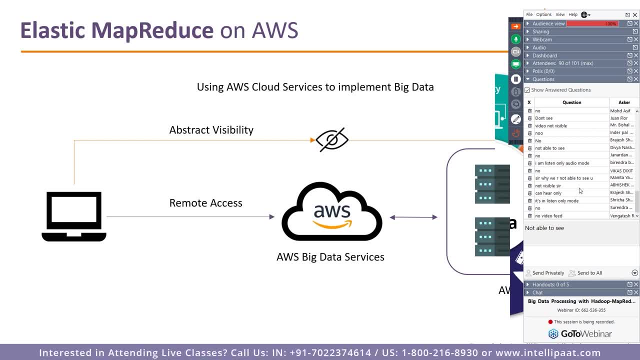 emr cluster that you've started, other than the hard drive space. that is a very nominal amount that doesn't even make a dent in the wallet, nothing big. it's just basically a nominal amount that you have to pay depending on the hard drive space that is there in your server. 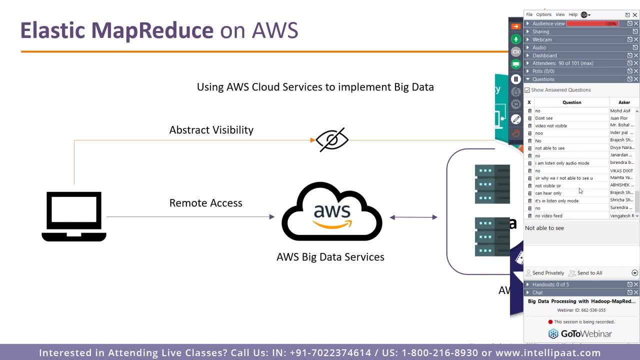 so other than that it, as long as your emr cluster stays dormant- right as long as your emr cluster stays dormant- it does not do anything. you will not be cost a penny for that right. so that is how it works. it only pays when you're running a job on it. other than that, it does not do anything. it does. 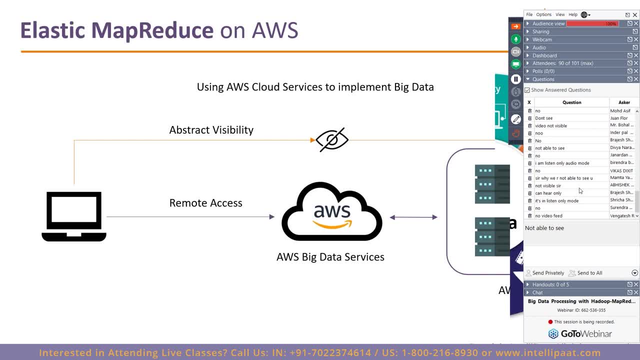 not take any money from you. a lot of people asking about aws. what aws is? aws is basically a cloud computing platform. so you might have heard about microsoft, assure, google cloud. so aws is a competitor to both of those particular services. so if you don't want to buy expensive hardware, 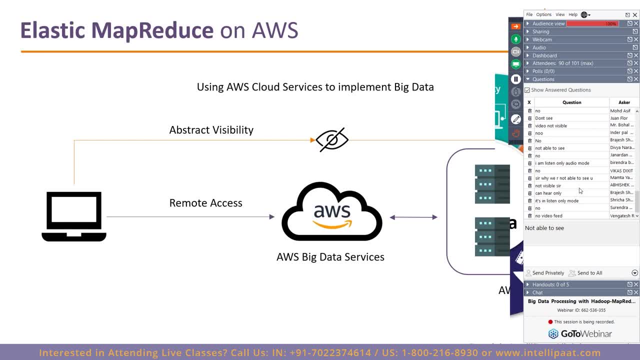 if you don't want to buy a server. if you're working for a company, if you own a company, you don't want to buy a server. you can basically do implement all of your server's needs using a cloud computing service. cloud computing service is basically a big corporation owning the servers for giving to. 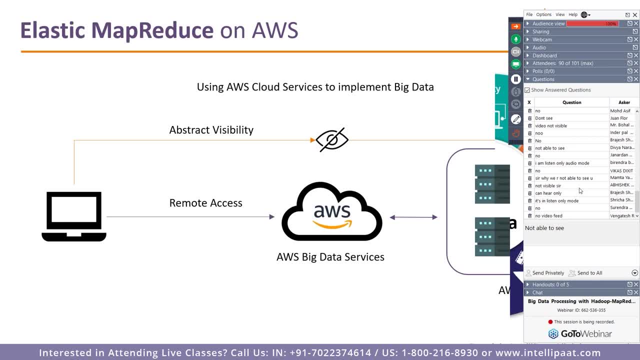 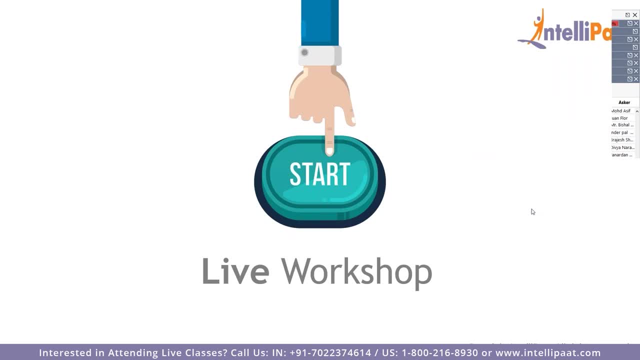 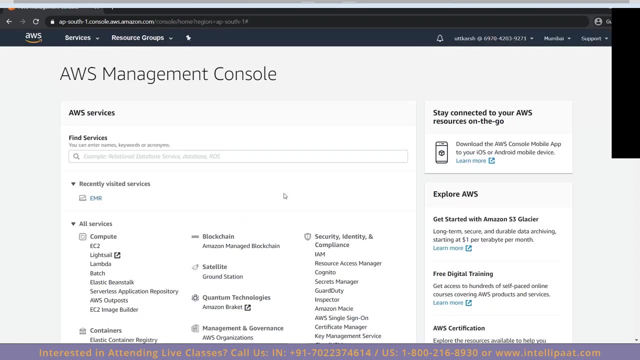 giving to you the servers on a rent basis. so that is what a cloud computing service. you can access the cloud computing services via the internet. so the live workshop, what you guys have been waiting for. so already logged into my particular aws account, so here's my aws account. so this is what the aws 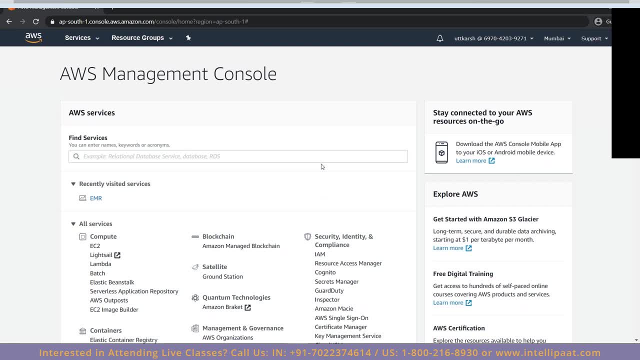 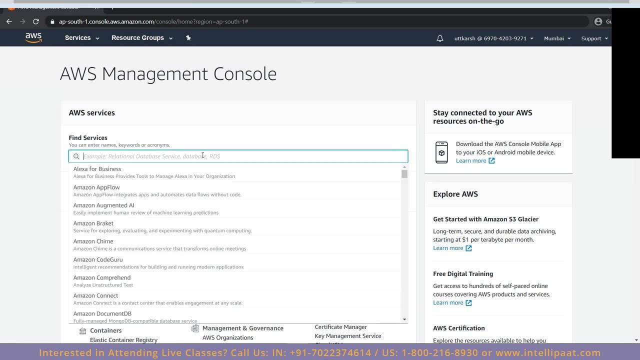 management console looks like right, you create an aws account. uh, you will be created this with this page once you log in, right? so i'll be showing you from the start how it works. so aws has a lot of services. there are services for virtually everything. aws does it for you, whether it's 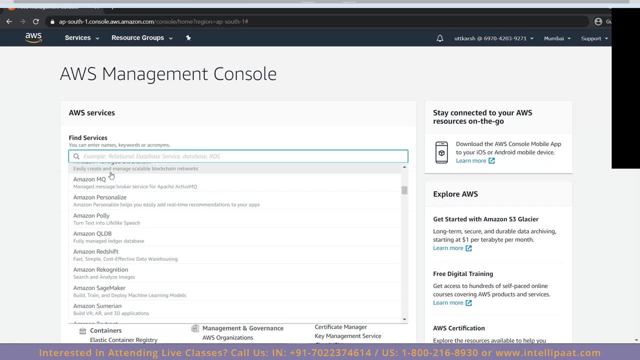 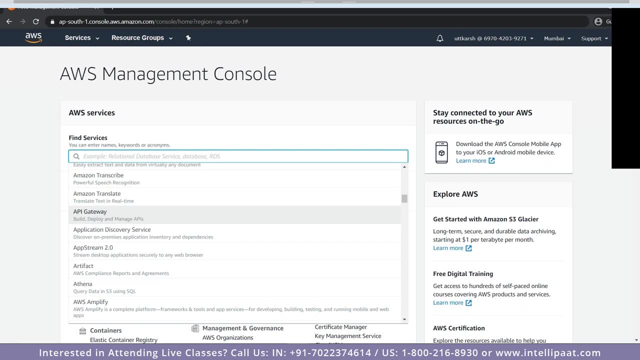 storage, whether it's processing, whether it's whether it's lambda functions, uh, uh data database management, data warehousing, uh. video data streaming and everything. you can basically do everything with aws. aws has service granted for you, right, so, as you can see, athena does query data, which is present in s3. s3 is basically a storage platform for aws. you can store some. 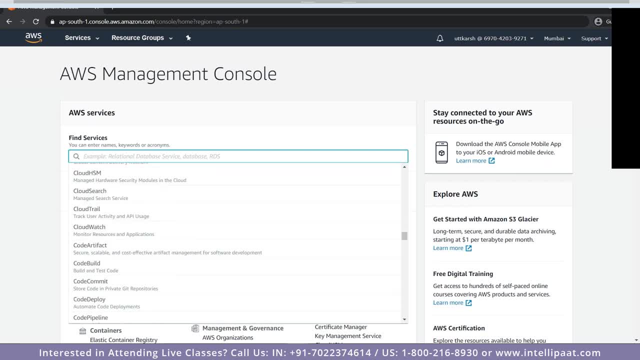 data in buckets necessary. so all of these things are there and at very reasonable costs, if i may. so if, depending on your organization size, you have to pay only according to the use case that you have, you don't have to pay a fixed amount every month, you can pay basically all of these services. 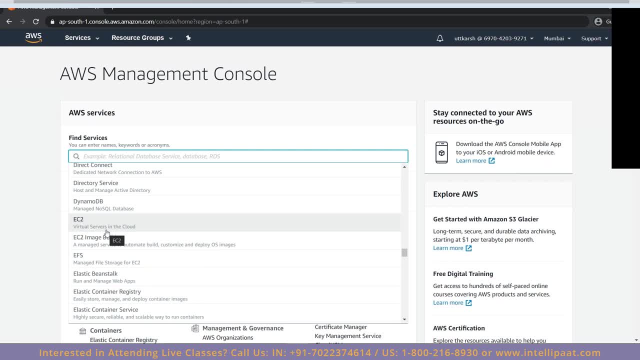 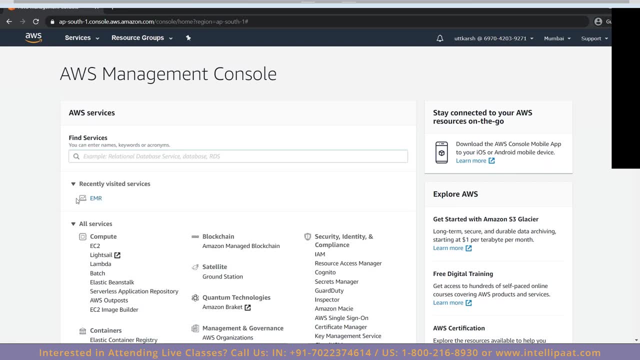 which virtually all of these services that there are there exists. you only have to pay for as much as you use, nothing else, right? so all of these are there. so the first thing that we want today is elastic map reduce, so we'll simply type in emr, which is the euphemism for that. 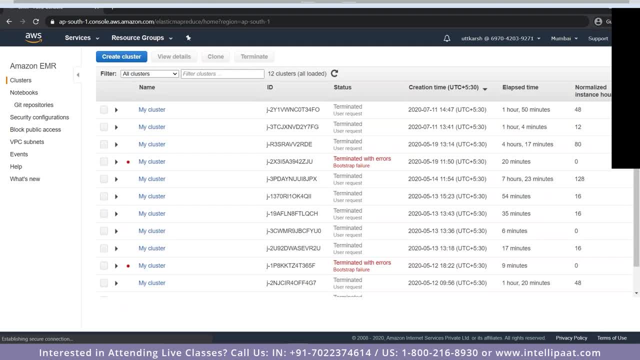 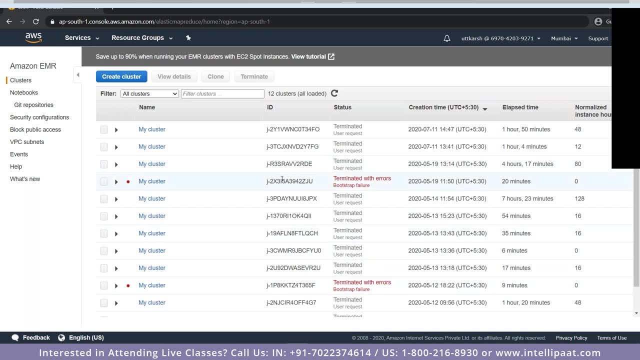 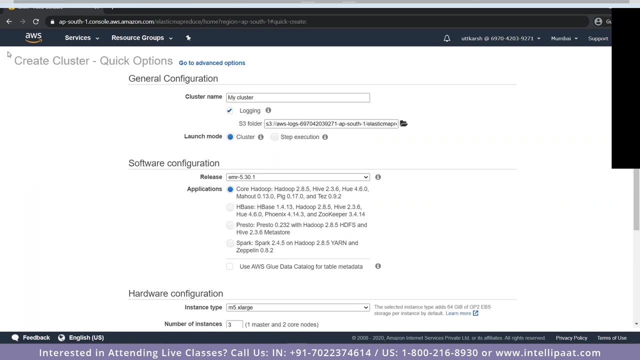 and open it up. so i've already uh created some clusters and terminated them. that does not uh really mix, uh really account for anything that we're doing today. so what we're going to do is create a new cluster. you simply click. as you can see, it's very simple. you have a simply click. 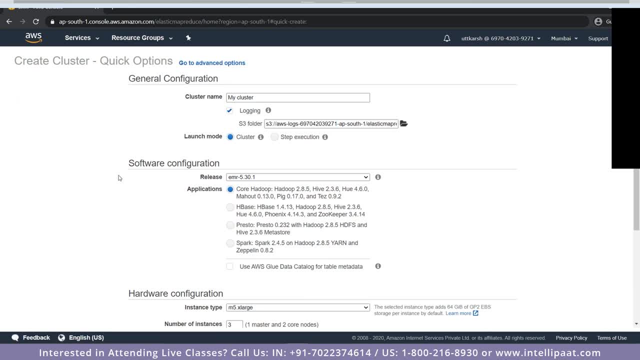 there's no coding involved in all of these server creations. so if you were setting this up locally in a particular localized space, uh, you basically have to install the appliances in every particular computer that you have. you're adding to the cluster. so all of this you don't have to do. the amazon web services will do. 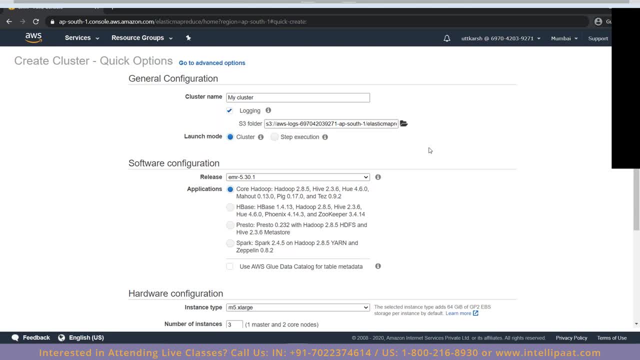 it for you. so the first thing that we would do is name our cluster something so we can name it workshop cluster. you can do that and, uh, you can enable logging- so always better to enable logging- and, uh, you can now decide what you want to install on your particular cluster. so the 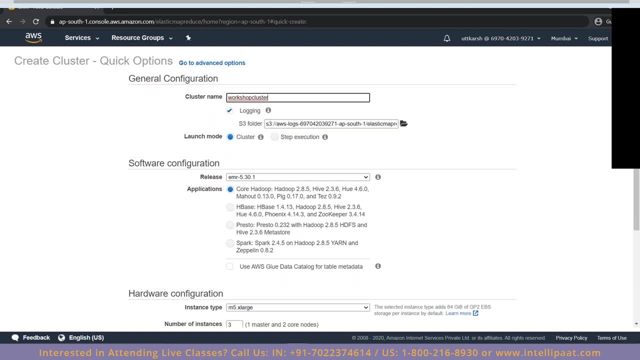 core loop is absolutely essential. so for you to, in order for the cluster to exist coherently, you need to install core for that. uh, then you can simply- i can simply- select the spark option. uh, because we're going to be using sparks, so this includes spark 2.4.5 with. 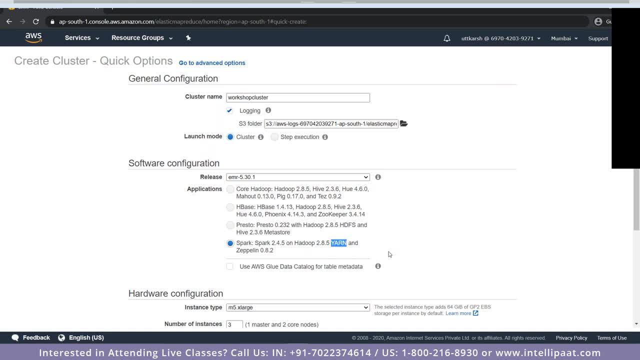 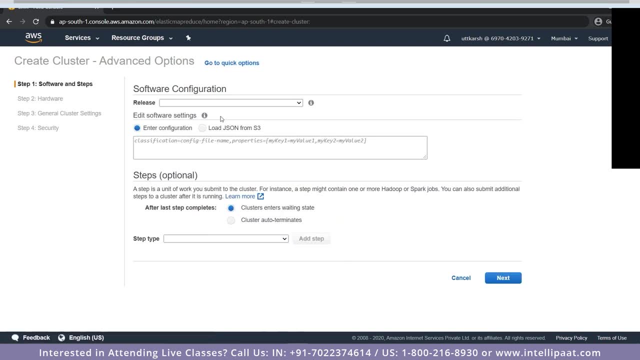 hadoop 2.8.5 and yarn, which is the resource manager. so this is the configuration that i want. if you want to do something a little more complex, you can also go for the advanced options, where you will be, uh, prompted to choose what particular frameworks you want to install. so the all of these. 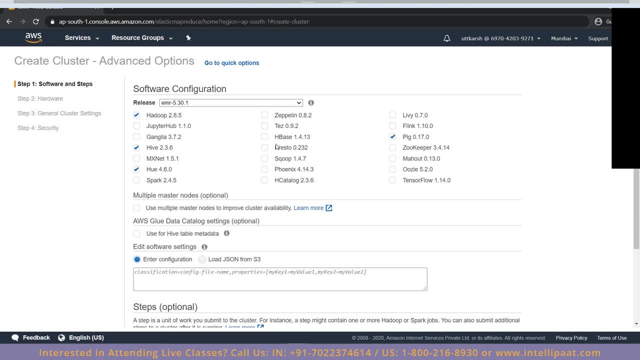 components: hadoop- is there mandatory? uh, these are. hbs is basically a data querying tool- uh sorry. and hive is a data warehousing tool. scoop is basically what connects your relational database management systems to your cluster and hdmi space and tensorflow. if you're doing, if you're opting for machine learning, and right now we're implementing spark, so go back to the. 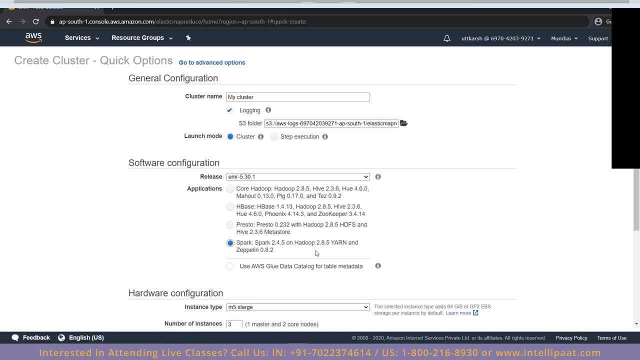 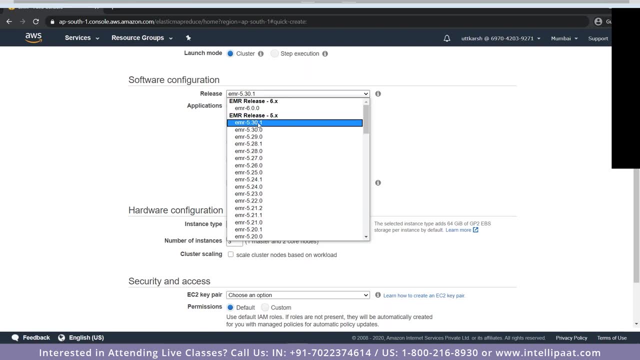 quick options and select the default option that they've provided for me, this particular thing. that means that the latest version of emr, this is the stable release, which is the 5.3, 30 and 0.1 stable release right now. select that and then we can, uh, actually choose. 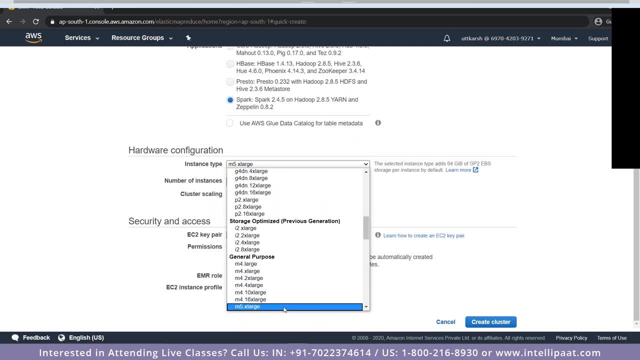 the hardware configuration that we want. so if i expand this, you'll see a lot of things. so all of these are nothing but machines, right? these are server configurations, right? so, uh, what? what we want is basically a general purpose server, right for our slave nodes and master nodes. we want a. 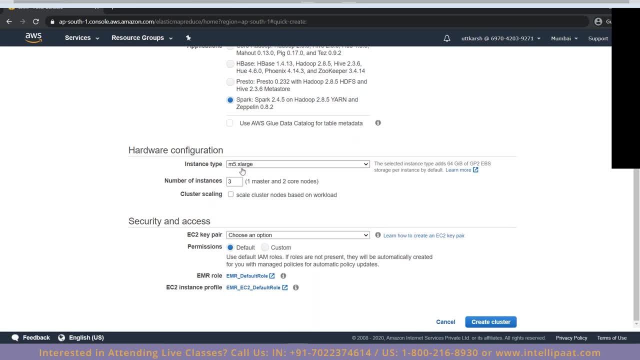 single purpose server, so we'll simply select what is there already, which is the m5.x large. so, and you don't have to worry about their sizes at the moment, because, as long as you're not using the cluster, it wouldn't cost you anything, right? so, uh, it's always a better practice to terminate. 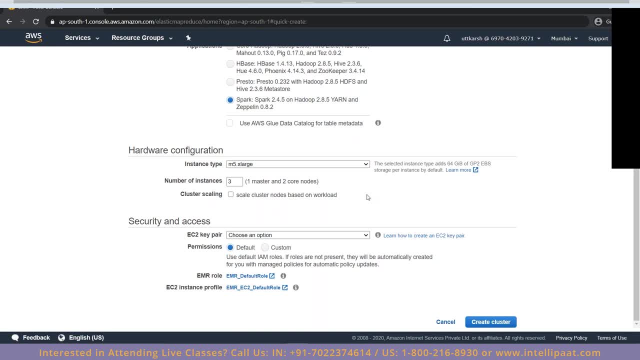 when you're not using. but uh, even if you don't terminate, uh, it only costs for the ebs volume that is attached to your particular system and it does not cost much if you just leave it dormant. but better option to terminate. and then number of instances i want is three. you can expand the server as well. so if i say four, 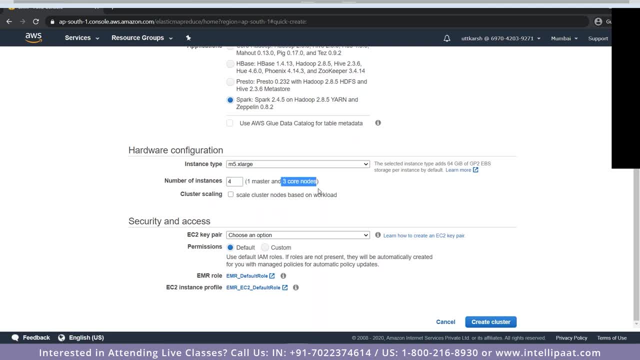 what will happen is there will be one master node and three core nodes, which is the data nodes. if i fired five, there will be one master node and four code. so it depends on your use case. right now i'm not going to be doing anything really big, so i only need uh three. but uh, depending on the 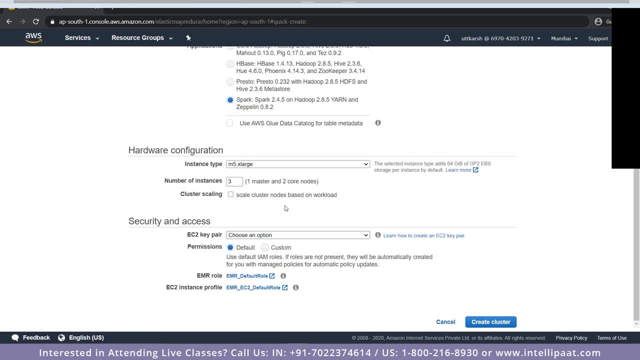 organization and the workload. they can scale this up as much the same point, right and uh. we're going to be using a ec2 key pair, so this is important. i'll tell you why. so, firstly, we'll create a ec2 key pair, we'll go to the uh. 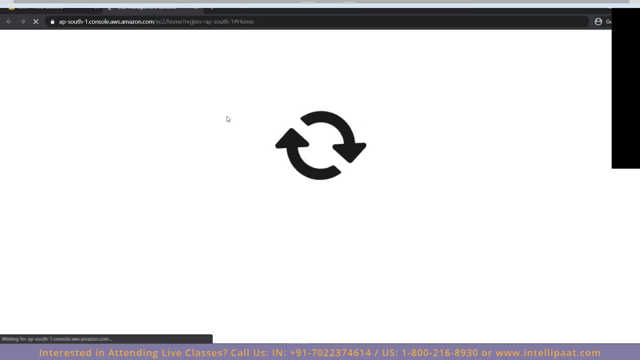 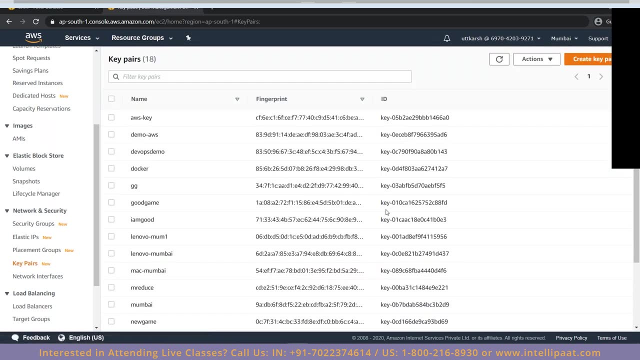 just a moment, go to the ec2 console and then we'll go to keys, key pairs. here, this is basically an uh. instead of using a password to actually access your particular master node, what you could do is simply create a key, a public and private key pair, and you can use. 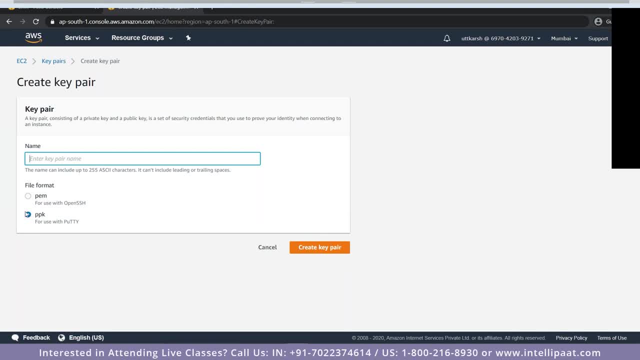 that in party to remotely access it. so always be sure to select ptk for that. this is the format that goes: the party. you can also use the pem if you're using open ssh, but i prefer to use party instead of that. so, uh, you can name this anything you want, so i'll call this workshop key. 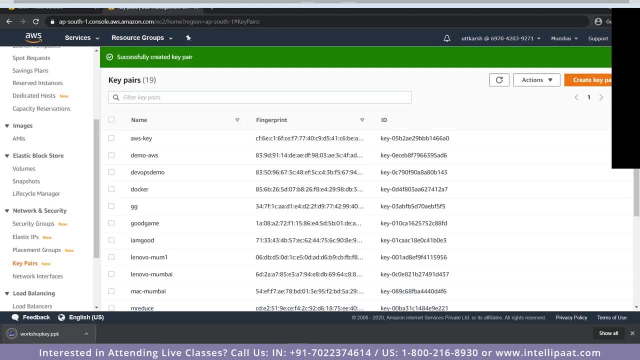 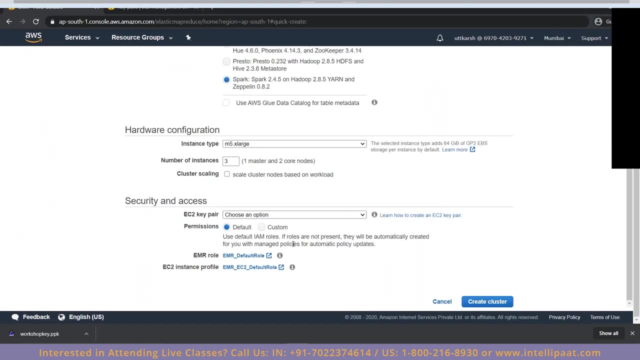 and i'll create a key pair and it automatically gets downloaded uh in my system. so now we can use that uh with using uh while we're using partners. first, let we need to launch it right. we need to launch the cluster that we have. so the first thing that we 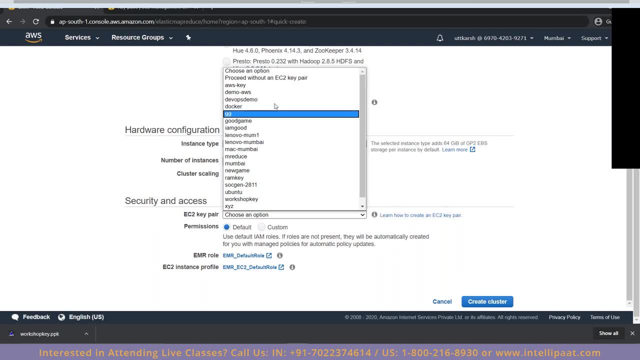 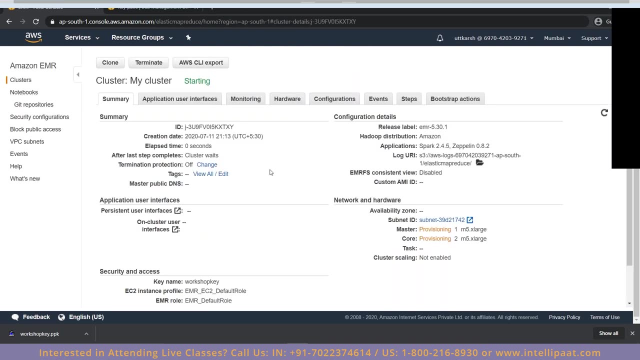 would do is select the key pair that we just create. so let me see the name: workshop key. it automatically comes in. you don't even have to refresh the page. it will automatically come in. so you select that and then we'll click on create cluster. so it takes some time to start. so the 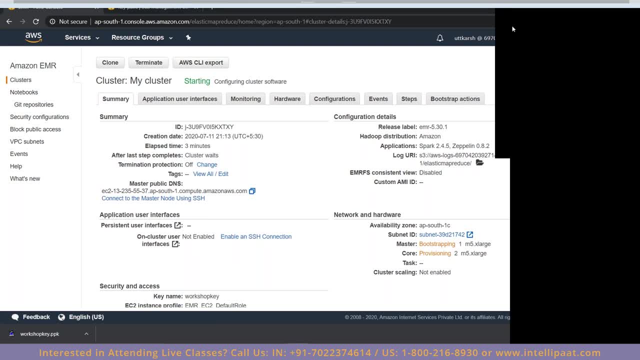 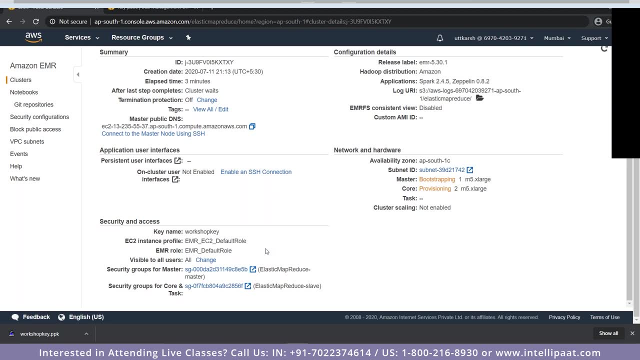 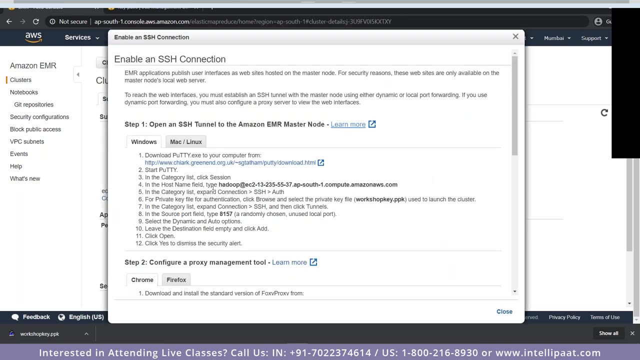 cluster has started right. so the first thing that we need to do is actually access the master node right. so the first thing that we need to do is get the uh host name for our particular master node right. so in our case, we can enable an ssh connection. click on that, it will actually. 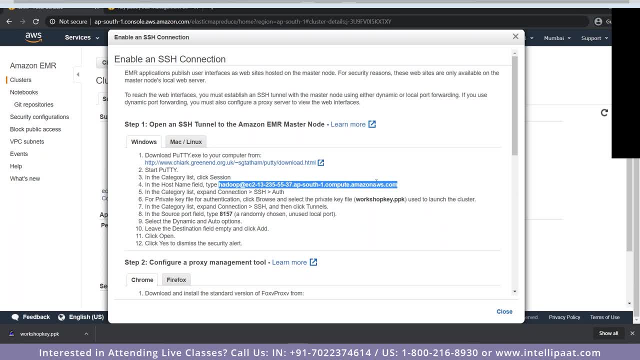 show you what you need to use as to enable your master right to say- this is another practice- say, you guys are watching me here today. uh, and i, if i had used a password instead of a actual private key file, so you guys would have been able to log into the server that i've? 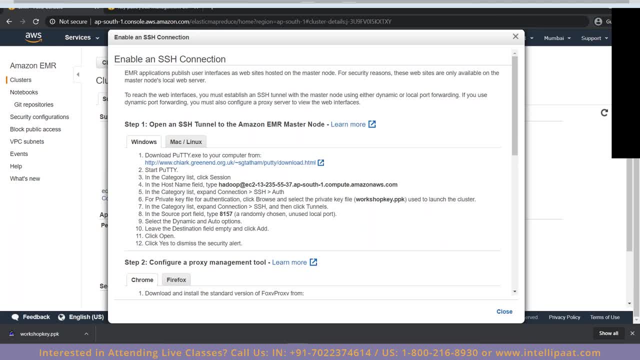 created the same way as i am doing right now, just because i've created a ppk file. you guys cannot do that. so that is also a very essential factor in public, private key management affairs, right? so that is why i created an encrypted file. so i'll copy this. this is what you need to copy and then 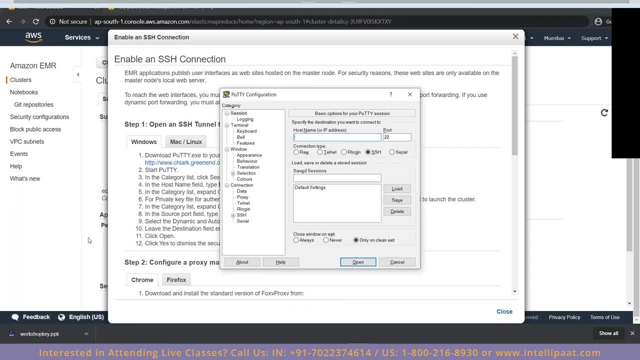 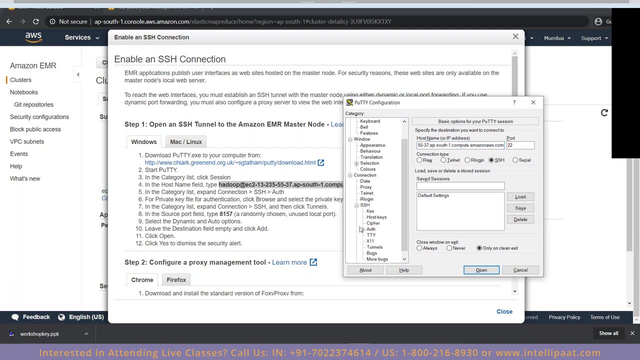 i'll simply open party. you can simply type in party on google. you'll be able to install it. so in the hostname i'll paste that, that at this copy right. and in order to remotely access this, i need to authenticate myself, and i authenticate myself with the new key that i have created, so i've 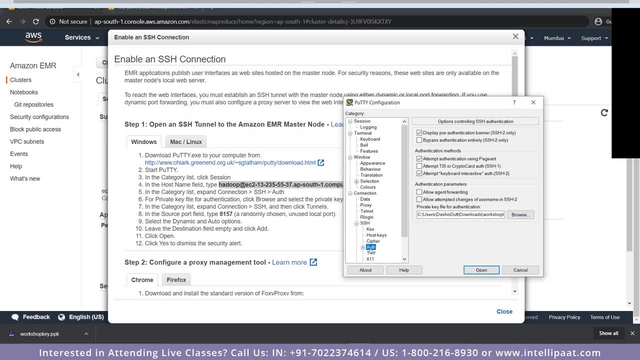 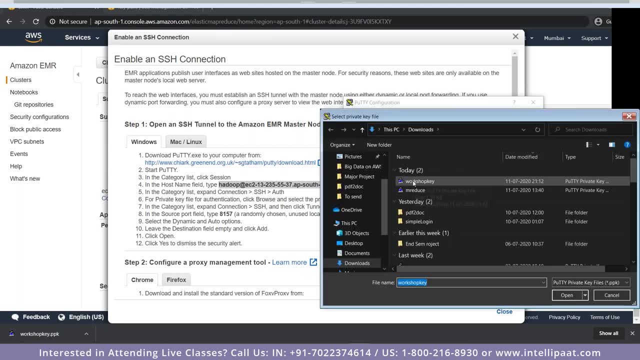 browsed it to that. so you simply go to auth and you double click on auth, it will allow you to browse to your particular ptk file. in my case it's workshop key that i had downloaded. i select that and then i click on open and i you can click this. 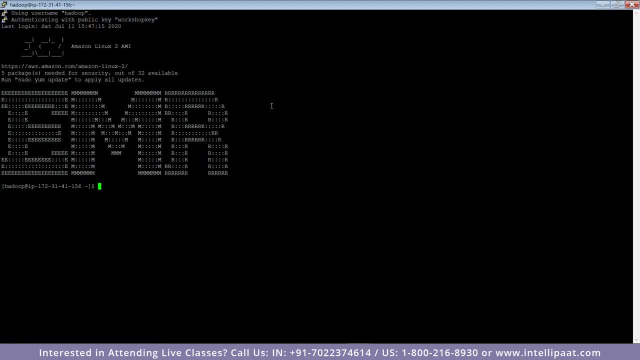 yes on this, and that will basically remotely connect you to the emr server that you created. so this is the master node. the two slave nodes, the two data nodes that are there are not accessible to you. you only access the master node. the rest of it, even if there are 100 data, 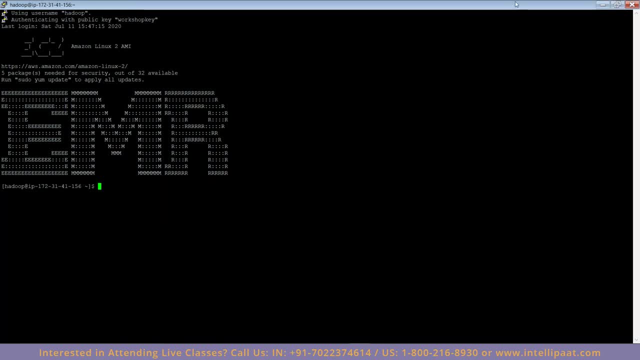 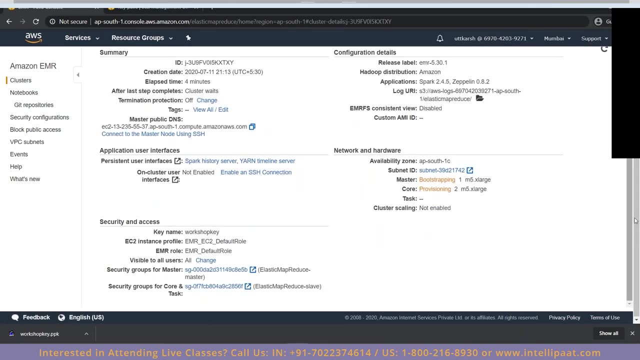 nodes outside of this. you don't need to care about them, right so now what we will do is actually upload our data to an s3 storage bucket, right so now. our processing framework is ready. what we need to do is get our data from a particular source, so i don't want to directly. 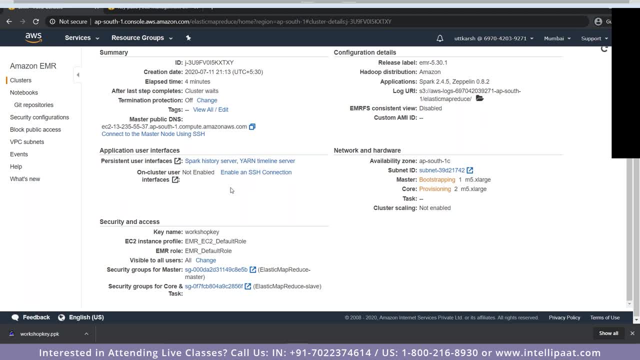 uh, put in the data using some sort of a remote, remote file transfer protocol. i don't want to do that because in a real world scenario, you'll be getting a data from an online source. so that is what we're going. that is what we are going to be doing, right? so let us just upload the data. 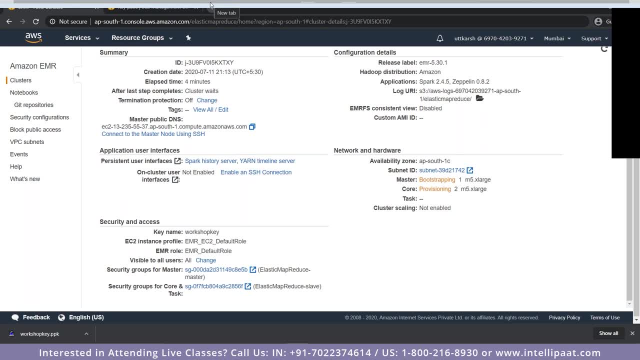 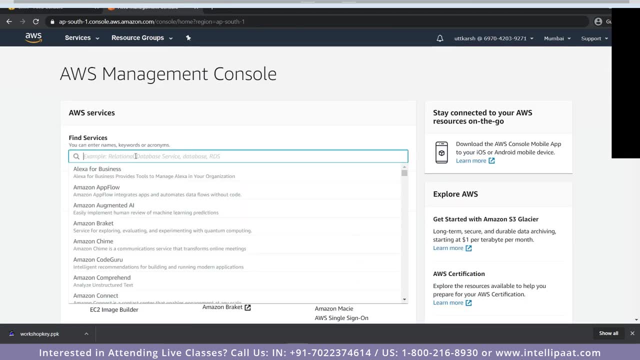 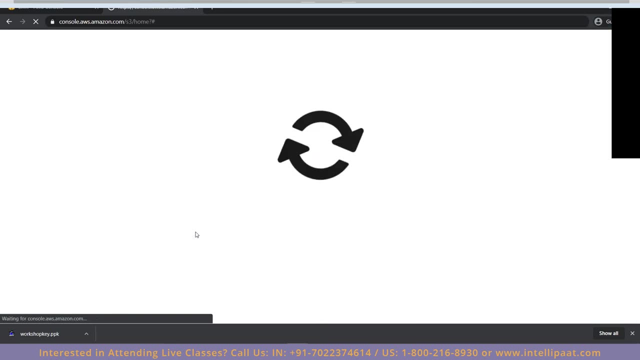 in an aws service ec3. uh, not an ec3, but an s3 bucket. so if i simply go up and click on the dashboard again and search for uh, let me s3, right, so this is the scalable storage in the cloud. uh, nominal storage is provided for this. 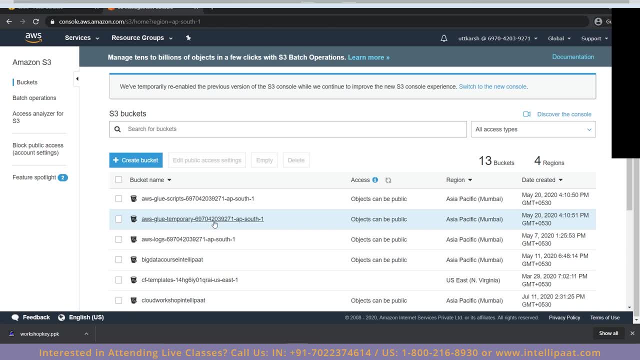 uh, up until i think, a particular amount. but if you want to uh rent like terabytes and terabytes of storage, then you have to actually pay for this service. other than that, uh storing some nominal amount of data on the s3 console, on the s3 service, is free of cost, you don't need to pay anything for. 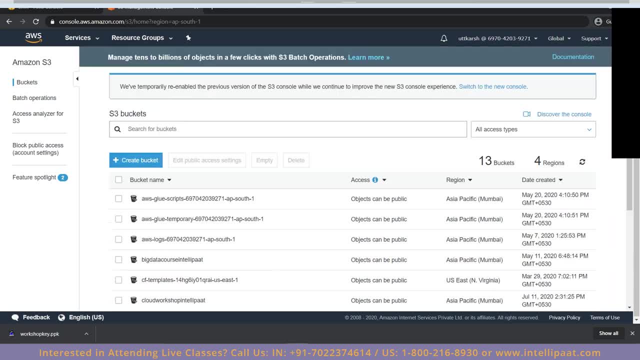 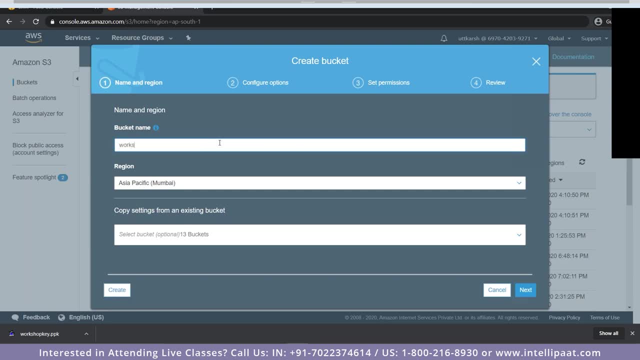 that. so the first thing that we will do is create a bucket, right? so, uh, we can call this bucket workshop practice. so the bucket also needs to be a unique name, like a username. you cannot somebody else in the world, in the particular region that you're operating in, at least. 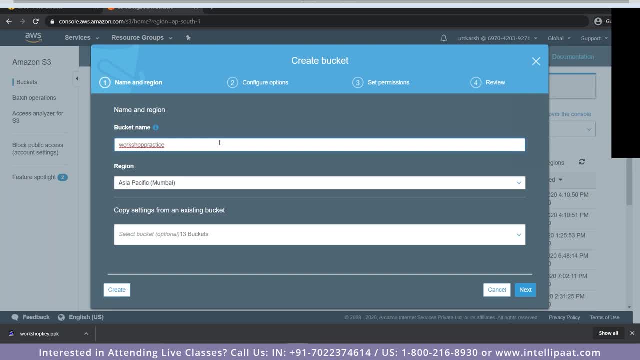 cannot have the same bucket name as you, so that will actually give you an error. so i'll just add an intellipath after that. so this name is probably not taken right. and then the region is asia, asia, pacific, mumbai. so in this particular region this name is unique. 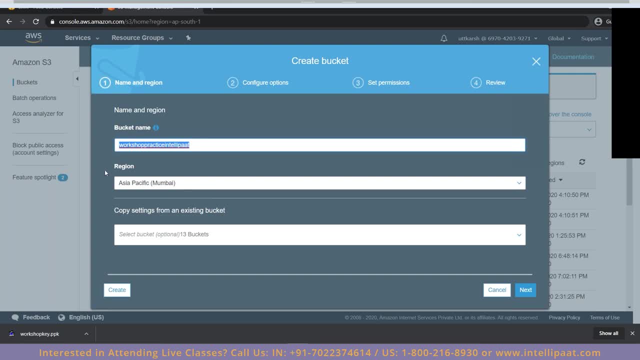 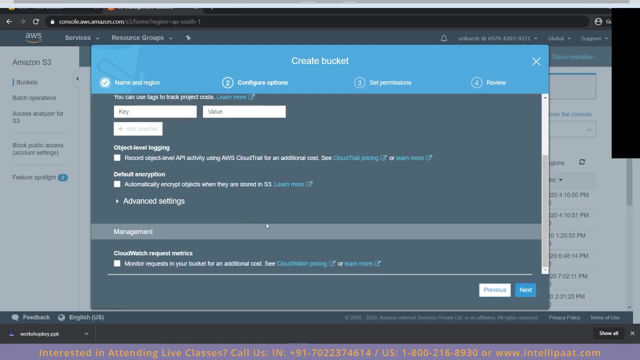 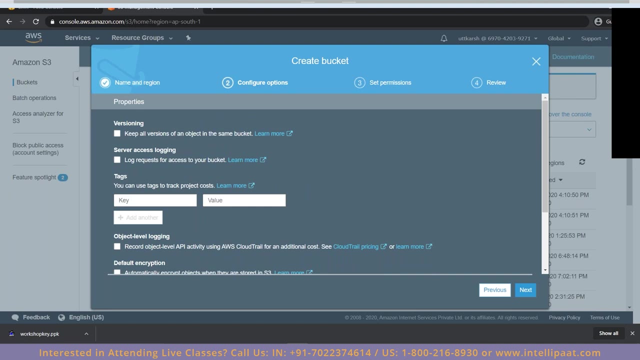 nobody else has used this name, otherwise i would have been prompted and error. and then what we will do is basically: uh, click on next and click on next. you don't need to actually care about this. we don't need to particularly configure any options. let me see: we don't need. we don't need. 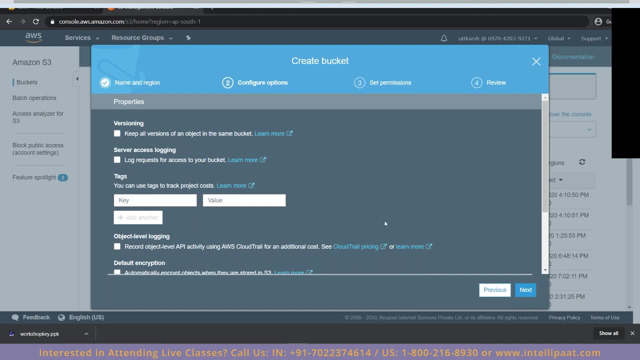 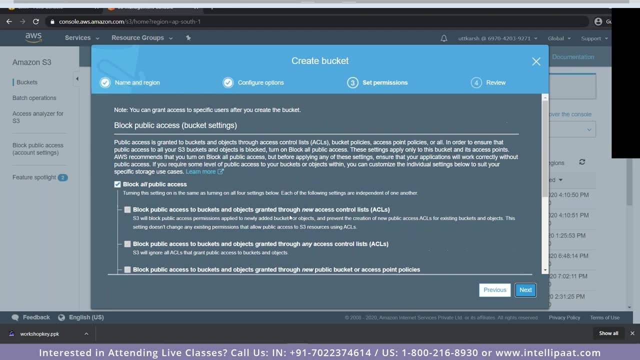 to uh configure any sort of logging, because this is a basic bucket. we don't need to do that right now. so yeah, here is where it comes in. uh, right now, by default, what the s3 would do? it would block all public access. so if you're operating from anywhere in the world, 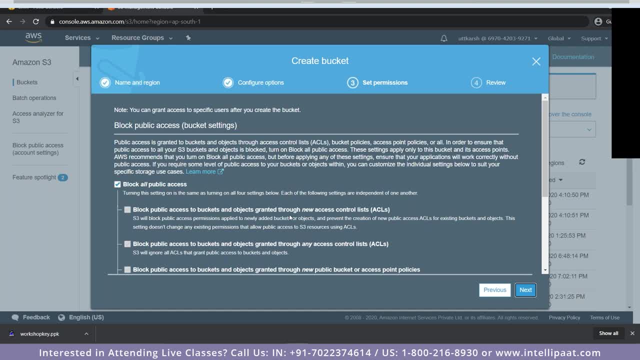 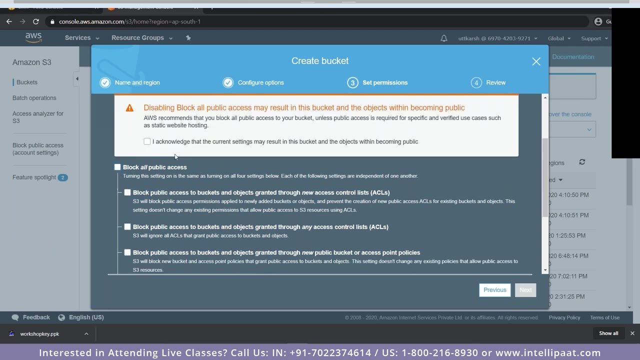 uh, you can basically have your amount of data security and it will basically block anybody else from accessing your bucket, right, so you can store your data safely and nobody else will be able to remotely access it or basically open up your links. so we'll basically unlock this for now, uh, because 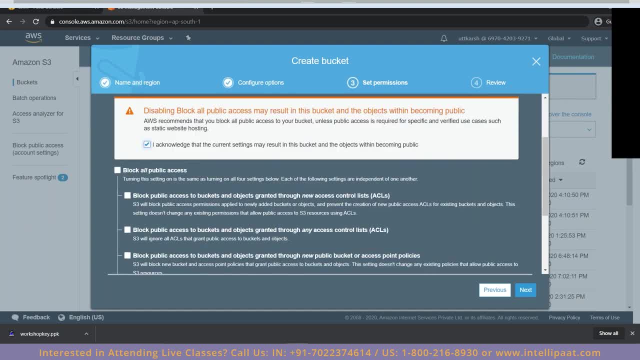 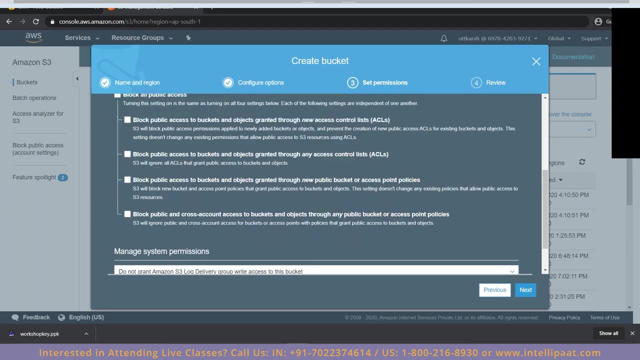 we are going to be accessing it through our cluster. but, uh, depending on the organizational policies that a particular organization has, you can unblock it, block it and set up a particular im role for that so that only a set individuals can access it. so a lot of things are there, but 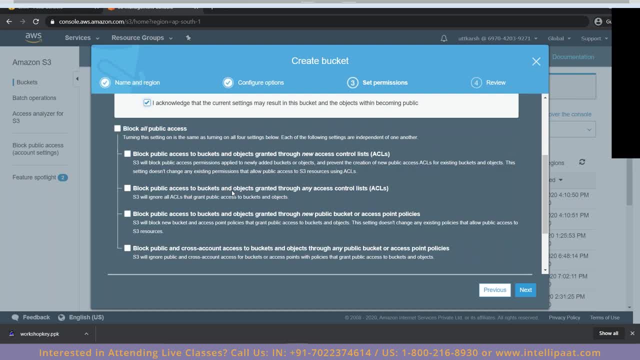 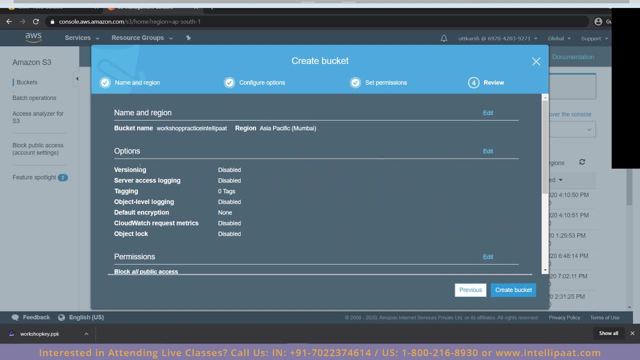 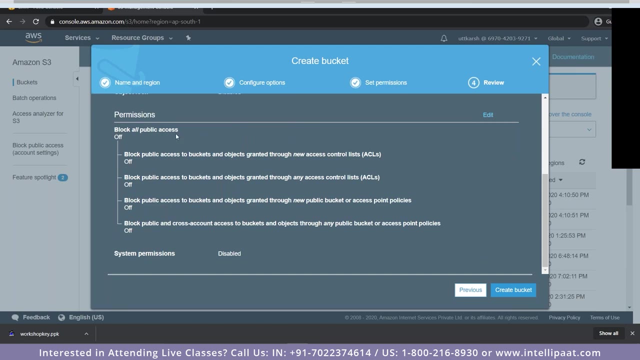 for now, for demonstration purposes, we'll unlock it so that, uh, we can access it without any issues. so click on next. so, as you can see, we it gives us an option to review everything. so we've named our bucket this and, uh, the block. all public access has been turned to off. so 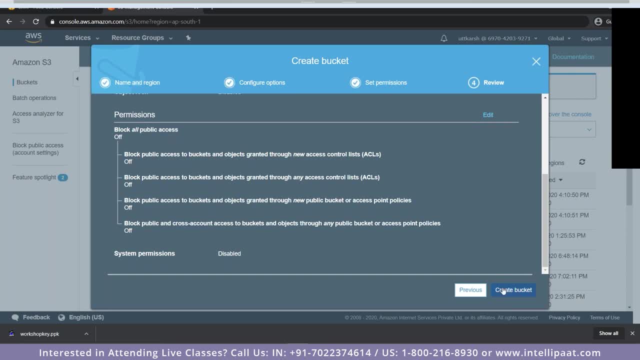 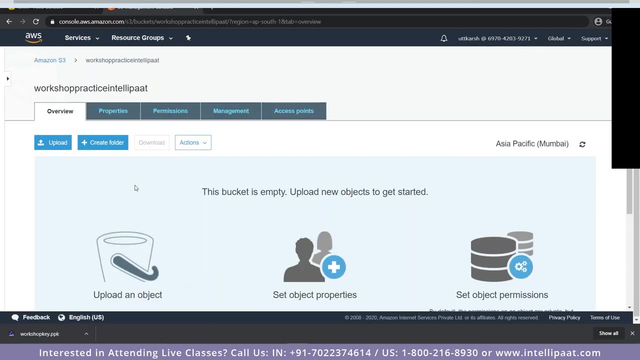 we can basically access it with our emr cluster and then we can create our buck. so just simply scroll down and here we can see workshop practice in telepath. here is our new bucket. yeah, so, uh, if, unless, uh, some of some of the people have doubts about the storage space. 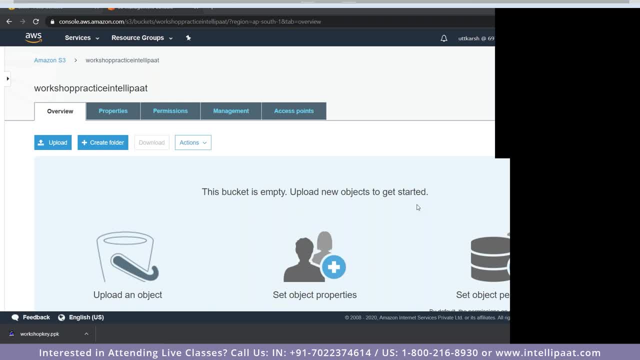 so, uh, unless there is, you're renting a huge amount of storage space, like a terabytes worth of storage space. uh, you're not going to cost anything for it. uh, if you want to scale up the storage space that you have, then only you have to, uh, basically pay amazon for this. otherwise, this service is free. 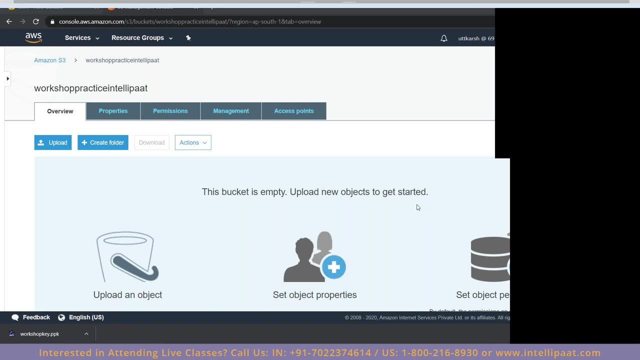 the s3 service that amazon provides is free, yeah, uh. deepak is asking: why are we creating an s3 bucket? we are creating an s3 bucket because we're going to be using, we're going to be uploading our data set onto the s3. uh, we're going to be uploading some data set. we're. 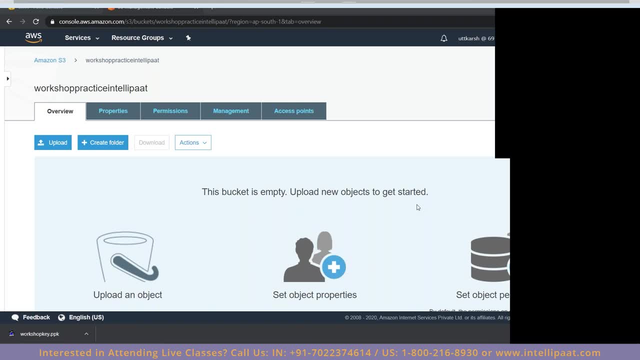 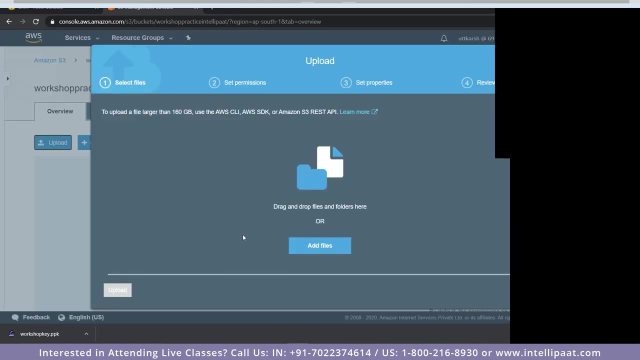 going to be doing some spark uh querying on that data set, so we're going to upload it to the s3 and going to access that data uh from our emr cluster. so that is what we're doing, all right. so, uh, first thing we need to do is upload our data, right, so you can simply click on add files. it will. 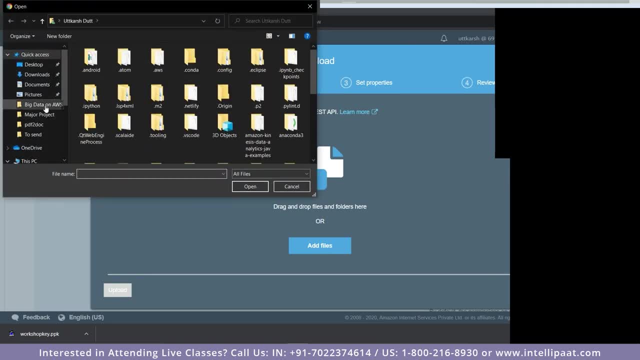 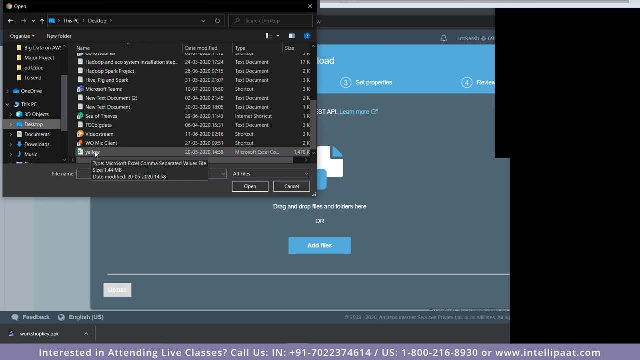 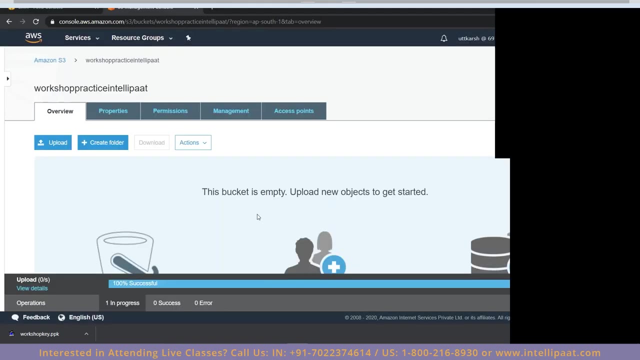 basically prompt you anything that you would want to upload. so right now, if i go to desktop where i've situated my uh- okay, so here here i have my yellow dot csv. i'll just show you what their data set is. if i simply click on this and click on upload- about 1.4 mbs, pretty big data set. 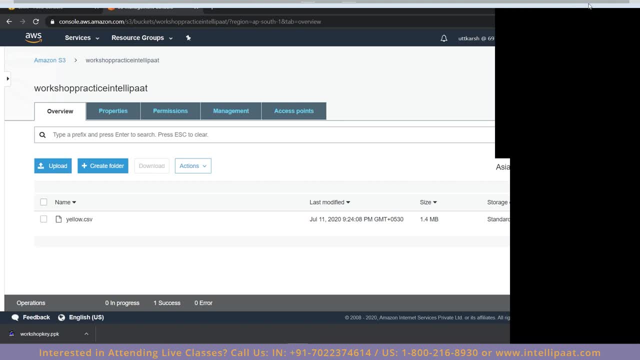 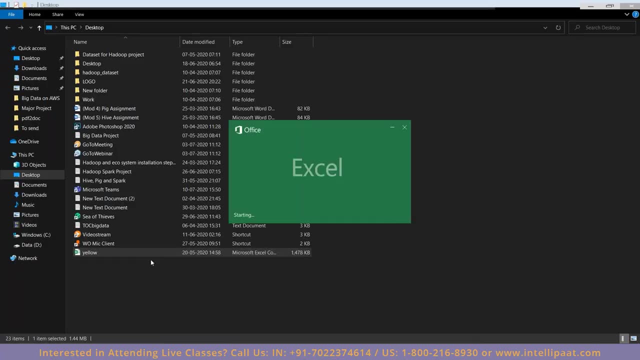 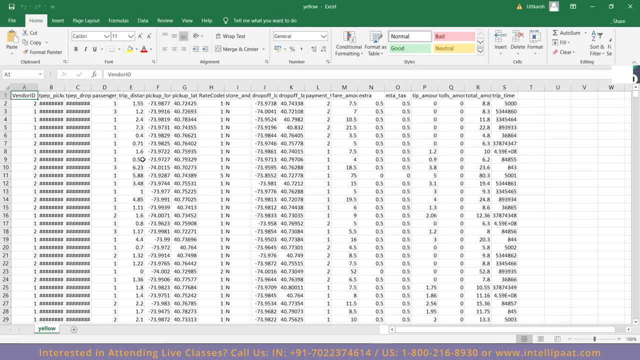 okay, so, uh, if i minimize this and show you guys what that data is, so this is my yellow dot csv. so, as we can see, if i expand this, so here is basically a taxi data set like uh, an online gap service data set. so you have ola, you have uber, uh, you have all of these, uh, taxi services that. 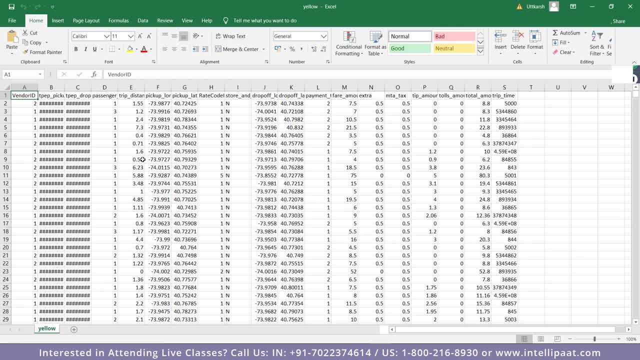 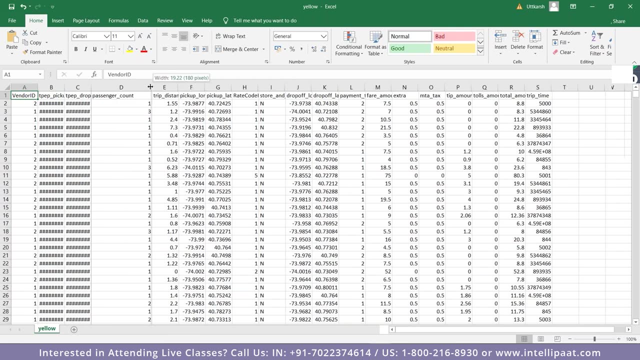 you use today. so a taxi service also generates a lot, of, a lot of amounts of user data. so this is how it looks like, basically. so, uh, firstly, you have the? uh pickup times, you have your drop-off times, you have your uh the passenger count that was there in the taxi, you have the distance of. 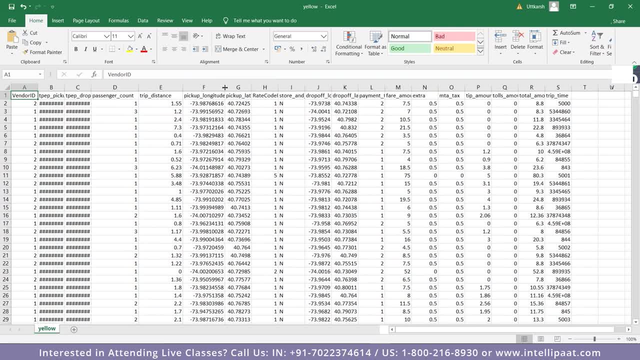 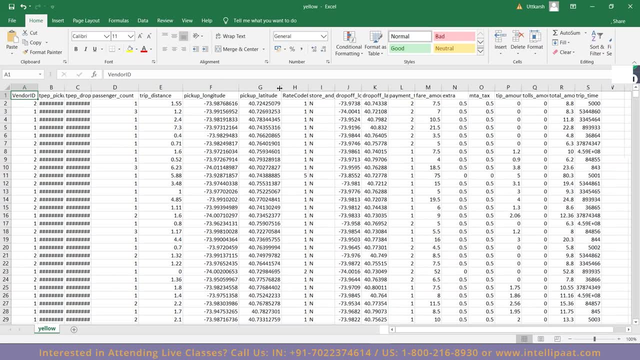 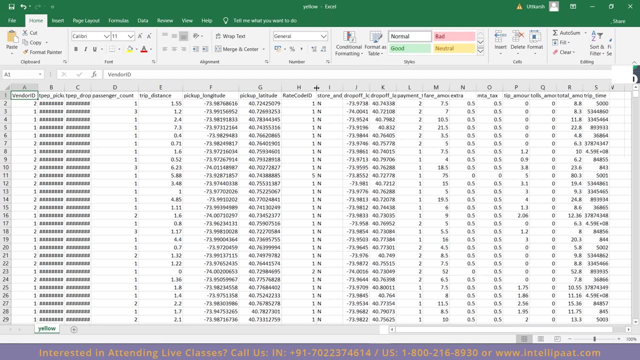 the trips. that is calculated. you have the uh longitude of pickup, you have your latitude of pickup. so basically, the positional, positional, geo-positional data, that is where you've been picked up and there you have to be dropped off. uh, you have your rate code id, which is something i think it's about the ratings, and uh, you have your. 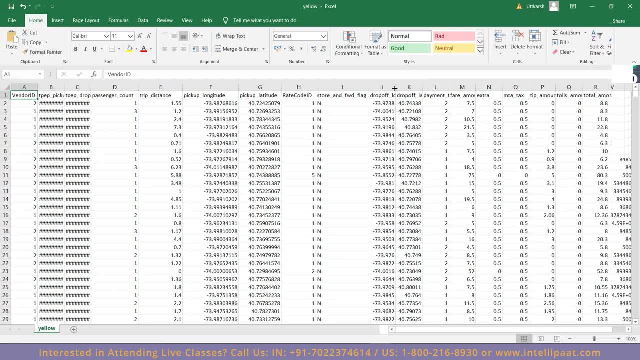 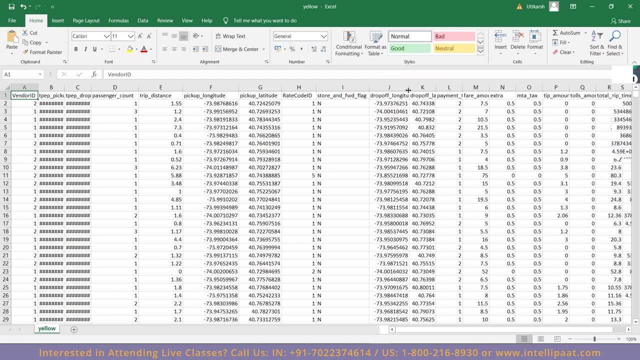 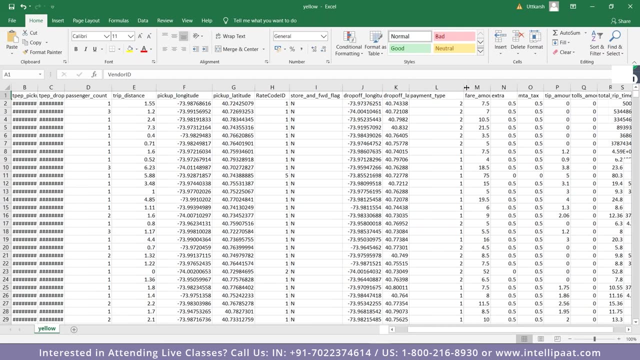 storage and forward flags and other other- basically other- column names for that. right now, all we're concerned about is the fares and the payment types, right? so we're going to be focusing on the revenue generated by this taxi data. so you have your uh payment type, which is two, two stands. 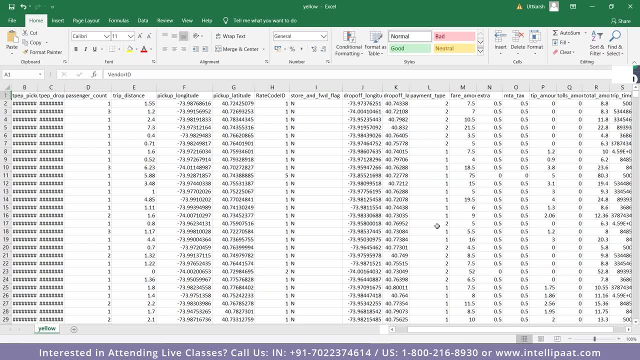 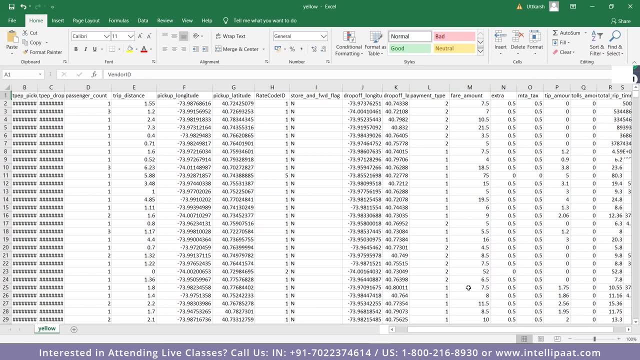 for, basically, it could be online payment. one stands for cash payment. uh, there's also three and four, which could be for card payment and other payment services as well. the fair amount is the fair that is taxed, the extra amount that is there, the mta tax and all the taxes. 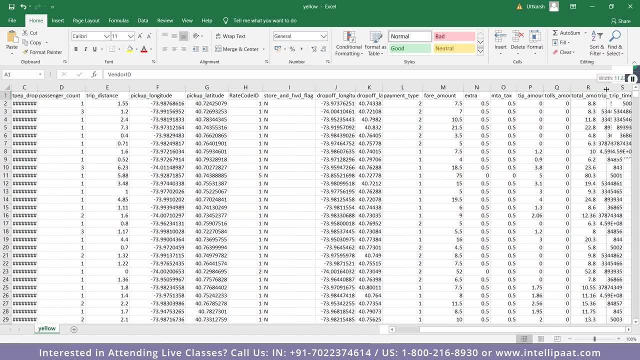 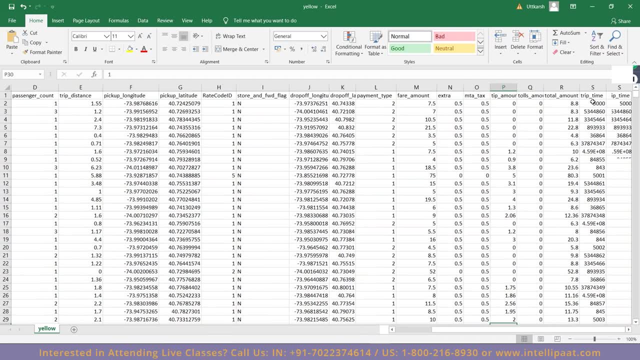 so the total amount that comes to the customer is in the total amount. so that is the column which actually tells us what the revenue is, and then there's a trip time. so this is what, basically in seconds, essentially, uh, what the trip time is, basically what, how much it took. so, yeah, so this is the data set that we are going to be analyzing today. 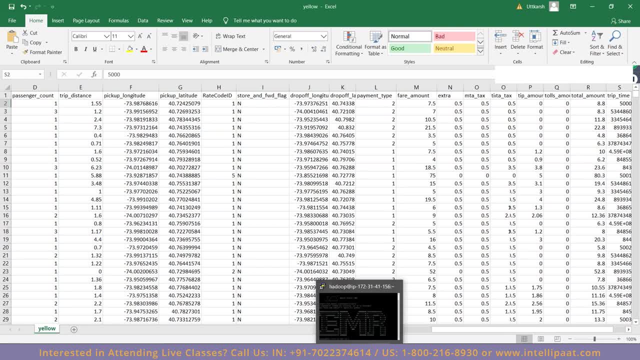 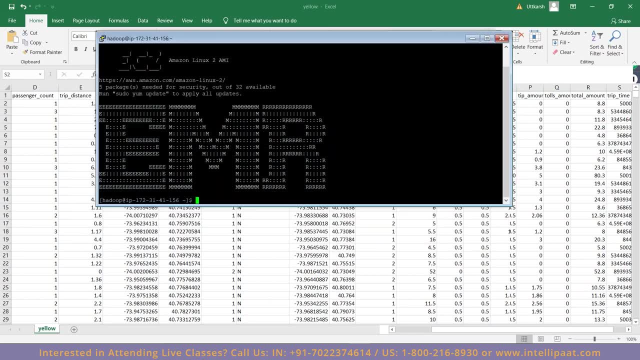 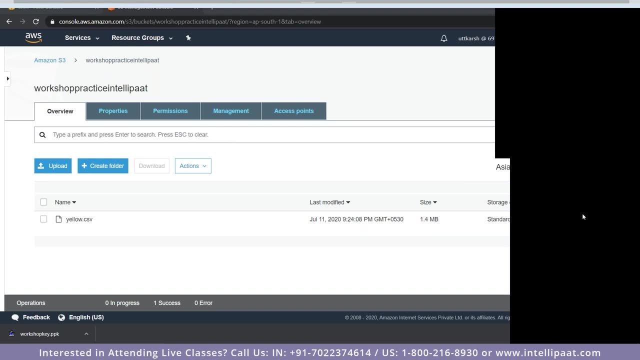 and then, uh, we're going to open up our 40 again, which is the remotely accessed emr server. yeah, so nathan is asking: how is this going to work? so we're going to be doing this right. so now we're going to be accessing this. 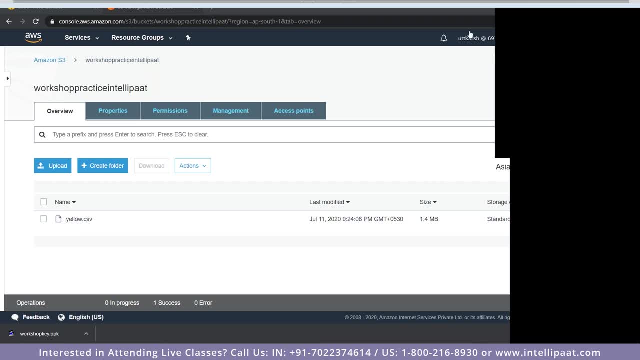 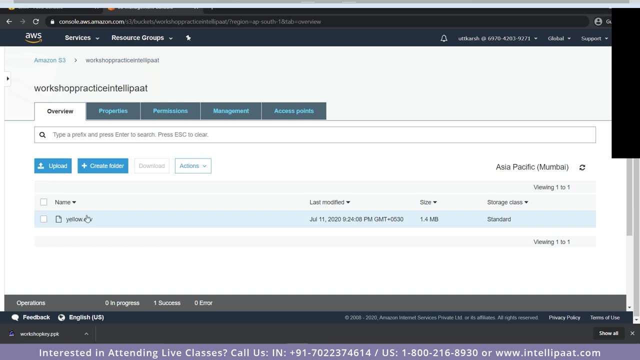 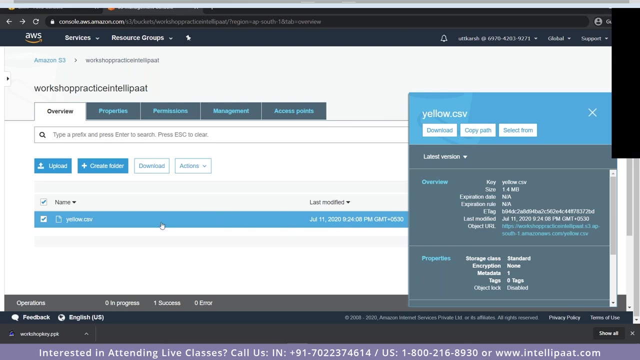 yellow dot csv, which is the file that we just uploaded. so we're going to be up, we're going to be basically importing this into our data nodes. so how does that happen? click on the file, right? uh, not actually click on the file, just click on this. click on the file engine in the general reduction. 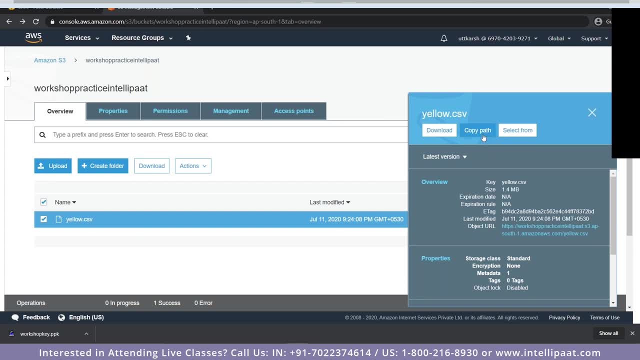 not on the file name, on the general function, and then there's an option: copy path. so this copy path is the same as the object url. find your object url redirect you to a web page. you don't want that. you want the actual file path. so for that you'll simply click on copy path. so i'll show you how. 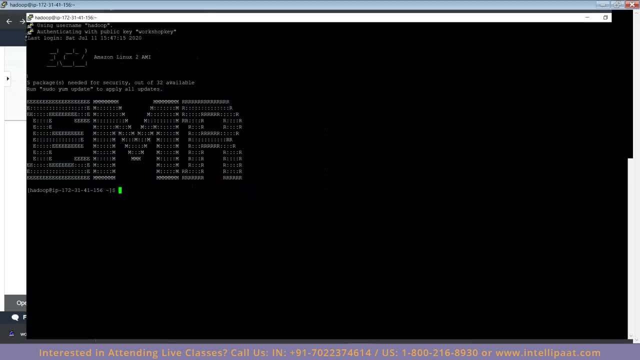 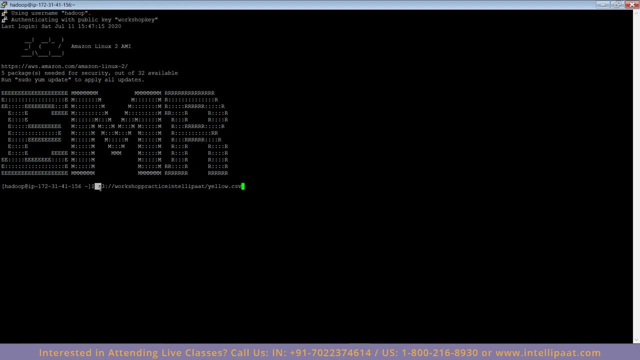 this actually looks. i simply expand this because- and yeah, so this is how it looks. uh, this is the file format that it looks. it doesn't have the http protocol attached to it. it has the s3- s3 protocol. so that's a. that is how the difference is. the first thing that we need to do is start a spark. 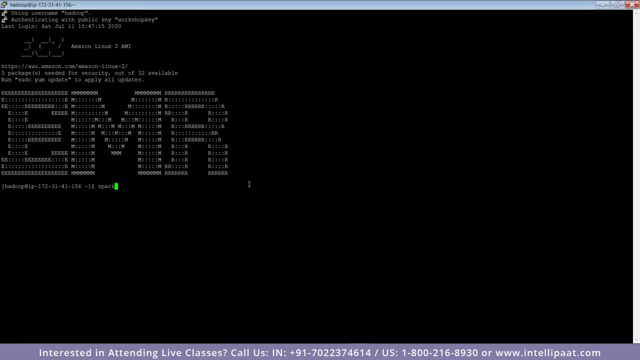 session. so, uh, the way of spark operates is whenever there's a spark session operating, as long as the spark session is active, that data is in within the ram. whenever the spark session ends, when the sparks job ends, basically you end the job. so when that happens, your 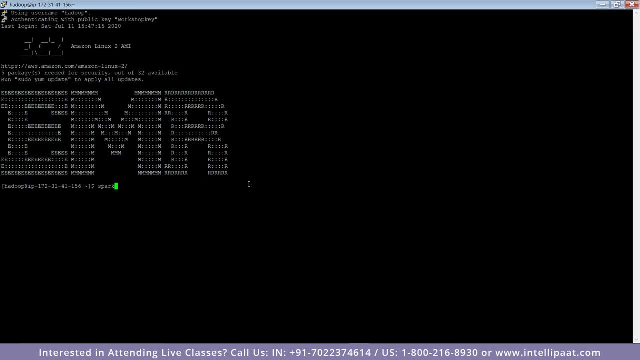 ram is cleared off of that memory, the garbage is collected and, uh, if there is some data that's there that has to be stored, it will be stored on the disk, and if it doesn't need to be stored, it will not be stored in this. so you can use spark for data querying. you can use spark for data. 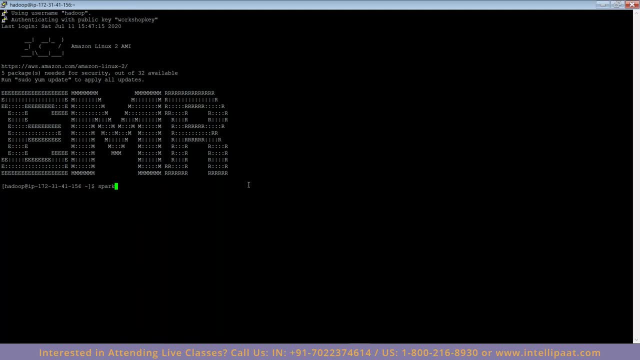 warehousing as well. you can do all of these things. so this is what spark is. it starts spark, the sparks spark installed. you can simply type in spark shell. so what this will do is start up a scholar shell with the spark libraries already important. it takes some time to happen, so we've successfully. 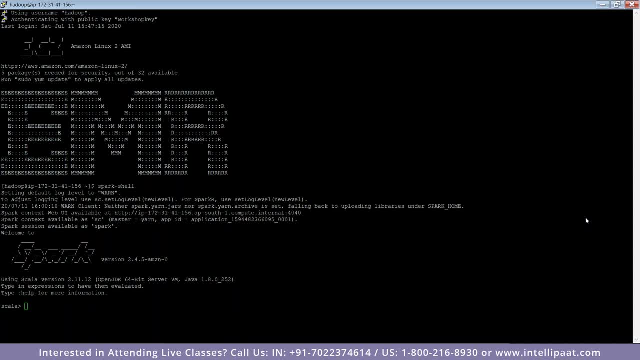 created our spark ship kartish is asking: ip will be created automatically. when we yeah, the host name will be created automatically. you will not be given the ip, uh, you'll be given the host name for the master node. it will be created automatically. whenever you clear, whenever. 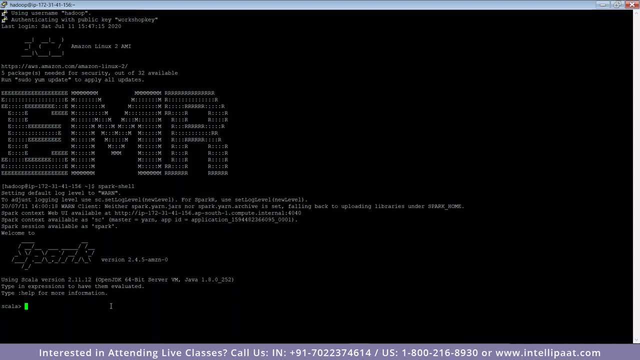 you create the cluster. so as long as your cluster is not terminated, the host name will remain the same. but if you terminate the class, uh, the cluster, the host name will be lost forever. so you cannot use the same host name again. so just so people don't have to do that- they. 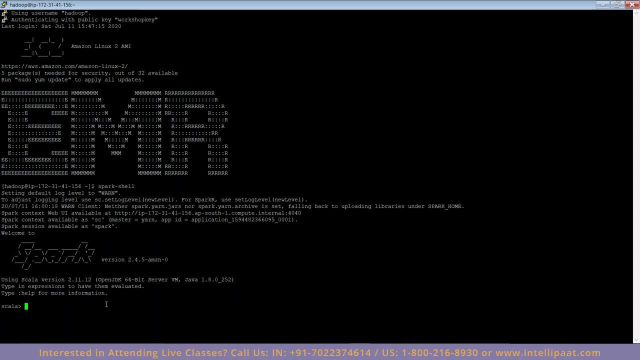 generally in an organizational space. they generally we keep the cluster running, uh, because they only have to pay for whenever the job is job is being done in that particular cluster. so that is why they do that. so the first thing that we need to do is create a data frame out of that uh, yellowcsv. 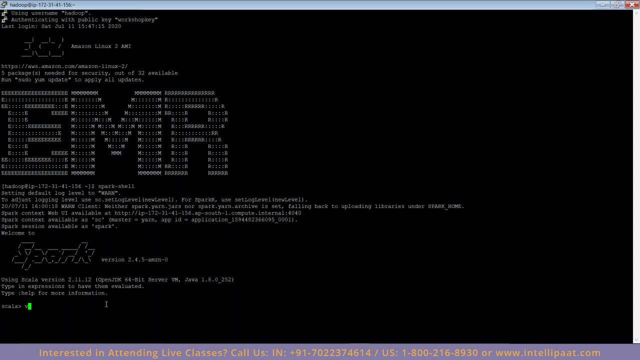 file that we just used, right, so we can do this. this way, we can create a value and call this dfc. this is basically an object. df is an object. create it to uh, spark, dot, read, dot format and we can specify the format of file. so in our case it is a csv file, so we will format. 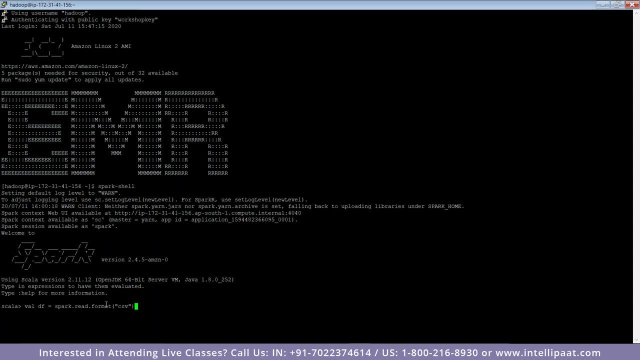 csv, which is a comma separated values file. so that's it, and then we can add some options. we want to include the headers, right, we want to include the column names. so we'll include the column names setup and we will give the value as true. so we can add other options to this as well. so for memory management, for basically accessing: 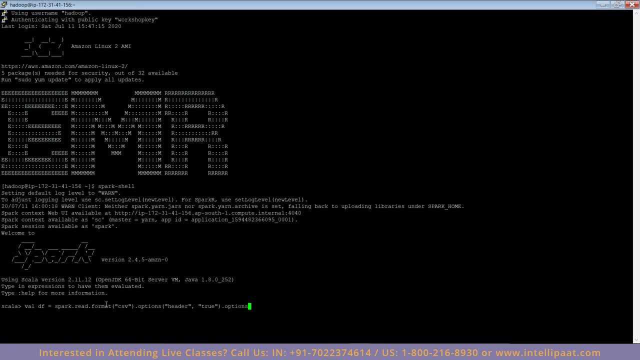 this particular data data file as a schema, because we're going to be creating a data frame out of this. we are going to infer this as a schema. so this is another option that you can put in and put the value as true, and for memory management, and for memory management purposes. uh, we'll also. 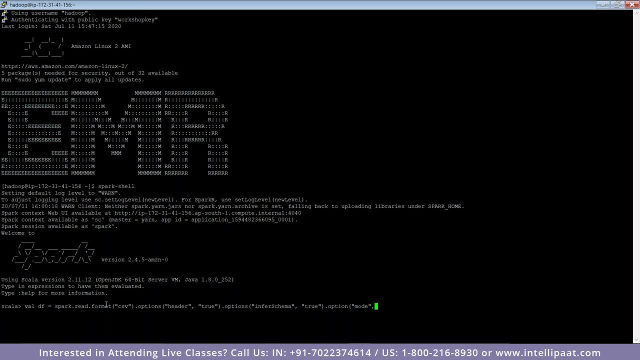 create data replication for this by using the fail fast method. now that all of that is done, we can simply give the location to the file, so dot load and then, given the location of the s3 bucket, the bucket file that you use- right? so i already have it in my clipboard? uh, actually don't. uh, i'll have a. 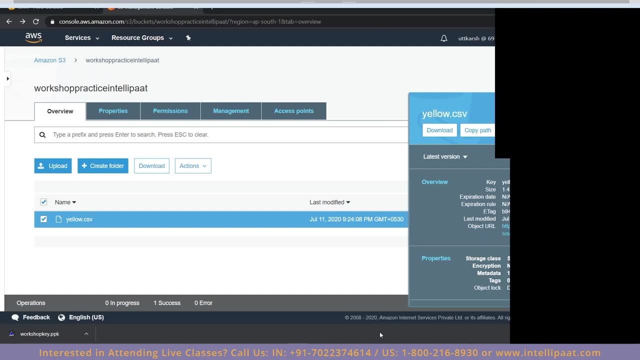 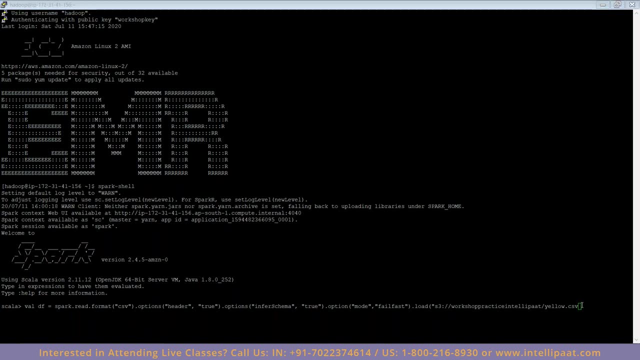 to do it again. okay, so i click on copy paths, remove this and, given that particular location and double quote, back it at close, double quote it close and press enter simply so that will basically load the data into the data frame and divide that data equally throughout the two rams. 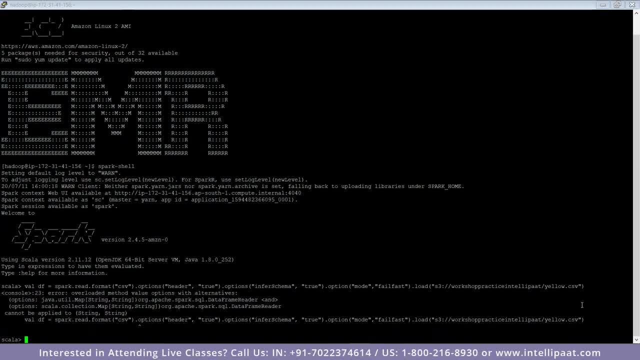 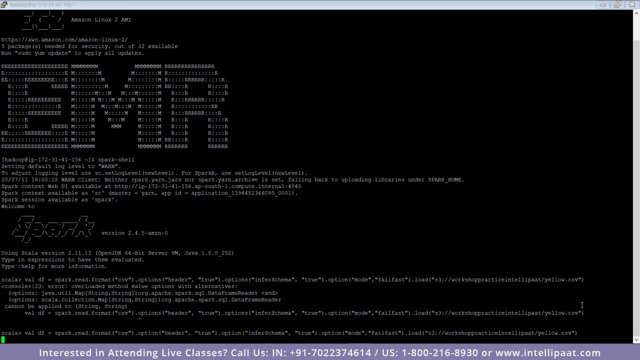 present in my data nodes. press enter. so there's some error with that. oh, i just put in options instead of option. that is an issue. they're going to do that syntax issue and then you simply press enter. so that should work. so it will. you will see the gradual process of it actually importing. 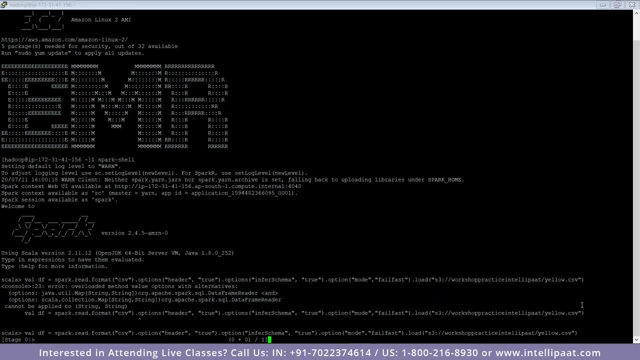 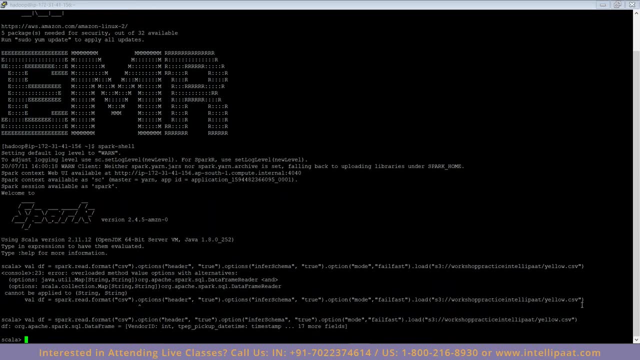 the data. you'll see that right about now, so it's on stage zero right now. since it's a big file, it will take some time to create a data frame out of it, so it did it almost instantly. so, as we can see, uh, the data frame has been created. 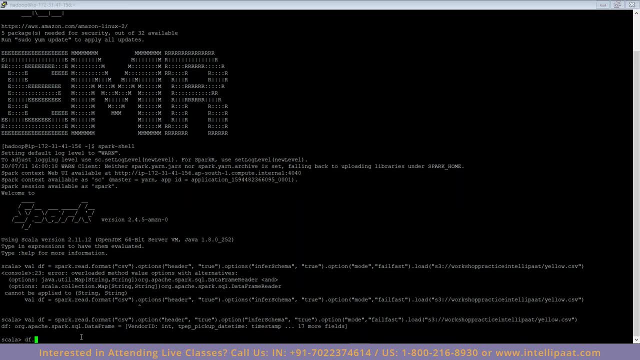 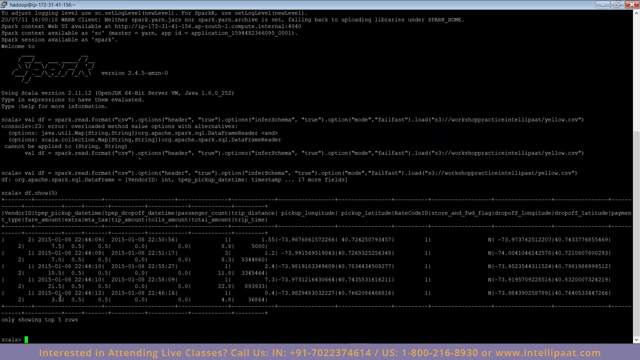 right. so just to confirm that, if i simply type it df, dot, show and type in like i want to see five records, four records, uh, out of this data frame, five records, press an enter so as we can see: uh, it's not actually completely in the screen frame. that is why you see all of this gibberish. 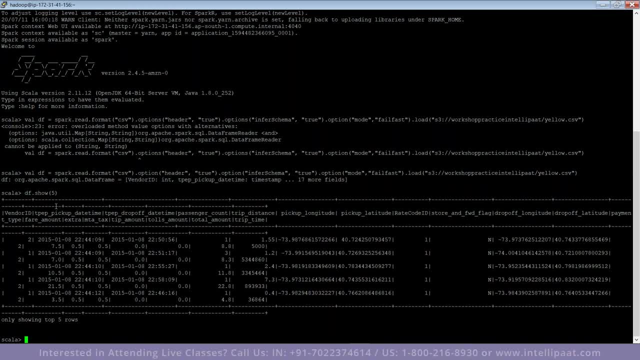 but uh, what happens is: uh, it is in that format, as the first header format isn't. so, as you can see, the first value is vendor id and the pickup time and the drop of time and everything. so that is there. it is in an actual sql table format. so we've successfully converted a semi-structured data. 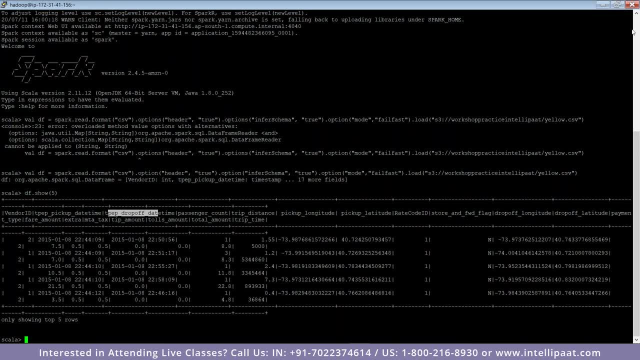 set into an sql table type format, right, so now we can operate on this in an sql sql type way. so just that you know how that happens. okay, so the first thing that we need to do- and this is important for the readability purpose of it- and to actually access this data as a from the 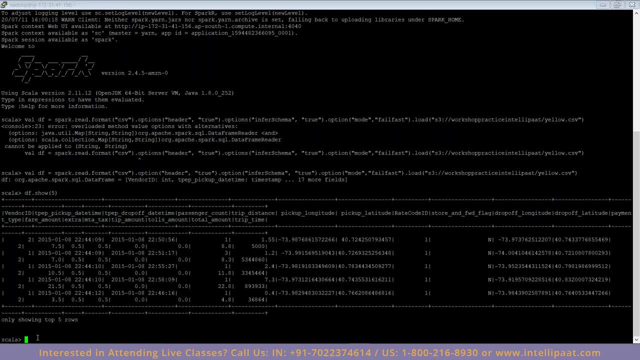 SQL context that we will be using. we need to give a temporary name to this: dfcreate, or replace tempview and then simply taxi data. so what does that mean? right? so, just basically, this DF is the name of the way data. so what does that mean? right? so, just basically, this DF is the name of the way. 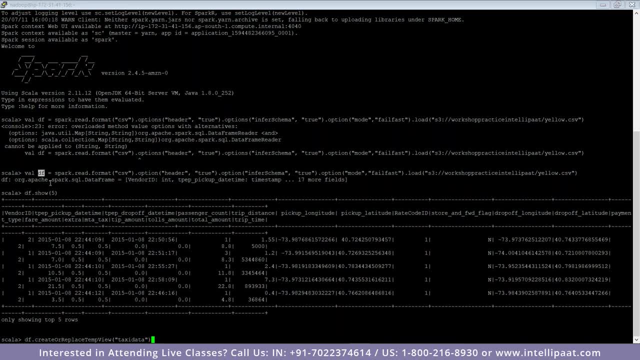 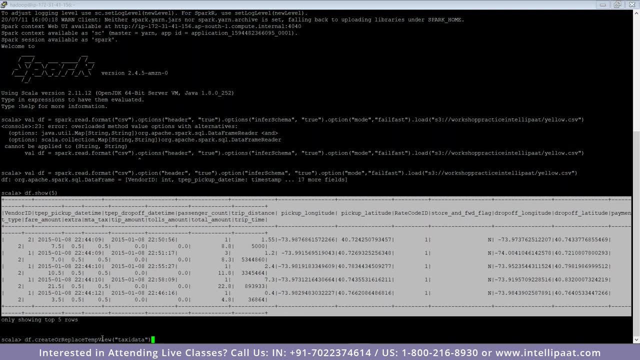 that we're using this object name in the Scala shell that we're using. what we want to do is try to access this data frame that we've created as an SQL table. so for that, we are renaming this in the SQL context and I'll tell you what the 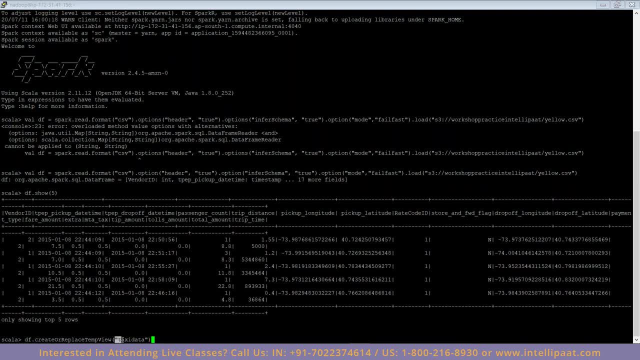 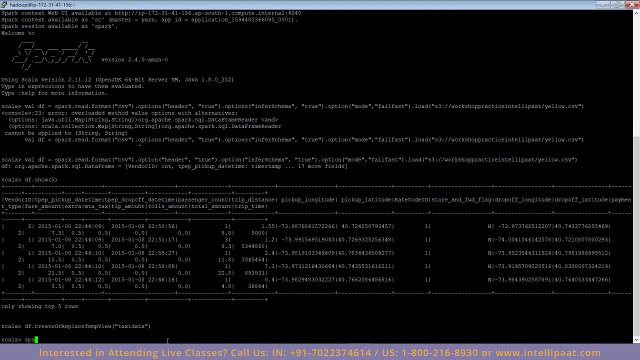 SQL context is in a bit. we are renaming it to taxi data, so we'll simply type in things like: say, we want to use SparkSQL, this is what you will use for accessing that data in an SQL format. say a basic SQL statement like: select some, so this will select the sum of, let's say, like the 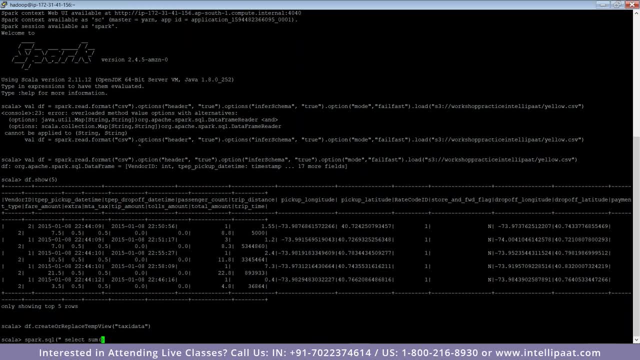 sum of everything. we want to collect the sum of, say, the total amount, right? so this is the total amount that we are. we want to collect the entirety of the total amount, so all of the revenue that is generated. right? so we type in the column name the exact column word-to-word total underscore. 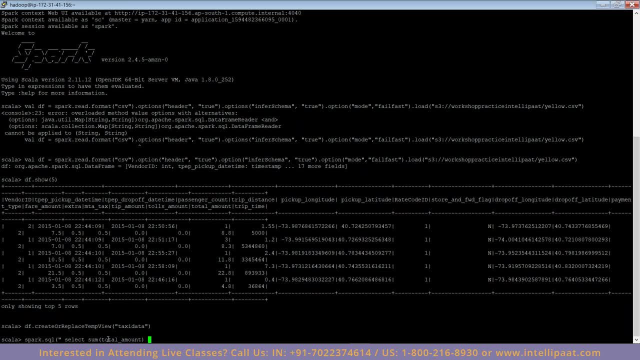 amount and then, similar to people coming from a relational database background, you type in from and given the table name. in our case, we've named the table as taxi data. so what we've done essentially right now is actually, without having to use a relational database, an SQL database we've mimicked. 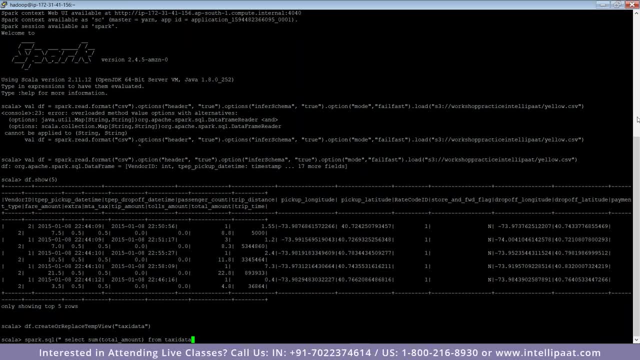 it using spark this moment. so, similar to an SQL statement, you will type in Spark dot SQL and you open up the double quotes and whatever you add in the double quotes is basically equivalent to what you would type in my SQL, right? so you've renamed the DF, this particular data frame, as taxi data. 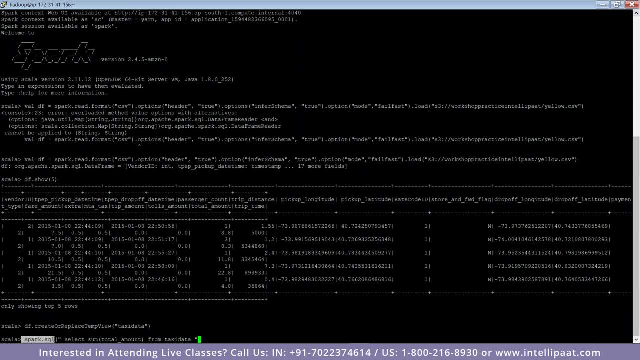 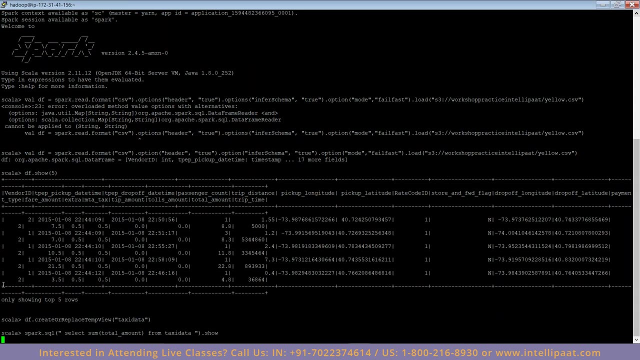 and you can basically query it as that only thing. you need to add a spark dot SQL and a bracket over here and a dot show so that I can actually see the output that you've created and present. so it takes some time to process that data, but once it does we'll see the actual output of all. 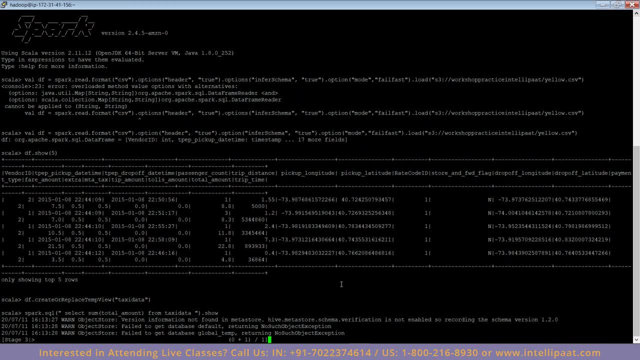 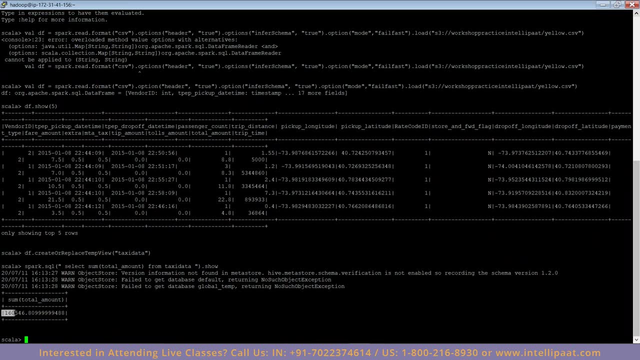 of the revenues that are there. so, as we can see, it took some time, but about a hundred and sixty thousand dollars or rupees- whatever the unit for that particular amount is- is that. this is the complete total amount and it's there, available for you, right? so imagine you have terabytes and petabytes of data. you cannot possibly calculate the total sum. 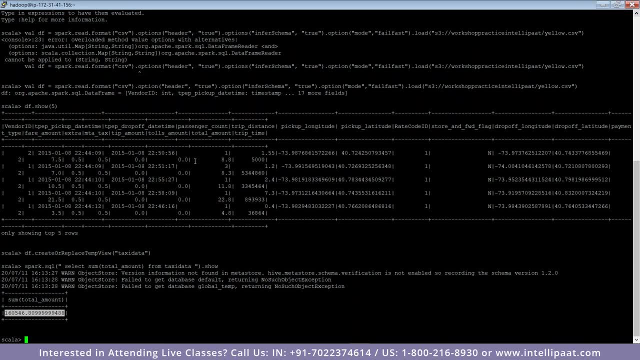 if you're using my SQL on a single system, you cannot possibly fathom to do that. first of all, you cannot store terabytes and terabytes of data on your system. even if you are able to afford that much hardware to store it, your processor will simply take days and days and days, even months. 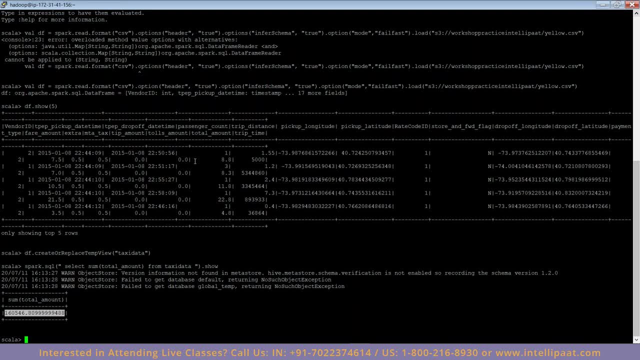 sometimes an year to actually process that amount. depending on the processor that you have, depending on how many threads that processor has, it will take some- somewhere from weeks to months, to actually process this amount of data- not this amount of data that I am currently processing, but if you were processing a large amount of data, like in the terabytes and petabytes range, 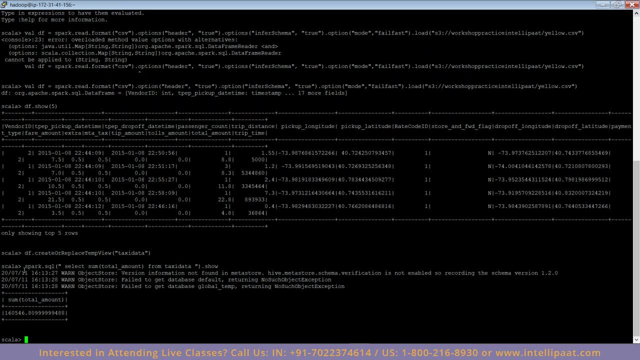 basically and all with this particular simple statement, no complications at all. this simple statement and you basically get the sum of all of the data and any querying statement that you would add, basically, so, yeah, so we can do some other things with it as well. right, so let's now get. 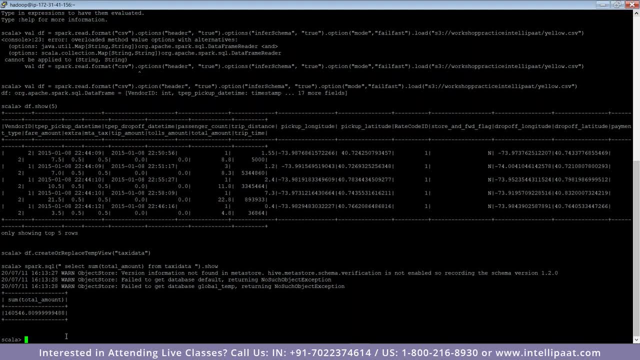 into the MySQL part of things, right. so the other things that we could do is, uh, say, we want to calculate the total number of trips- right, we want to calculate how many trips have been taken. okay, simply do a select and you can do a count, and you can simply type in star. star basically stands for every data record that is there. so 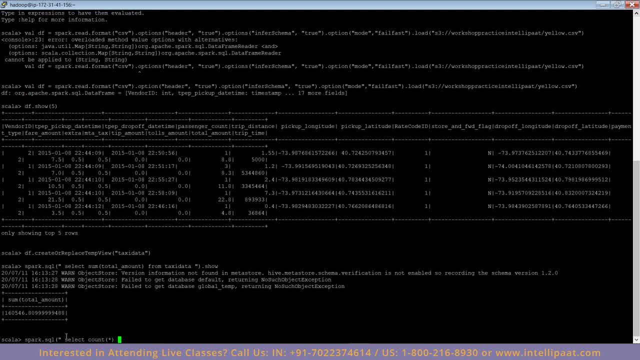 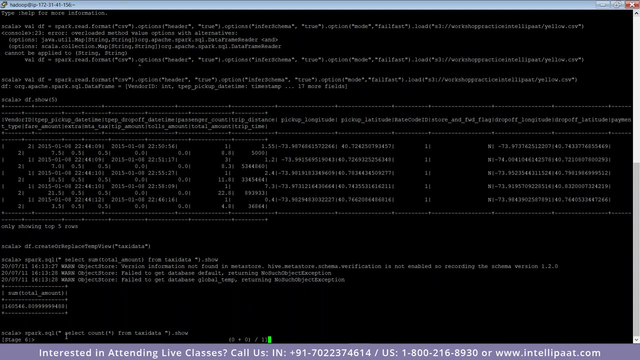 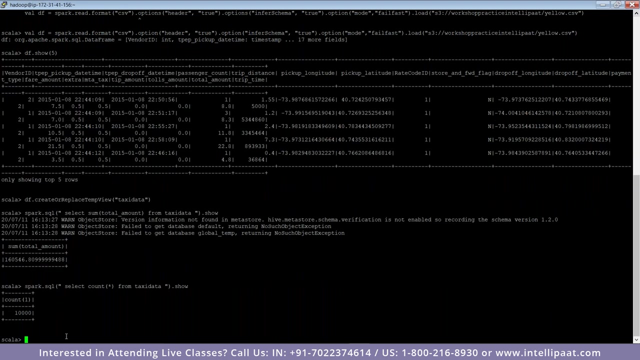 you want to count the number of data records, so that is the number of trips, and you can take some time, but this is nothing compared to uh. this would take the relatively same amount of time, even if you're actually trying to process terabytes and terabytes of data. that is the thing. 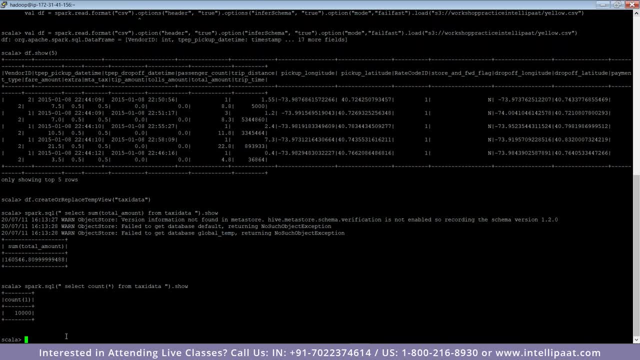 here. so you might think that in some in so so, so few accounts, it's taking this much time, right? so how will it, uh, perform on a big system, on on a big data set, right? so the thing about that is the reason it's taking this much amount of time. it is that it is because it is a standard. 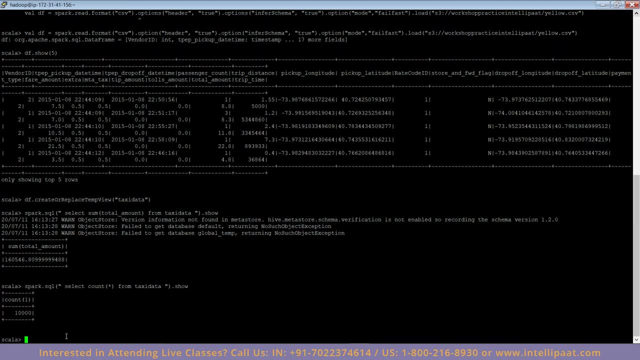 amount of time taken by a big data cluster. right? so right now I am doing the wrong thing. I actually processing a small amount of data with this enormous cluster that I have, but in a real world case, you would be processing terabytes of data. so in that case, also depending on this, 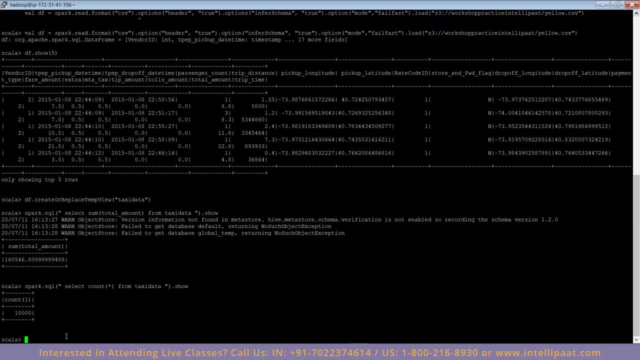 cluster size that you have, how much it has been scaled up, that data that you receive. Хорошо je mondo. you have, how much it has been scaled, how many instances are there and that's over. depending on that right, you will get an optimum performance out of this. so, in the same time that it can be, 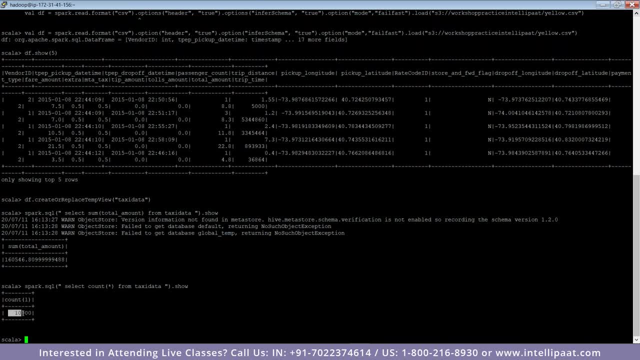 that calculated how many records are there, which is 10,000 records, right? 10,000 records. in the same amount of time as that, you would be able to calculate terabytes and terabytes of data. so that is the main advantage of Hadoop. then we could do something else: we want to calculate the percentage. 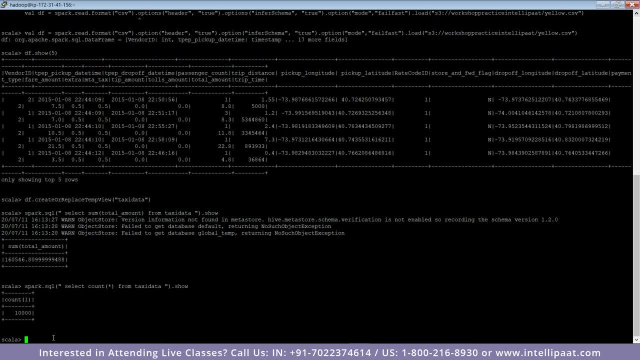 of how much tax has been implemented in the total fare. so we want to calculate the tax or the ratio between the tax and the total revenue that has been generated. we can do that as well. the time is bar on SQL. select the tax and the total revenue that has been generated. we can do that as well. 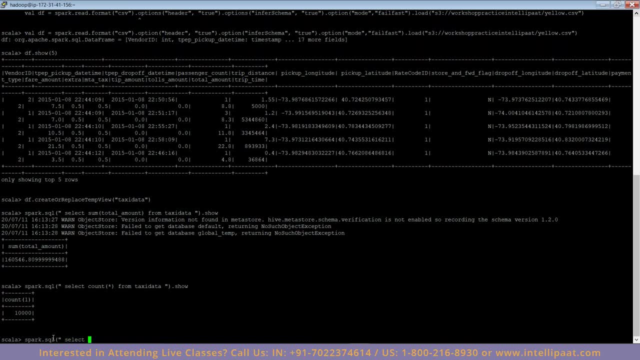 and we can give in something like um some, and we need to search the column name for the tax, right? so let me see here what is the column name for the tax? we can use the MTA tax, but let me use this tolls amount. let us use the toll amount, right? this is the column that we want to use. we want to use. 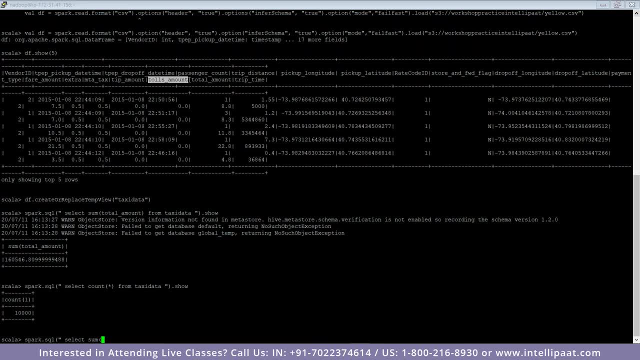 the tolls price. let's just discard the tax for now. let us use the total amount. we want to calculate out of the entire amount of the tax. we want to use the total amount of the tax. we want to use the entire revenue that has been generated. how much was spent on tolls? so we can do something like: 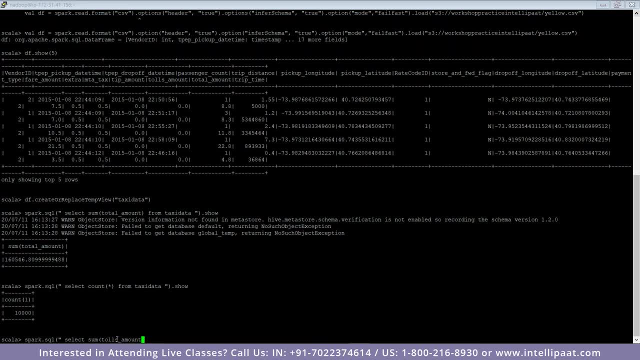 tolls underscore amount. so that would calculate all of the tolls and divided by the sum of the total amount, so that we have read the entire revenue once again, like we did in the previous section. and from taxi data. table name is important and then simply I can don't show, so this will do that for you as well. 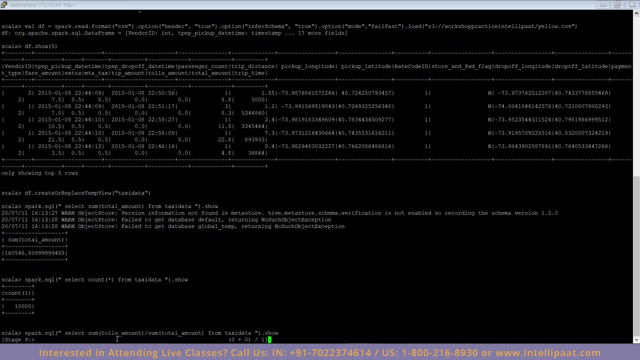 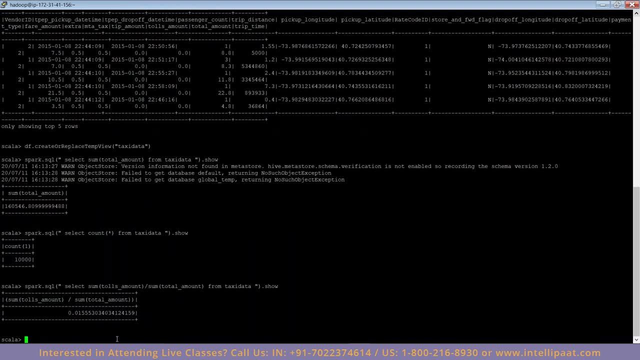 again, remember it will take the same amount of time even if you're processing large amounts of data. but the only caveat there is you need to actually increase the server size, the number of instances that are there again. so you need to increase that and to take the exact same amount. 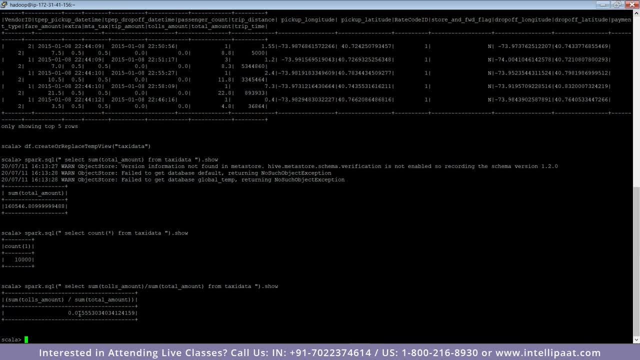 of time to calculate that. so, as you can see, here we have the total revenue that has been generated. so we can see it's about a 1.5 percent. so that is how much toll, that is, how much of the revenue has been spent on the toll. basically, so we get that. so say if you want to calculate the average. 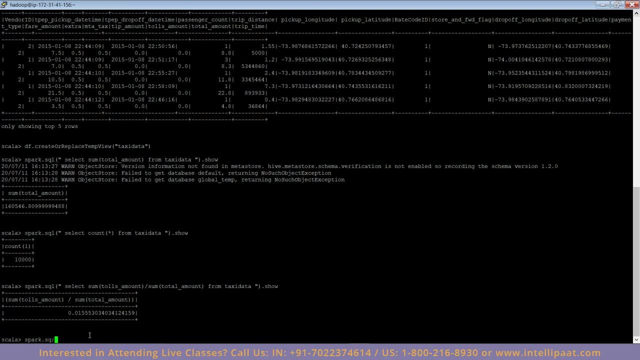 trip amount. so we can type in sparksql, select and like: SQL gives you these functions. SQL also gives you average function. but note this: we are not actually using mysql or anything. there is no sql system that has been set up on the system. my mysql has not been installed on this particular. 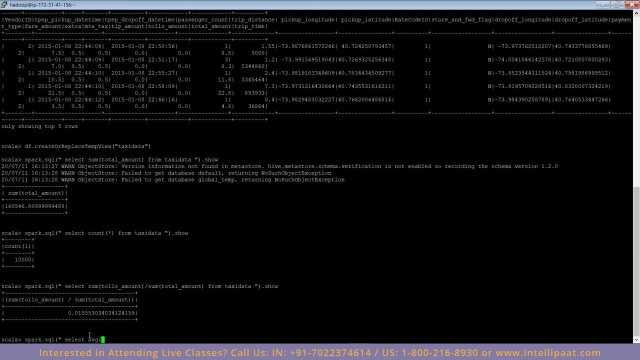 system that i'm using. nothing, nothing of that sort. spark has an inbuilt sql context, right? so it mimics sql, but it does not actually use sql any in any way, right? so that is what we're trying to do here. so sql is a language, right, so you can implement sql with mysql and other databases as. 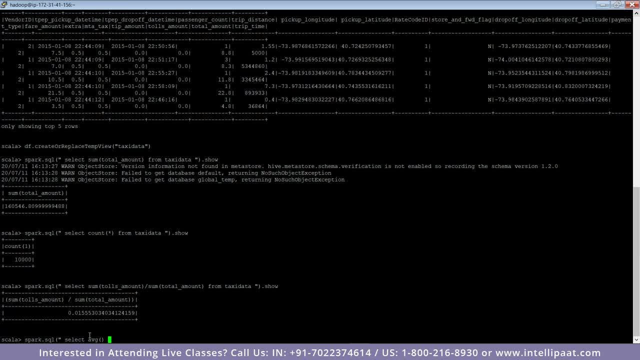 well, so it's basically a language and that language has been implemented in apache, apache spa. so average, and then we can give in like the total amount. so basically, you want to calculate the average revenue that is generated with every trip. so let us do that. so total amount. 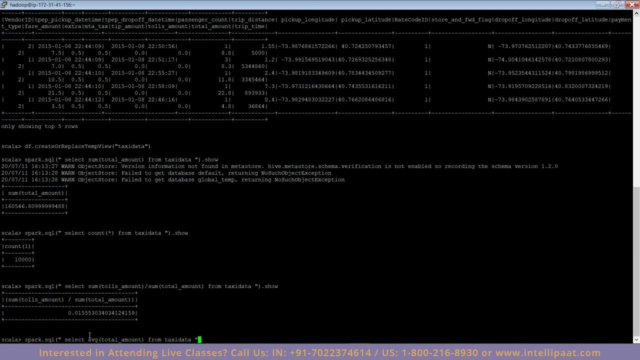 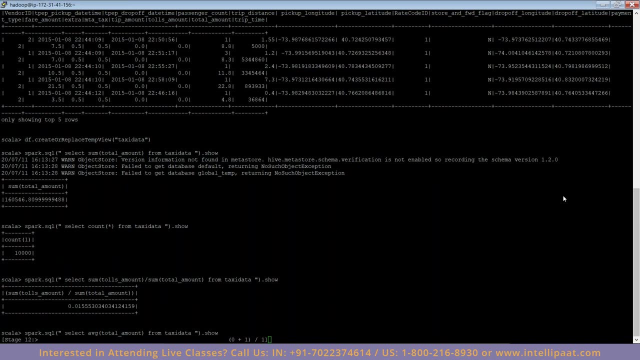 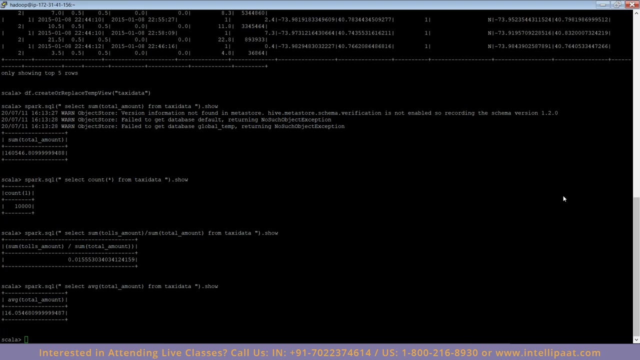 you and from taxi data dot short, it takes some time. let me look at some doubts that we have accumulated. okay, debug is asking: can we use health related or patient information data and, obviously, if you can use any data, state that data set that you would like. Fabian is asking is: 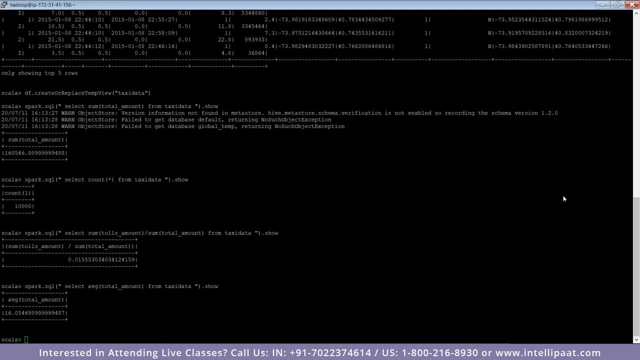 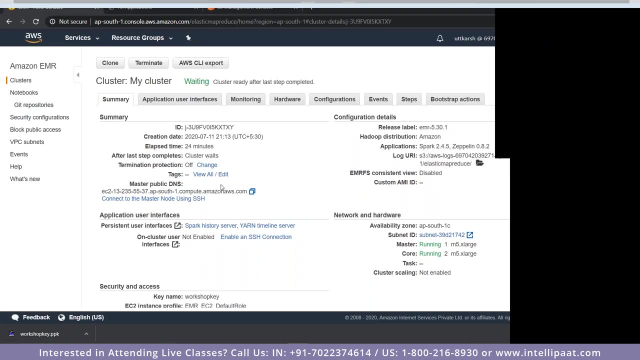 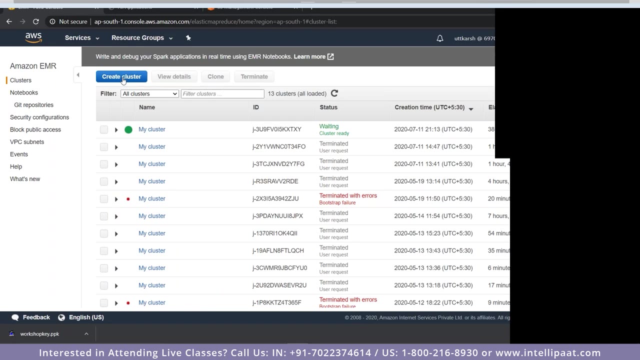 there, auto scaling and number of nodes based on my load. yeah, so there was an option, if you remember, if I simply try to create another cluster. so auto scaling. for those of you who don't understand, auto scaling basically means that Fabian, what Fabian wants to do is basically he wants to increase the number of instances. that is that. 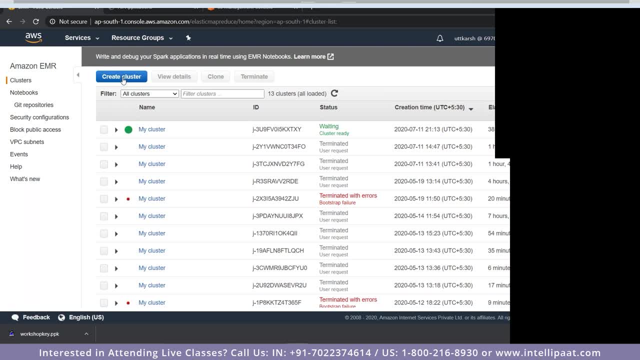 are being used automatically, rather than having us having to manually configure it. it wants AWS services to automatically detect. okay, this is a really heavy load that has been given to us as a job. we want to actually include more instances so that this job can happen in a much faster and more. 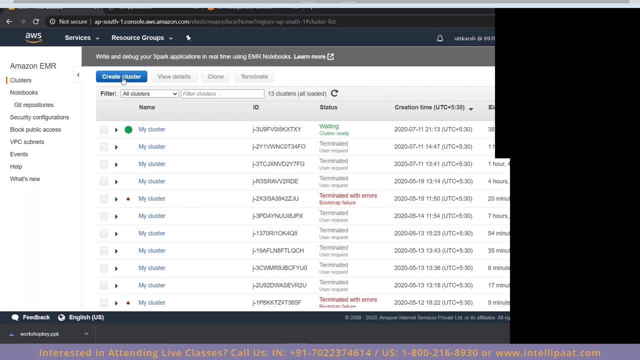 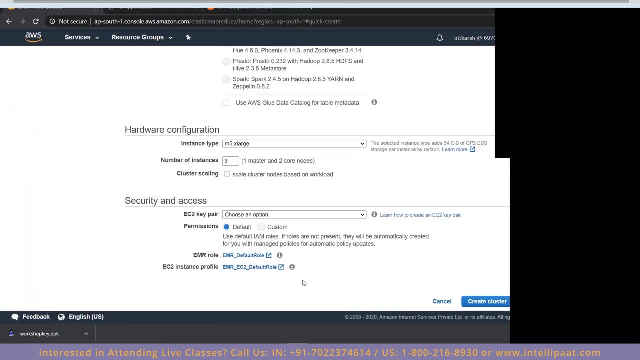 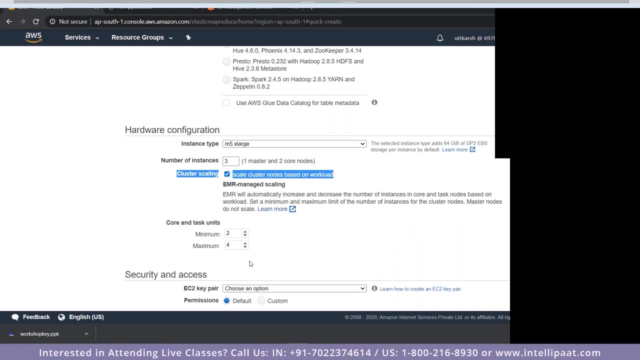 efficient way. so is there an option where aws automatically does that for you? so yes, there is. you create create on click cluster, create cluster, and here we can see there's an option: cluster scaling, right. so if you simply check this right and uh, what will happen is say that your cluster. 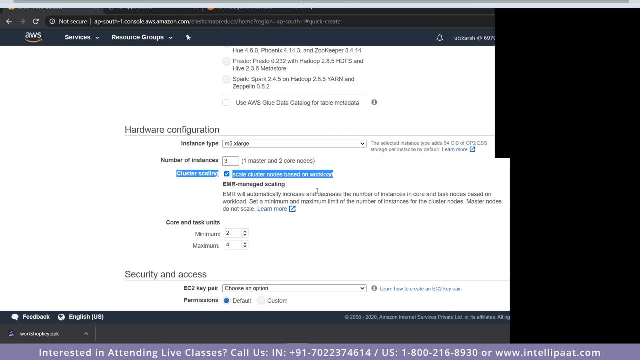 is basically uh accustomed to, basically uh configured or suited for processing only gigabytes of data, gigabytes of data- and you, suddenly you give that cluster a terabytes of data to process, right? so obviously that is not the uh appropriate setting. for that you need to need to have more instances. so if you simply take this option right and you actually 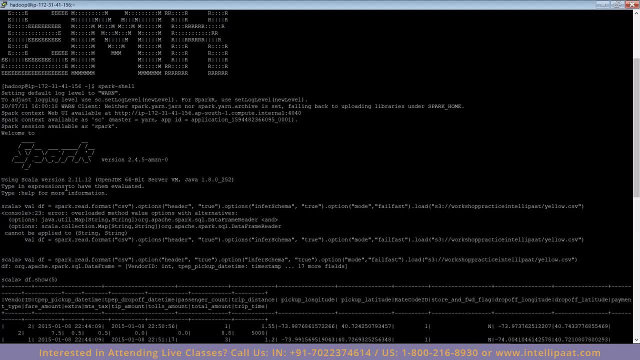 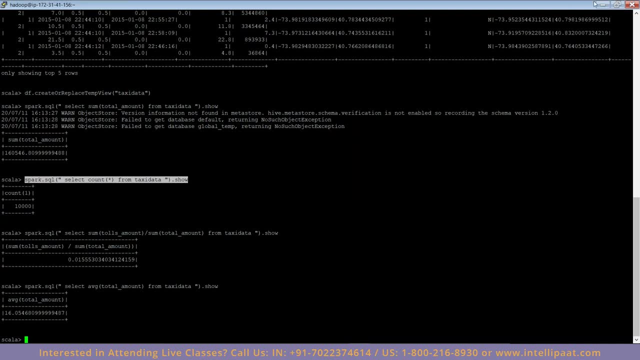 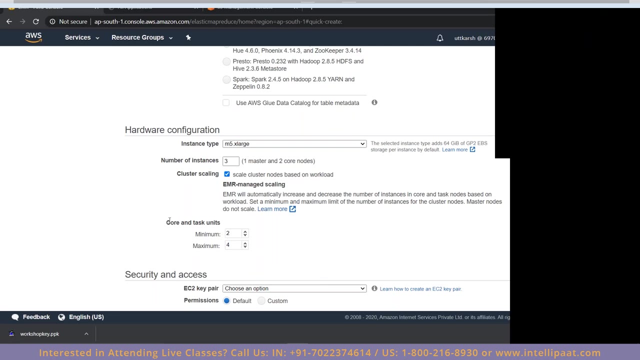 start to run that job, like i typed it over here, right? so what i did was like say, if i ran this job and it was on terabytes of data instead of gigabytes that the cluster is built for, right, so aws will automatically detect that and it will be based on these configurations. 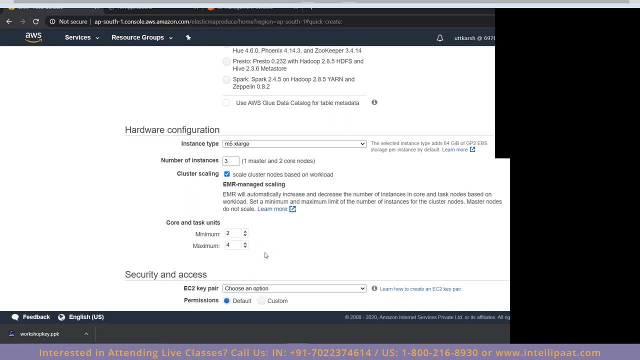 and, based on these configurations that you've provided over here, it will scale up your server so you can specify a minimum number of amount based on if your workload is really less. you can specify a minimum number of amounts. that is okay if the work is small. we don't want to have a really large cluster, so we can specify the minimum amount of. 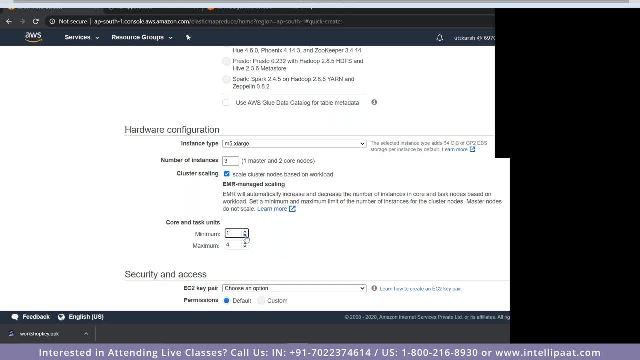 two, so you cannot go lower than two. uh, actually you can, but that will basically mean that, uh, your master's master node is basically your data node. it's always recommended that you keep it as two, so that there is always a data node attached to that master node, and the maximum number of 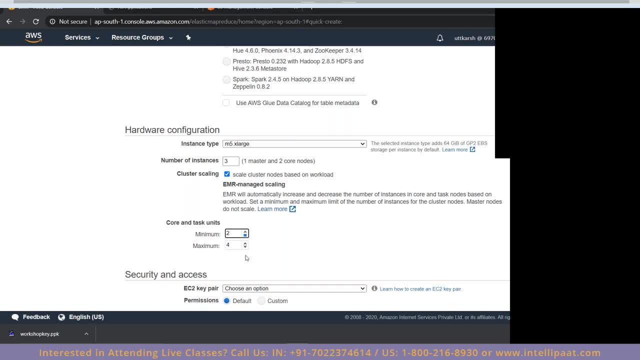 nodes that you would want to have in your particular cluster. so say, even if the job scales up really high, right, say it goes to terabytes, but even in that case you don't want a huge amount of bill, right, you don't want a huge amount of service bill, amazon service bill. so in that case you don't. 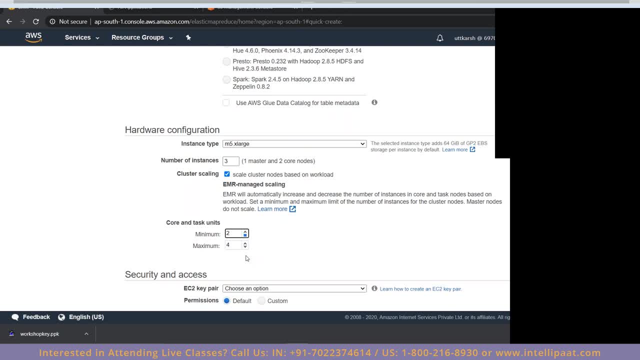 want to scale it up as much as it can. right, it could go up to a hundred, two hundred. you don't want that, say you don't, cannot afford that, that's why you don't want that. and you can specify the limit that you want on the maximum as well. so i hope that answers your doubt, fabian. let me just 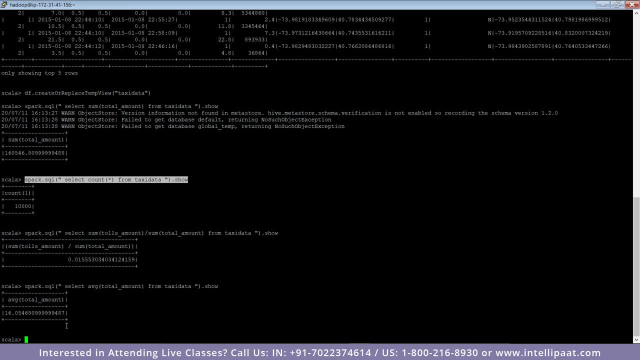 uh perform some other things and, on this as well, you want to calculate the average revenue for each of the payment types, right? so there are about four payment types, right? and we want to calculate the average revenue for online payments, for offline payments, for uh wallet payments, online. 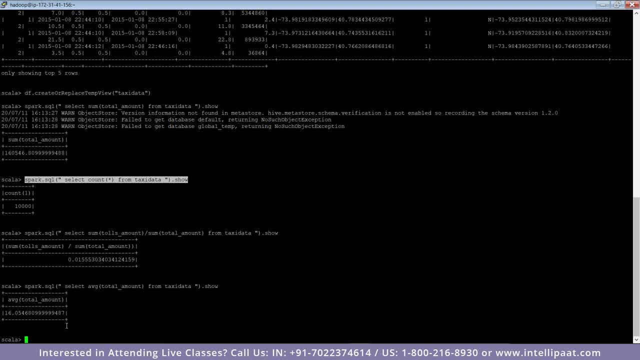 wallet payments or card payments. we want to calculate all that. so, whatever those four categories are, they are already one, two, three, four in this particular table. so whatever those are for, we want to calculate the average revenue that has been generated for with each of these payments. so we know which which customer, uh, how many customers? 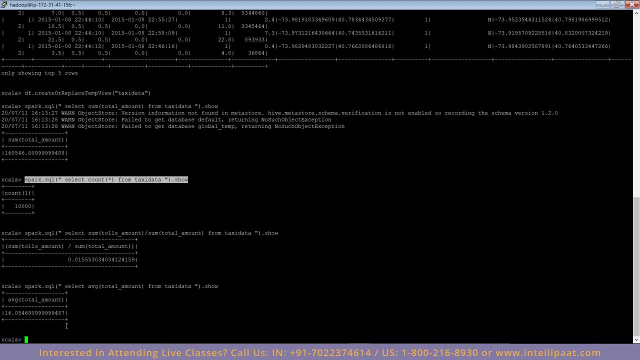 like what most right? so say, if it's, if there's a higher revenue for a particular, uh, payment type, we can know that that payment type is generally preferred more than most, right? so, um, for that we can simply group it by the payment type, right? so let me just see the column names. 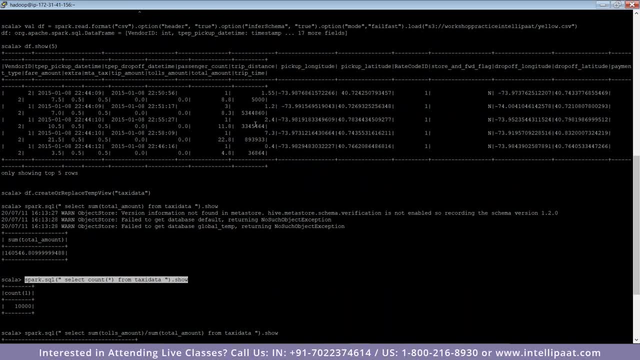 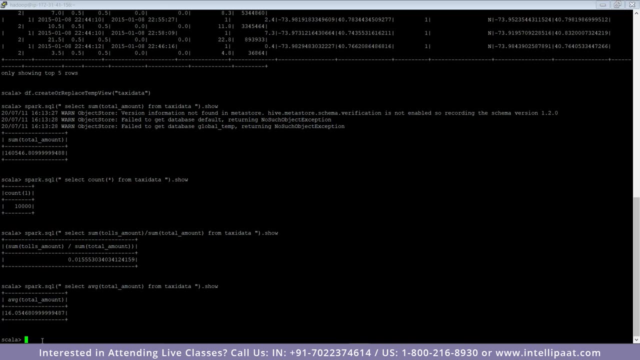 first. so what's the column name for the payment type? so that is the payment type column here. so it's basically payment underscore type and uh, okay. so let us begin with that spark dot sql and simply type in select payment type. so we want to actually include this. 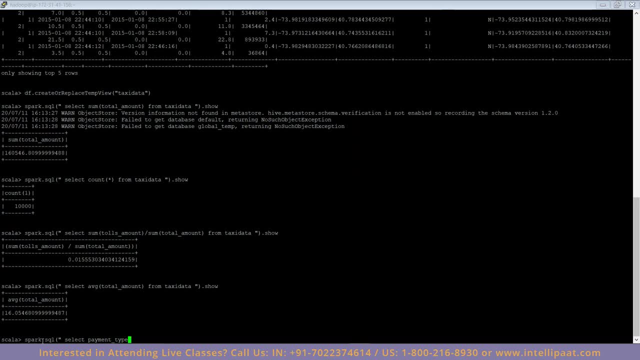 so that we can group it by that. so you need to actually include all of the column names. uh, you're going to be using in in the group by statement as well. so you need to include payment type. for that the average should say yeah, not the order. double quotes over there total amount. i want to include that as well. 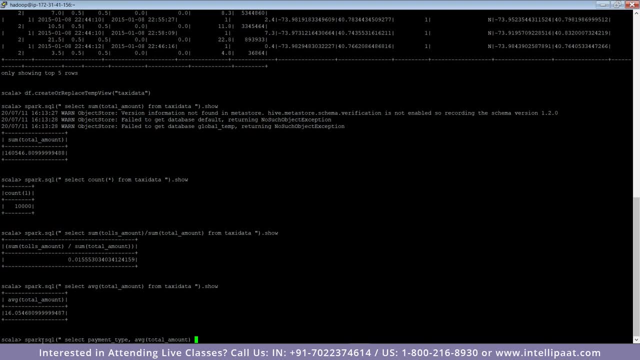 uh, and you want to include this as something. we want to change the column name for that. you can do that as well. so we want to display this as the average revenue and we're going to give the table name just taxi data and the service, and that's all. 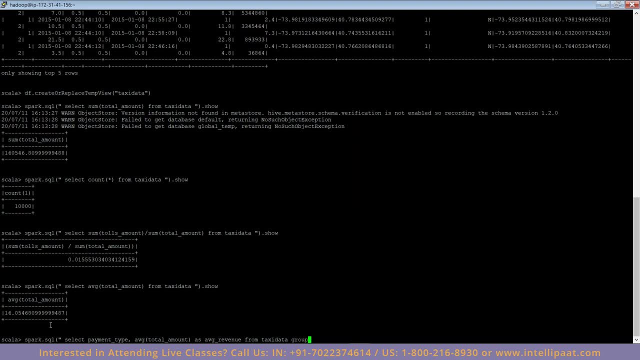 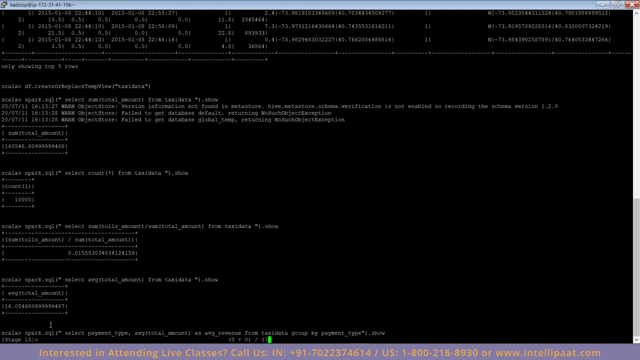 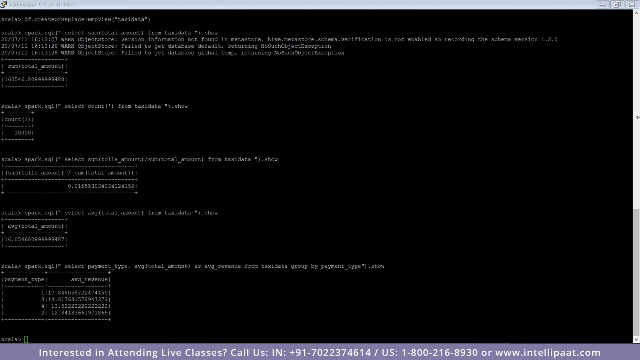 and that's how you're run data and want to prove it by the payment I and we simply type in box when we press enter. it will take some time and give us the output. now the asking: can we calculate the most profitable route from this data set? um, we look at the data, so 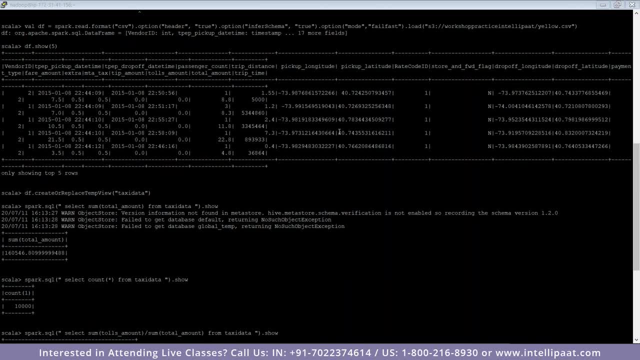 the thing about this is is it does not actually store the route information, right? I think it only stores the pickup location and the drop-off location, so any, because the route information then gets into very complex territory. it's geo positional data, right? so obviously Google, Google Maps records your or Apple. 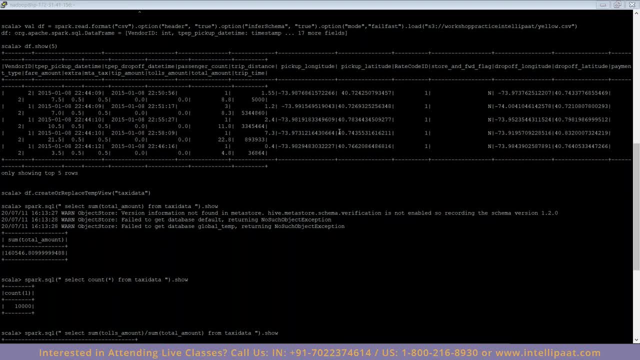 Maps records your route information, but I don't think the cab company this particular data set in. at least it's not recording the route information. it's at least not stored in the data in any way. but if it were there, definitely there is a way to do that, but it's not the column. 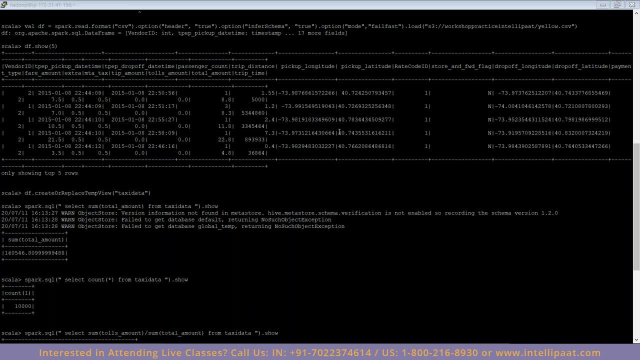 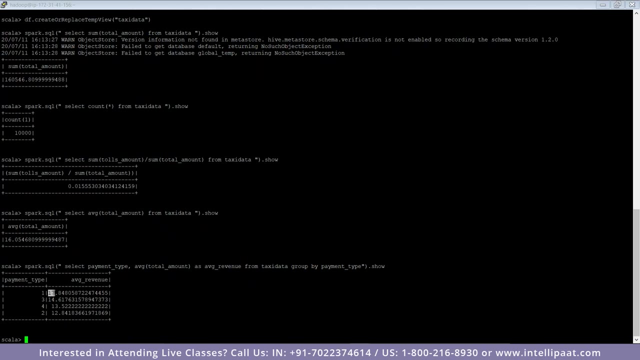 name is simply not there, the the data type. everything is not available in here, so I don't think we can calibrate the most profitable route and that for those of you who are waiting. so this is as we can see. for the first payment type, this would be offline. we are generating and cash payments were generating about $17. 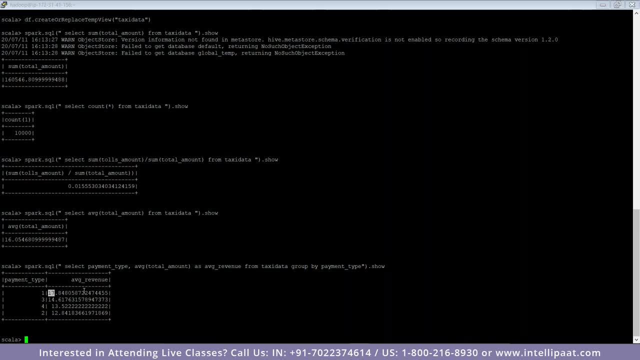 average on each trip if we're using the payment number three, which would be, let's just assume, online. so the online is accumulating about $14 average. four and two are accumulating thirteen and twelve dollars at an average. so we know the most profitable payment type is the first payment type or whatever the 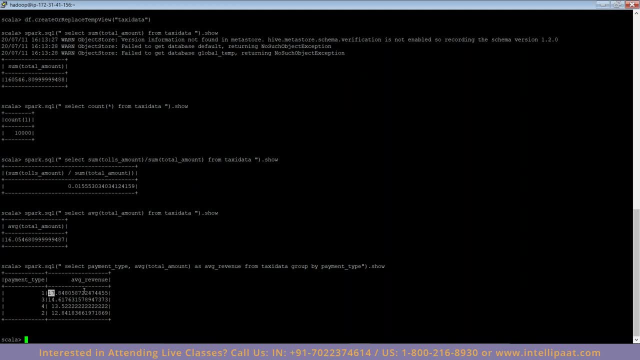 customers most used to prefer, use most to basically pay. so these are basically the problem statements that you would get as a big data analyst. calculate this so that I can implement that. so if you want to affect and impact company business policies, you basically give them these insights. yeah, so that we. 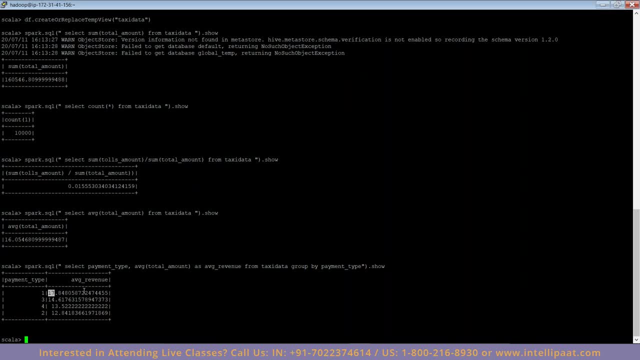 should encourage cash payments more. or, as we can see, we can try another question over here. if you want to calculate the most profitable are, so we say the employer of your comes in. you're a big data analyst. the employer asks you what is the most profitable? are in the 24-hour clock cycle that the cabs operate in? that our 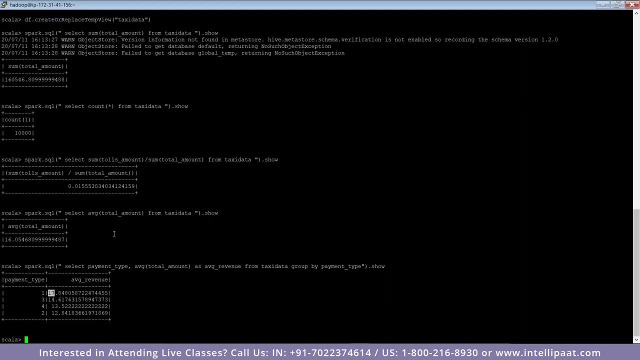 taxis operate. we want to know which are is the most profitable, in which are do we get? are the most revenue that we can right? so that is what the boss asks of you, obviously, to encourage the cab drivers more to be active around those hours. basically, give you that amount of data so we can do that as well. simply type in: 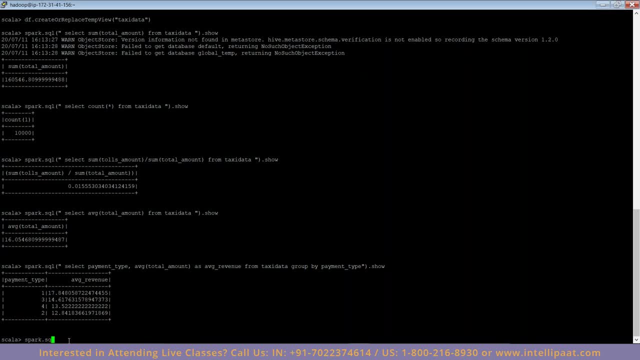 spark, and this is- this is not just in this small amount of 10,000 records of data. this could be in terabytes and terabytes of data. remember that. so it will give you the most accurate result possible, because the larger the data set, the more accurate the result is right. so we type in, select and we want. 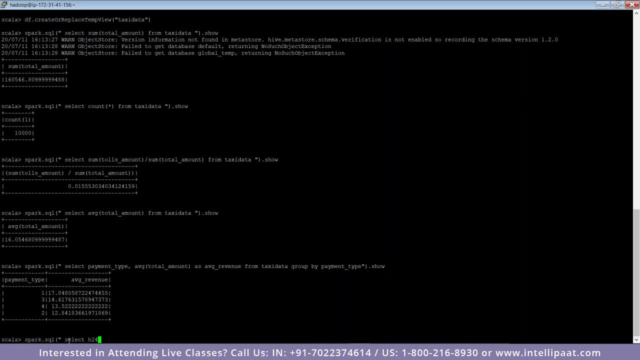 to actually name an alias for us. we call this a 24. since it's a 24-hour clock cycles will call it h24 and we'll display this as are. so we're going to be nesting an SQL statement and we want to get an average: the total amount to get. 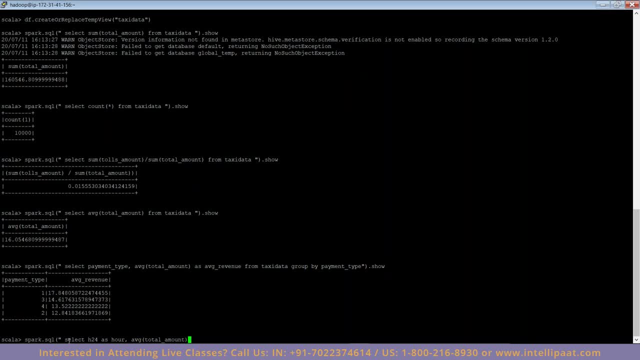 an average of that, or to get an average of that and we want to get an average of this. we want to actually see this as the aperture. let us just do that. you want to see this as the artist remaining, so that displays like that in the column name, like it did over here. we don't want. 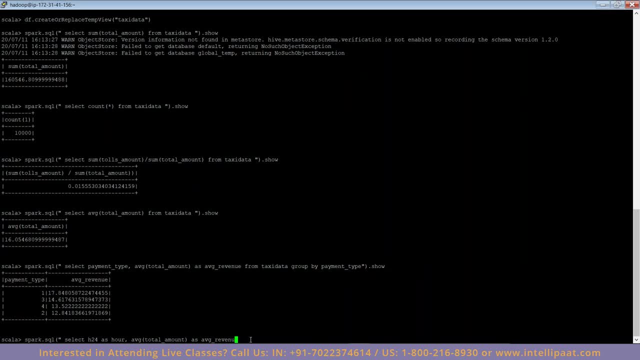 to see it as an average bracket open with a little amount or still have the stamina, and then we can give the select optionas role statement. so we'll do a Chinese check because I'll be sitting around repeating the same error if we click the Germany coming for us. but I think we'll see the average for the. 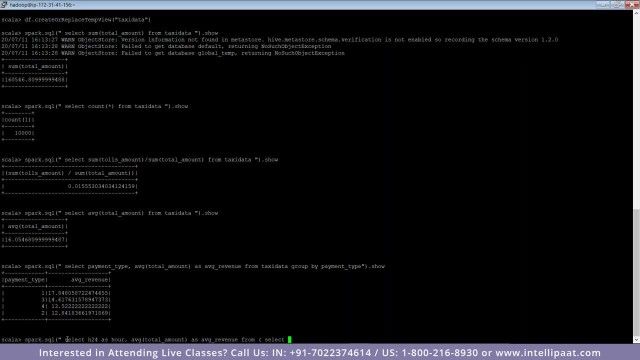 crust. we've hit over a 15so many times, 50 times, when the clock goes 20 said the government was doing. what can we do? we can into a few little mistakes in here, because if we we take pick this data that is being picked up right, right here, is being 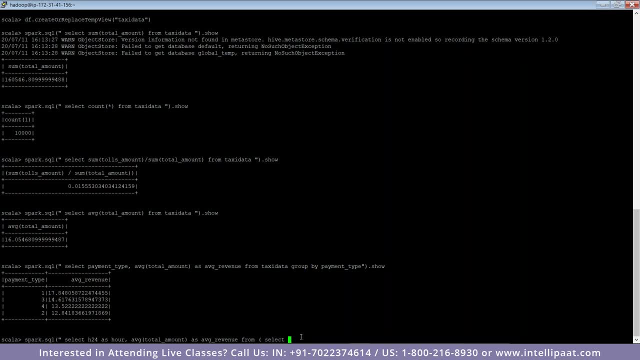 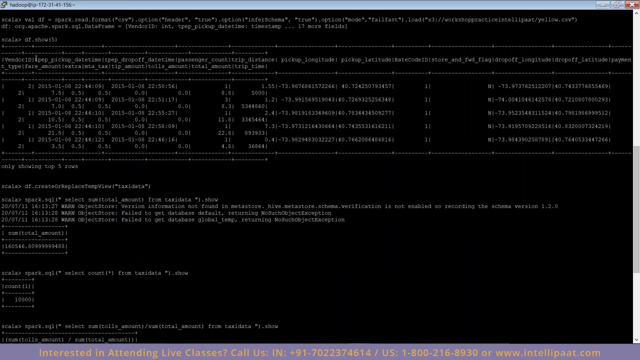 picked up from this nested SQL statement. so we can select R in this and then we can look at the pickup time. right, so we want to know the pickup time. we are not concerned with the drop-off time, we are only concerned with the pickup time. so let us look at the column name from the pickup time: just be pep underscore day. 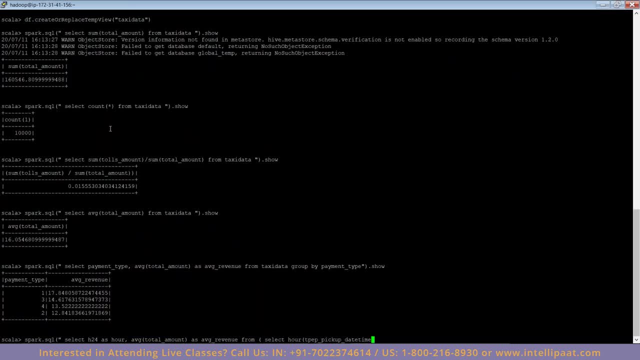 pick up underscore date time. we want this, so we basically copy that and paste it over here. so one thing happened. thing that happens with these terminals is that whenever you select a particular amount of string in this and you right-click on it, automatically pastes it wherever your cursor is. so that is. 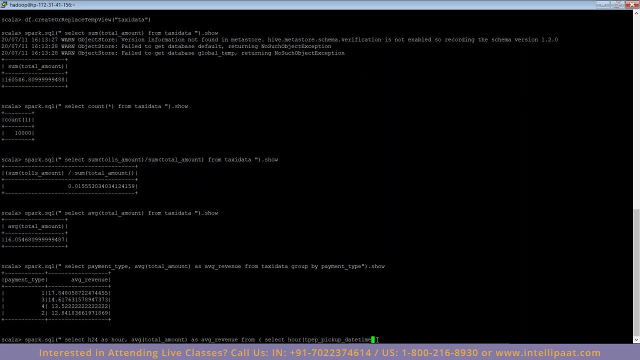 why it's instantly transferred from there. and then we want to give the R, as let's say, 24, so that is what we are referring to outside the nested statement. and then also, we want to get the total time as well, and this total time not total. 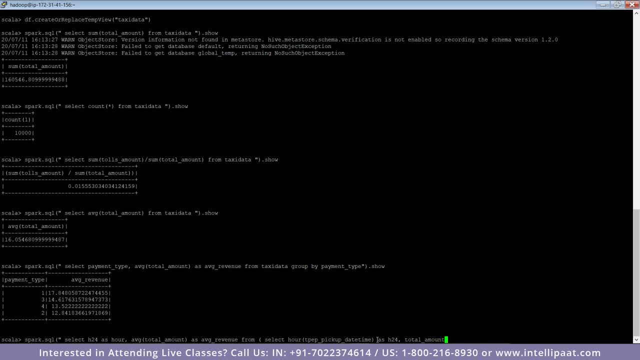 amount. you want to get that and you want to get the table name again. so this is the very important, because in the SQL nested statement you need to get the table name and simply close this up now and we want to group this by the R, right, we want to group this by the time of pick up, so we know this R is the most. 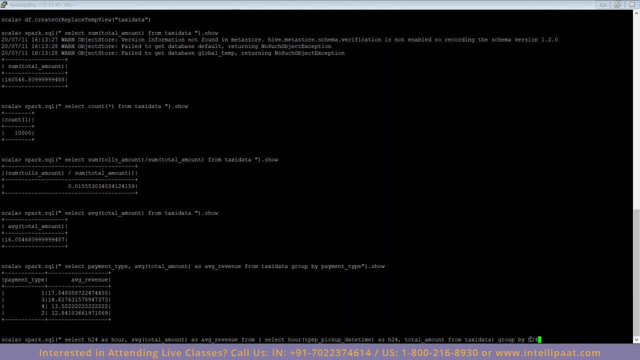 wrong. so you want a group this by age 24. total amount: you, not truth alone, actually. okay, so we had a grouping this piedage 24. now what he wanted: we want the highest revenue generated to display first, right, so we're also going to be ordering this. we're going to be sorting this. 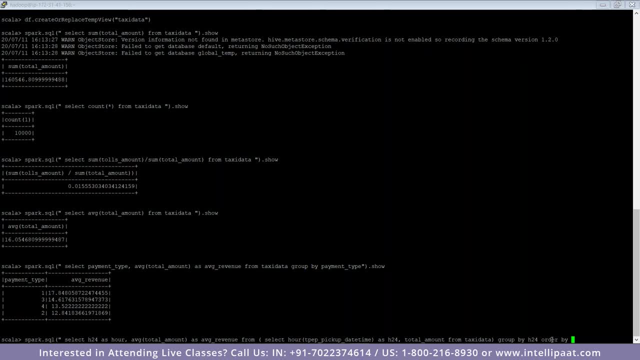 particular output that we're getting. by what? by the average total amount, which is the average underscore revenue. you want to actually sort it by that particular column value. so that's what we're doing and, uh, since we're not going to be assembling this in the ascending order, what we're 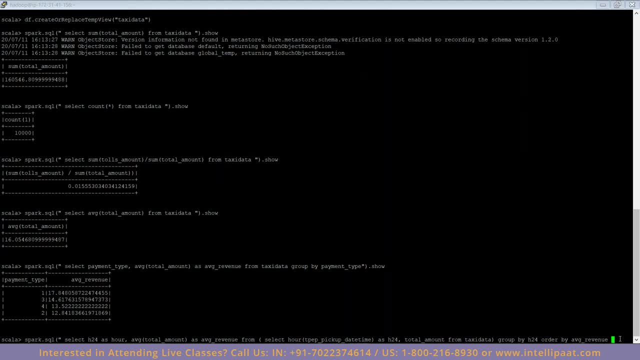 going to do is actually arrange this in descending order. so if you don't specify the desc over here, i'm simply going to write the writing dsh over there. if you don't write that, it will automatically arrange the data in ascending order and order it with the revenue from lowest to highest. what we 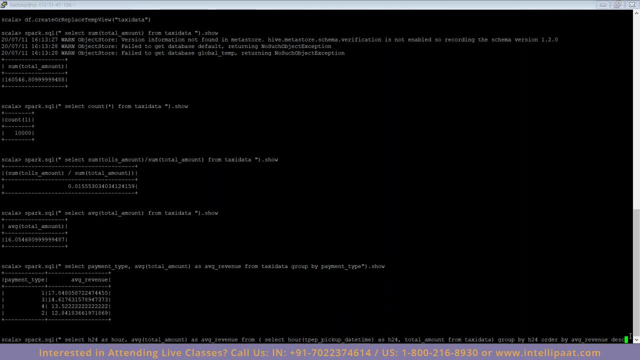 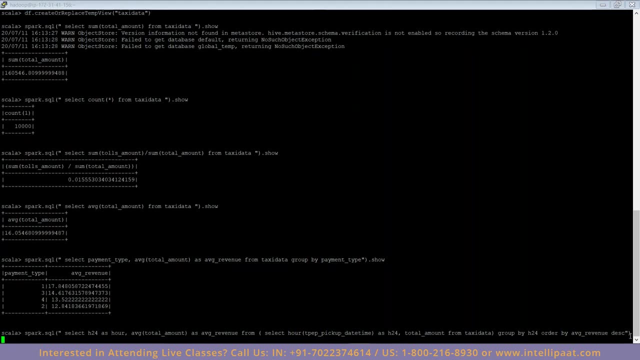 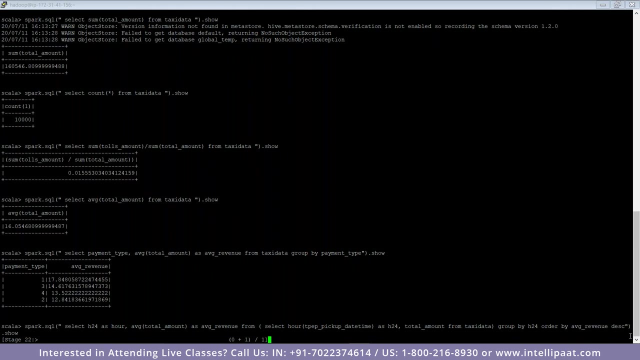 want to do is actually arrange it in the descending order. that's why i've done that the highest comes first and then. once we've done that and simply type in dot show and press end. so it will take some time but it will give you the most profitable r on the top. i think this data 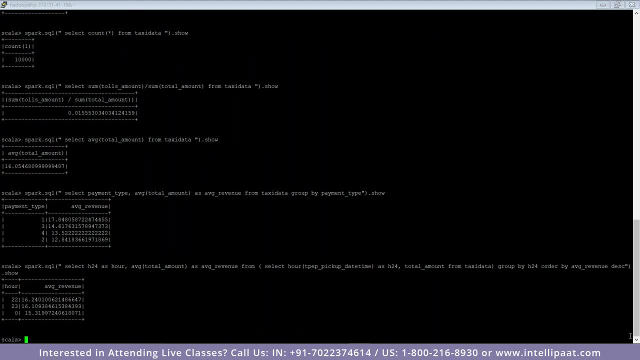 only contains data from four hours or three hours. yeah, so three hours worth of data. so the reason we're not seeing all of the uh from- i think there are 24 hours in our day, right, so we're not seeing it from uh zero one, two, three, four to twenty three. the reason we're not seeing that is because this: 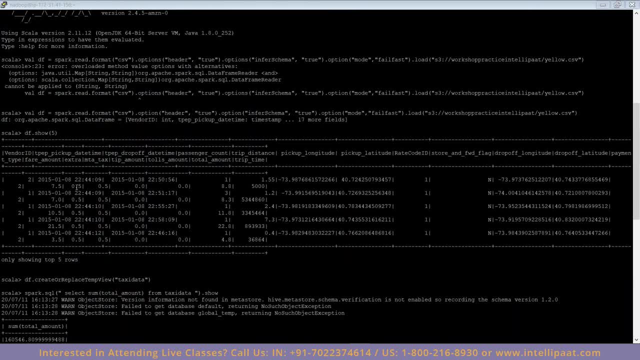 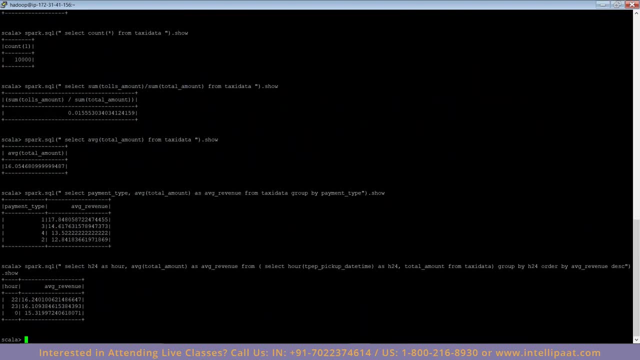 data is only ten thousand records and i think it's only been accumulated, uh, from the night time amount of data. so if it had all of the hours time included in this, we would have gotten all of the hours and the corresponding app is revenue to that. but we're not getting that, but for this case only. 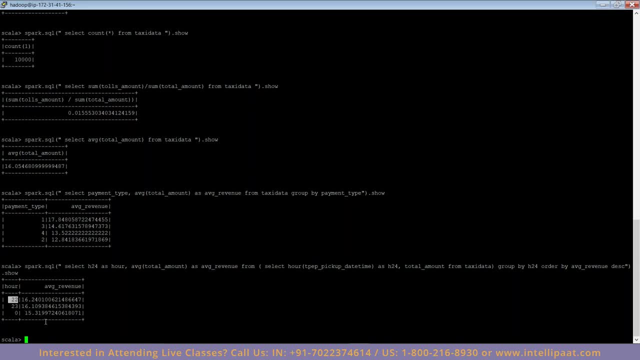 we'll see this- that in r22, which is uh 10 pm, that is, that accounts for the highest average revenue. so now the company knows when to push the most ads, when to push the most offers, when to push the most gap drivers on the job. right now it knows that this is the most. 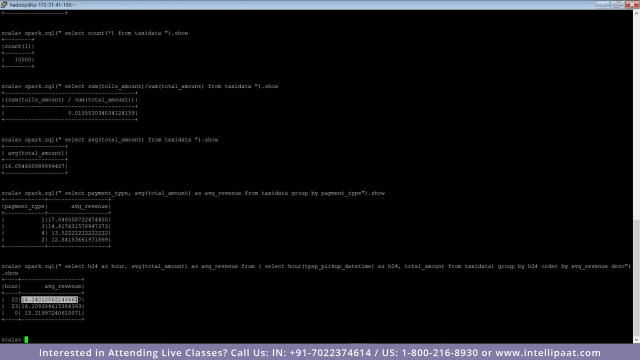 profitable r in our business and we want to push the absolute maximum business that we can in this r the 10 pm r. so you can see how naturally big data analytics affected uh company growths and profits. right, that is how technology assisted that company in determining which r is the most profitable and 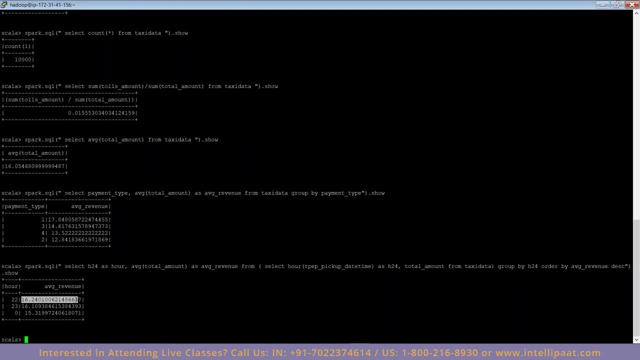 now the gap drivers will be focused on. that r only right. and naturally we can also see the other hours as well. so can see 11 pm, which is 23 hour mark. you can see it's a little bit lower than the average revenue at the 10 pm mark, so we know that 11 pm is also really. 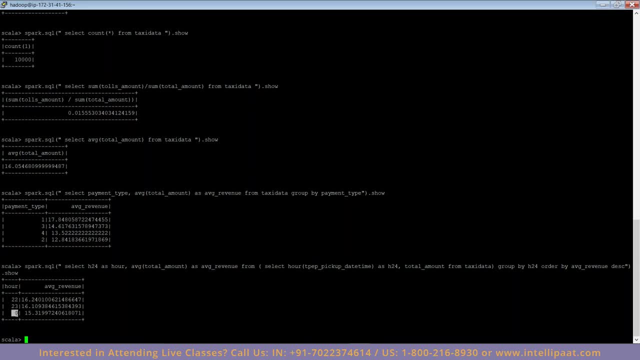 profitable. we know that 12 am, which is 0 hour, 12 am is 0, we see $15. we can see that it's gradually decreasing as well, because as the night progresses, less people try to travel in that time, so it will naturally get to a lower point. so 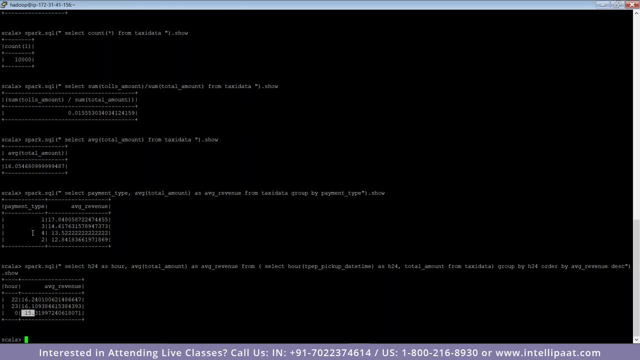 say, if it had all of the 24 hours available in the data set, say, the 4 pm mark might have been the highest to the 6 pm mark, when most of the people are returning from office- not right now due to the corona virus, but if it's a. 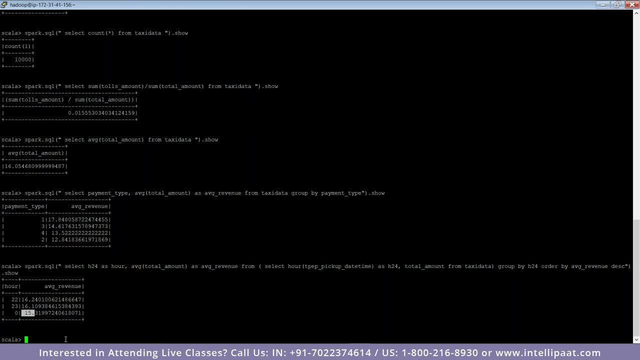 functioning time in our economy and everything. so they are returning at 6 to 7 pm, so you would have seen a very high hike in the average revenue during those hours. that is the advantage of big data analytics. let me see some doubts, Surendra, asking: how do we create insights like graph so spark does come? 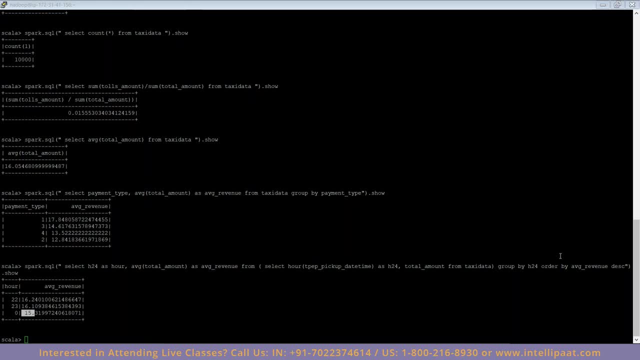 does comes with a data visualisation tool when it's called graph X, so you need to look more into that and you can basically perform some data visualizations on it. but the way I like to go about data visualizing using big data is by using pie spar, so let me just explain to you what my spark is. so right. 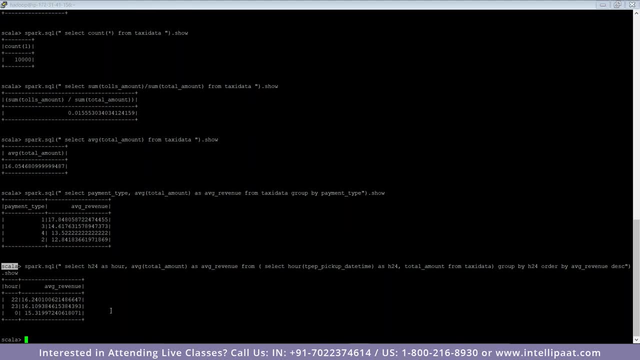 now I'm using a scholarship午餐 language, right. so what i'm doing right now with Scala is something that can be done with java, python and r as well, because uh, spark comes with apis and packages, uh, libraries for Scala, but spark also comes with libraries for java, python and r programming. so if you're coming from a data, 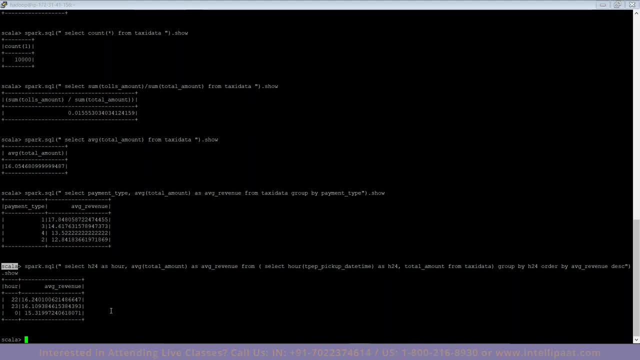 science background, right? so, uh, you naturally are accustomed with either r or r or python, because those are the most popular languages in data science, or, if you're simply coming from a normal data analytics background- not from big data analytics background, but a normal data analytics background- you know those two languages. either of those two, because it's basically your job to know. 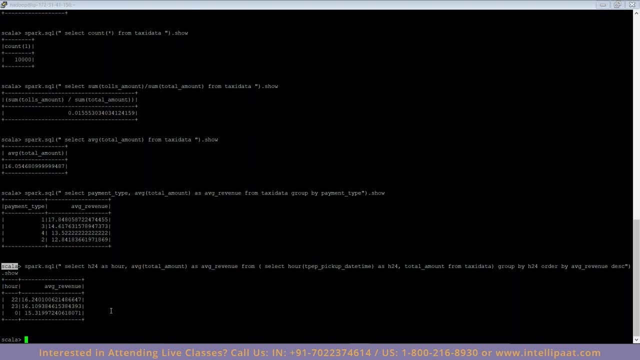 them and you come into, uh, big data analytics and there would be a lot of resource wastage if you are taught an entirely new language. right, you don't want that. that is very inexpensive, especially people who are coming from non-technical backgrounds, who have not coded developmentally if they're coming from a business. 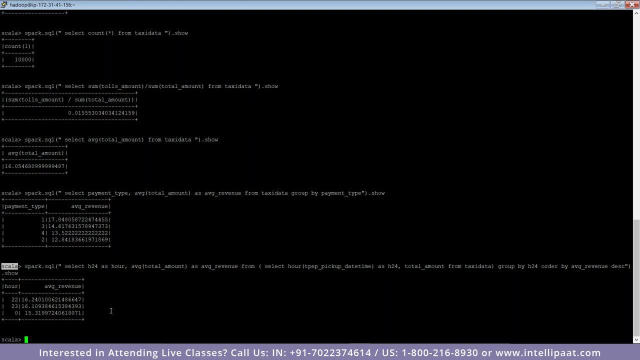 intelligence background, or simply a statistician's background. right, you want a tool that requires you to learn the most minimal amount of information you can and basically implement the previous knowledge that you had into your code. right? so that is what is there. so, right now. one of the examples that we displayed was: 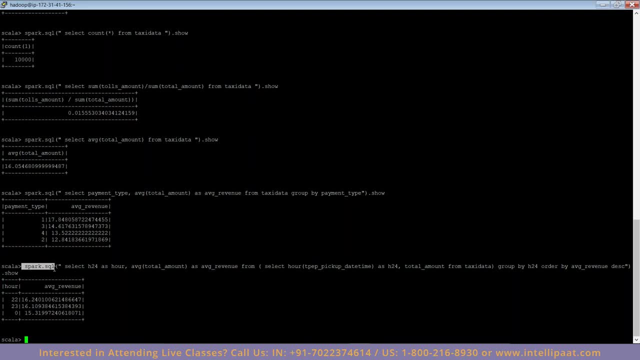 using sql statements. the only new thing that you had to really write was sparksql, right, and the rest of it was already, uh, what you would normally write in sql. you didn't need to learn anything new. so if you're coming from a database background, from a mysql background, you already know all of this. 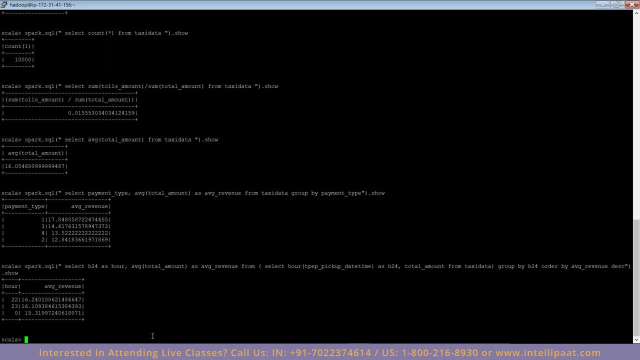 so you're not really doing anything new, but you do have the advantage of using uh, a tool which helps you process. instead of processing megabytes of data, you're not cross terabytes of data without actually having to learn anything new. so that is the magic of big data analytics with uh. 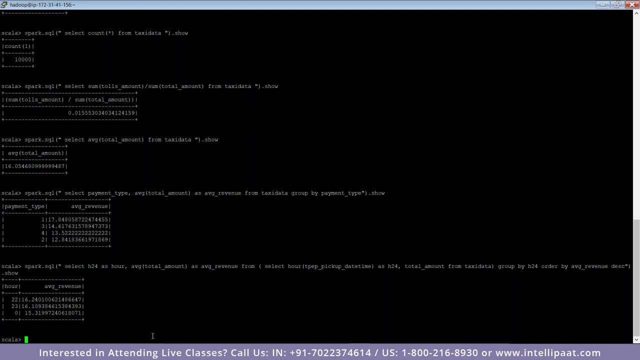 ardu and spark and all of these tools. so with python, there are libraries for it. with python also comes a machine learning library and a- yes, uh, uh. what do we call it? machine learning library? and just a moment, what was the? yeah, machine learning library? and data visualization tools like pandas and 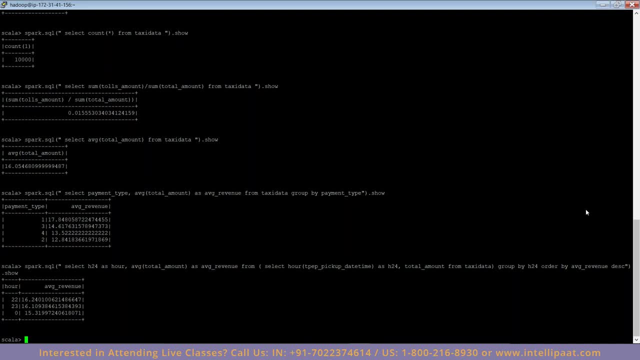 uh, matplotlib. so you have all of this right. you can simply integrate the both of them simply by using the spark library. you can integrate python and spark and perform all of the tasks that you want, and as long as you're using the spark libraries within python, it will take advantage. 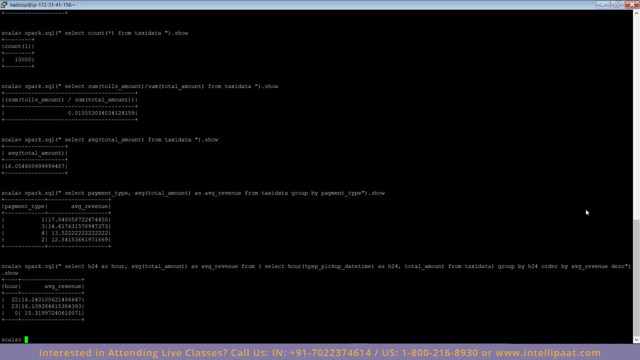 of the infrastructure that you have- your cluster computing infrastructure that you have, the big data cluster that you have. it will take the advantage for that and you will code in the exact way as you were coding before, with normal amounts of data with small amounts of data. so that is called by spark uh. it's one of the other uh friends for big data. instead of using 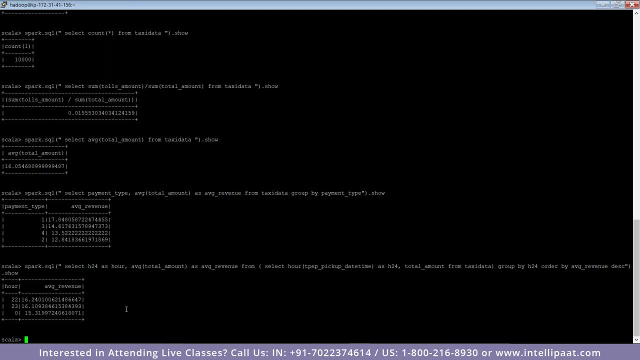 scala and spark. you can use python and spark as well, so that is, by simply importing the libraries for that. yeah, so i think that answers that out. as a big data analyst, are you responsible for selecting and shopping an online data set? so, uh, in most cases, uh, the job role of 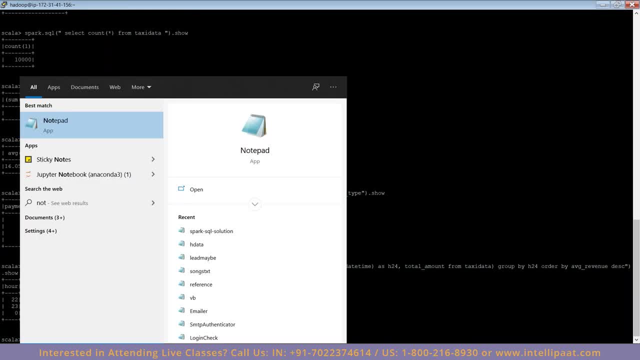 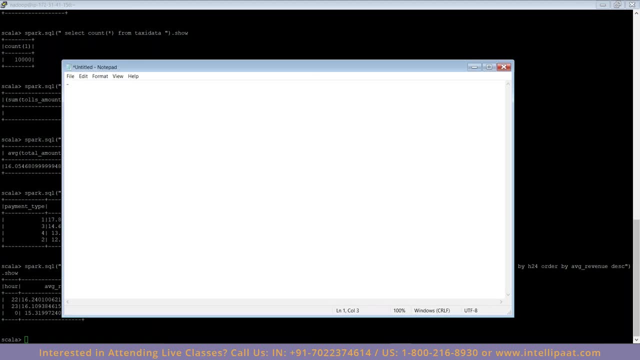 a big data analyst is just a moment. i'll just show you, guys, uh, 90, 90 of the cases, what the role of a big data analyst would be is, uh, extracting useful information out of unstructured data. this is the task of a big data analyst. the first task, then, uh second task, is converting this information. 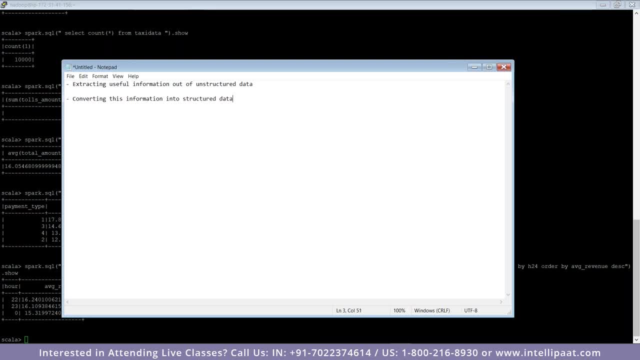 into structured data. and third task, which is the final task, where the actual innovation comes in, is uh actually uh, querying or solving business problems. business could be business. if you're working in the working uh for a government environmental agency, you might be analyzing some geographical data or environmental data. so, business, not. 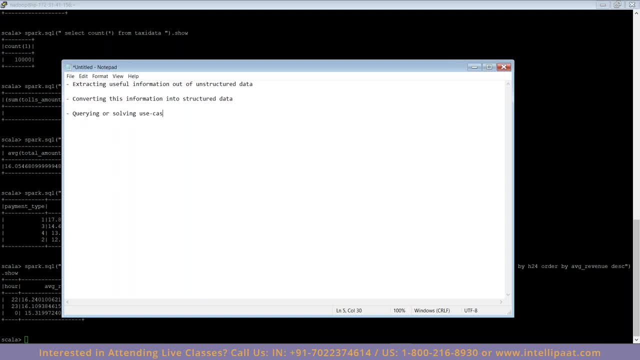 necessarily business any use case, basically solving use cases for your organization. so, uh, the thing about the difference between data analytics and data science: right in data analytics, you already know what you have to do. your boss has already told you, you have been instructions have been given that you need to. 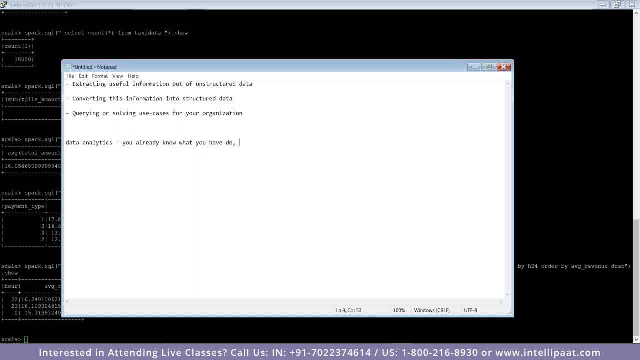 tell me this, right, you need to tell me which r is the most profitable. you need to tell me, uh, which? which route is the most profitable? not profitable, business route is the most used? which route has the most traffic? you need to tell me all of this. so the question that is being asked of you. 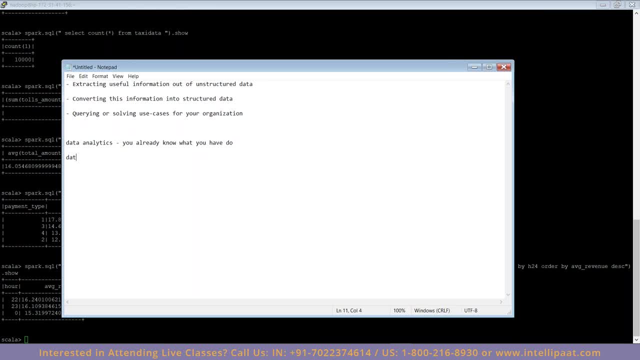 is already known by you, right, uh? so um know how you suddenly knowing the difference in what's more profitable than either the thought or theml if you have a comparison with some from some one single company or company, uh, or the, the, who is the most profitable? 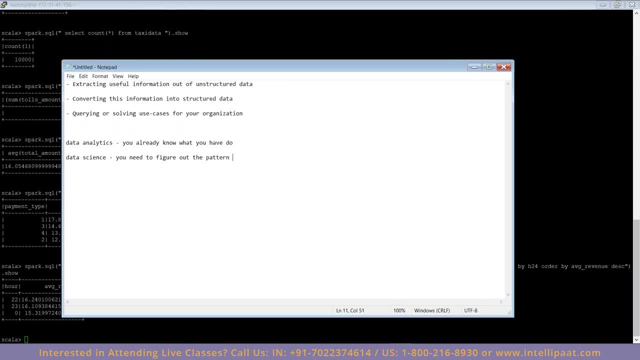 and fühlt. ¿no know the difference in those two countries, but in data science that is where the difference comes. you need to figure out the pattern. so the question is not known in data science, so you don't need know what you actually have to find. 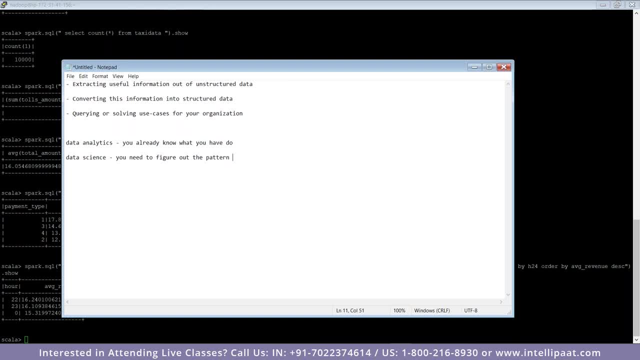 data scientist and the job of a data analyst is basically solving whatever problem statements the company is giving them. so the thing is, these two professions work really well simultaneously, right? because if you're this, changes to big data analytics, right? so, naturally, the first thing that you have to do in order to become a data scientist, first become a data analyst. 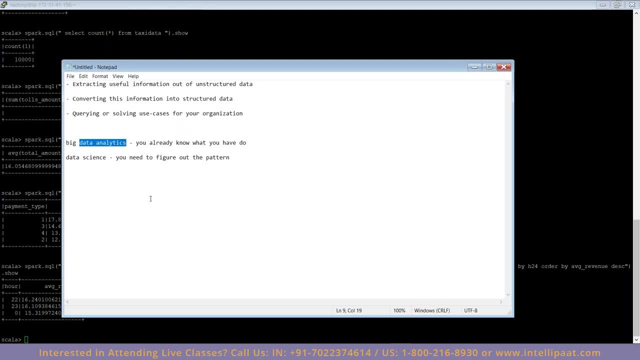 right then only if you understand how to work with data, then only you can get to the scientific part inside and only you can start with data science. and naturally the other front in that is machine learning and then the other front of that is artificial intelligence. so this is the absolute maximum you can. 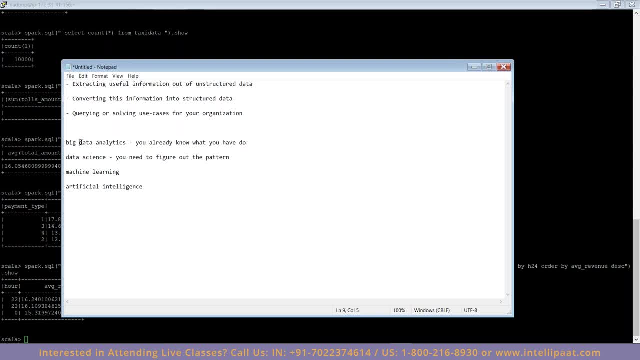 go with this particular field. it starts with the data analytics, goes to data science, goes to machine learning, if you want to expand on that, and goes to artificial intelligence, if you want to expand on that, right. so that is there. so the advantage that comes in if you already start with big data. 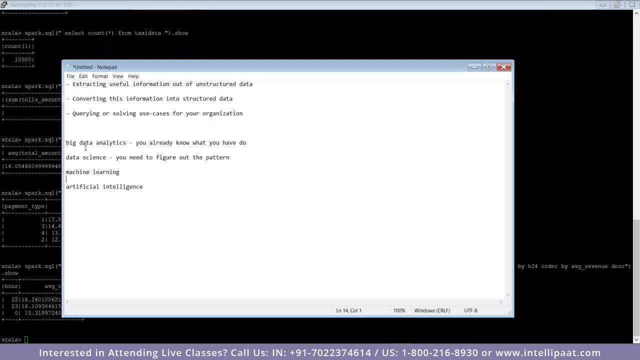 analytics right if you already start with that. if you start with that as the first step, then when you transition into data science, you basically have an upper advantage because you know how to perform data analytics right, but you also know how to perform data analytics with a huge data sets right. so, say, if you have terabytes- 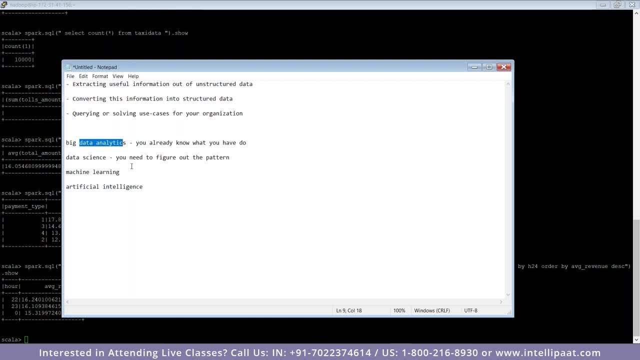 petabytes of data sets and you want to extract some models out of it. simply plug it into Python's. plug the spark libraries into Python, use PySpark and calculate the use case statutes. you use a Java manually or even, if you want to create a model, machine learning. 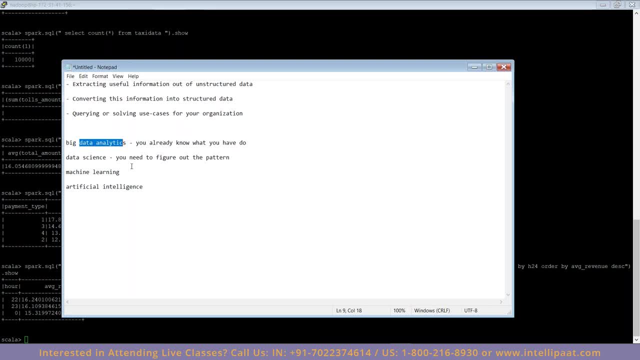 model. simply implement all of the things that you used in your normal data analytics knowledge with Python and create a model out of that spend with artificial intelligence. so this is the way, which actually is video. this is why big data analytics is a really good topic to basically understand. okay, the 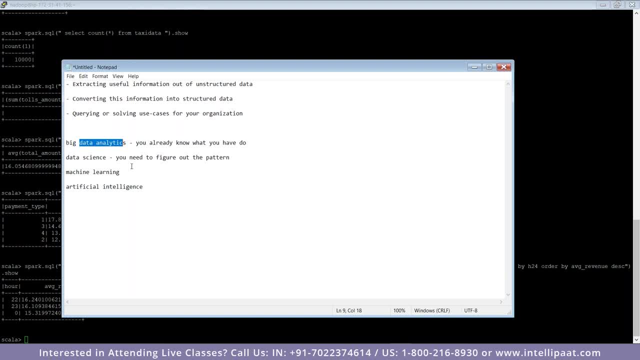 question was it selecting you are not actually responsible for? actually, you're not shopping for a data set as a big data analyst unless you're not actually have to pay for the data set that you're buying. If you're working for an organization, if you're an independent data analyst, right? 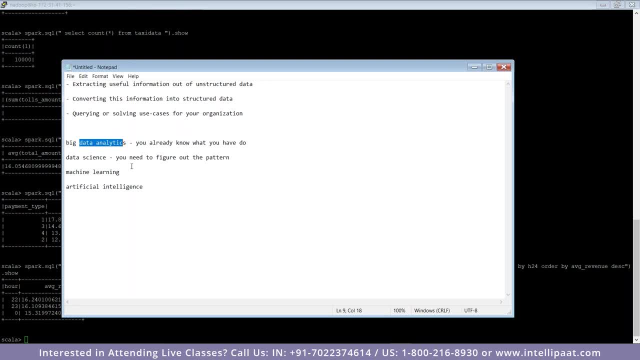 then definitely you might be shopping for a data set. But if you're working for an organization, they'll definitely provide you with a data set and they'll tell you what to do with it. Or, in most cases, if you're working as a data analyst for a particular commercial company. 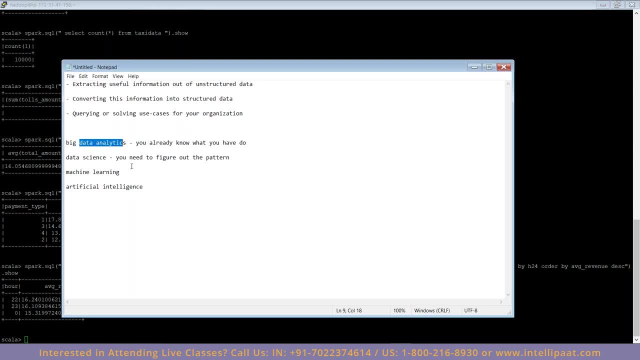 the company already has its data. you don't need to shop for it. they'll give you that for free so that you can actually do your job. Juan is asking what pays more obviously, if big data analytics, if it's data analytics. 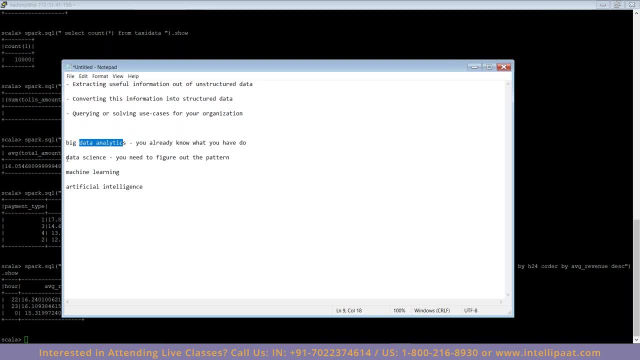 versus data science. if it's simple, data analytics versus data science, right. the pay scale is quite skewed. The data analyst earns a lot less than a data scientist, definitely because a data scientist has to use a lot of brain power more than the data analyst, right? 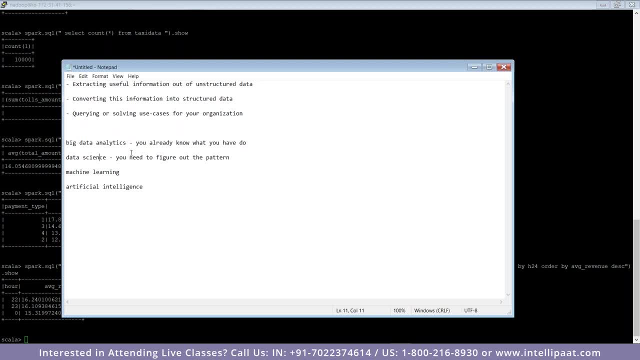 But if you're a big data analytics you'll lose a lot of money. But if you're a simple person, you definitely get paid a lot more- almost at an equivalent scale- to a data scientist, depending on the seniority that you have. 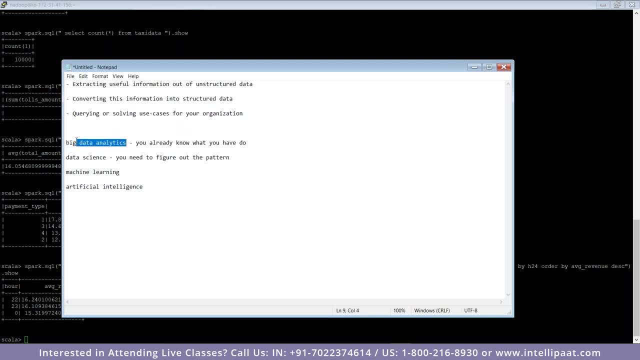 So that is one of the reasons. if you are basically a big data analyst, you can get paid, if not much in the same range as a data scientist. you simply get paid in that right. But definitely why not expand your career after that? there's no harm in learning data. science. why only stop at data analytics, right? And then simply, if you're a machine learning expert, definitely you get paid a lot more, because we need a lot of those today in our industry, and artificial intelligence is obviously the future. 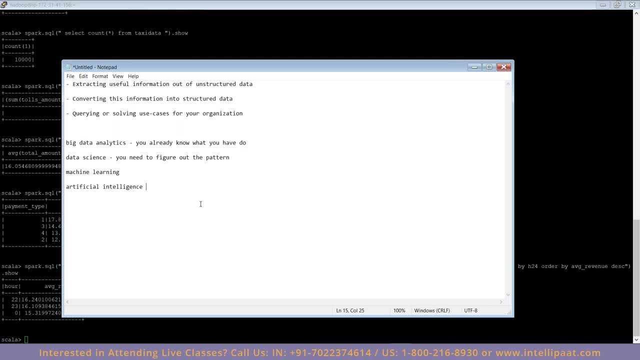 So everything in that regard: you get paid. as you learn more skills, you get paid more. In order to understand data science, you need to have a really strong mathematical base, right? you need to be good with statistics. basically, you need to be able to do that. 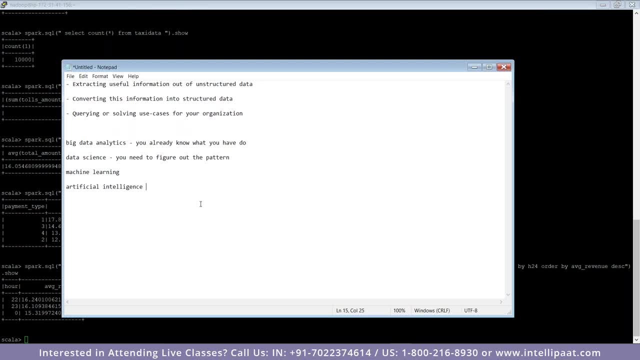 because a data scientist implements a lot of statistical information and data science and is basically in his job profession. So you need to be really strong with how you calculate your stats for data for in order to be a data scientist. So, alright, guys, I think we're about at the end of our session here today.